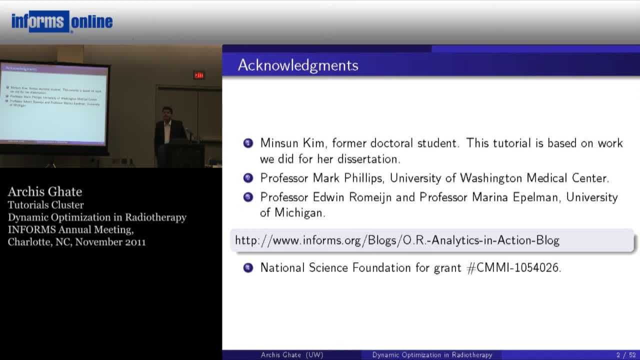 actually came to give a talk in my department in Seattle and I went to that talk and Mark Phillips was in the audience there And then the three of us had coffee basically, And that's how I kind of started thinking about this area of radiotherapy. So if we had not 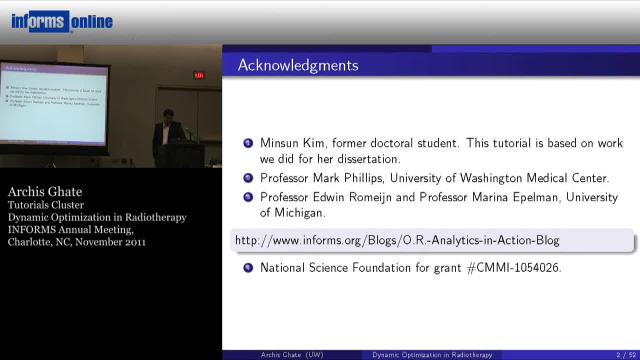 had that coffee, this would not have happened. So that's a big thank you to Edwin, And then to Marina Eppelman, who is actually here. She is a very true friend of mine And she has been a friend of mine for a long time And I think she has been a good friend of mine. 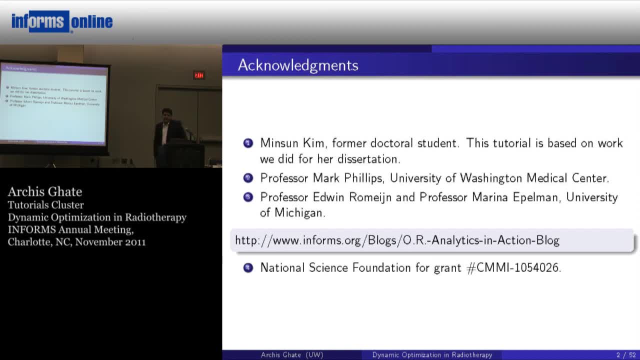 here. so one time actually, I gave a talk, a short talk based on some of this work, and at the end of the talk- I don't know if she remembers, but she winked at me and she said: this is neat. so because I was at that time completely new to this, 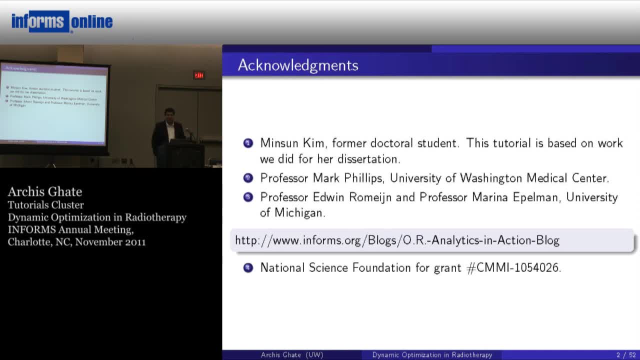 area. so I was not sure you know what I was doing. and then I went back home and I was talking to Minson and actually some of the ideas Minson said this is junk, basically we should not do this. and then I said Marina said it was neat, so 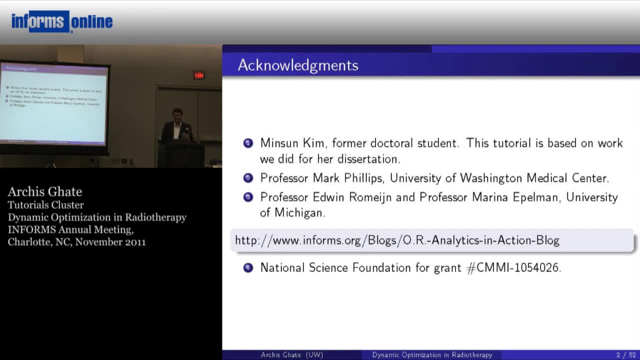 we're going to work on this, at least for a little while, and then see where it takes us, and then this is how this research kind of started. so that's why I'm indebted to Marina also. so thanks for that. so, in fact, recently Infonce invited me to blog about this topic on my work in 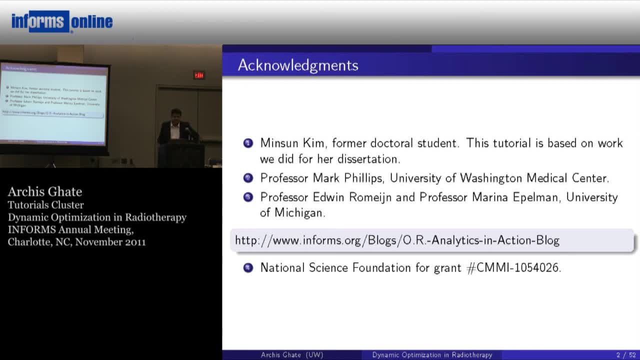 this topic on a blog that they have started recently. so if you want to read a story about you know these kinds of things that I just mentioned, you can go to that blog and find this topic there also. you can go to that blog and find this topic there also. 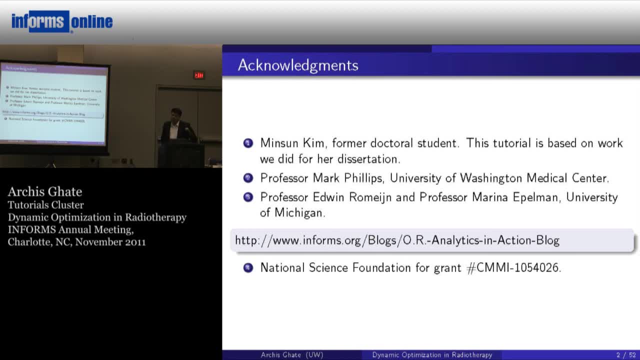 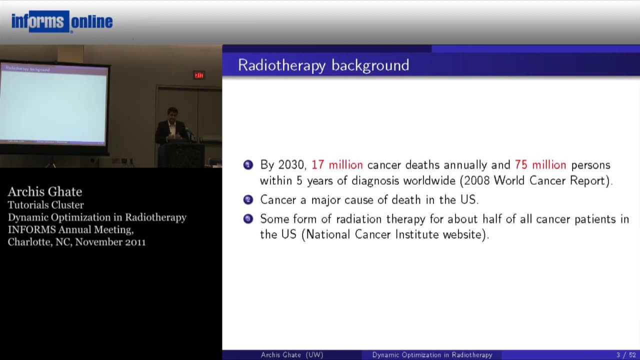 and then, last but not the least, National Science Foundation. so some of my current research in this area is actually funded by a grant from them. so that's why I'm acknowledging them as well. so let me get started. so I'm assuming that people here basically don't really have a background in 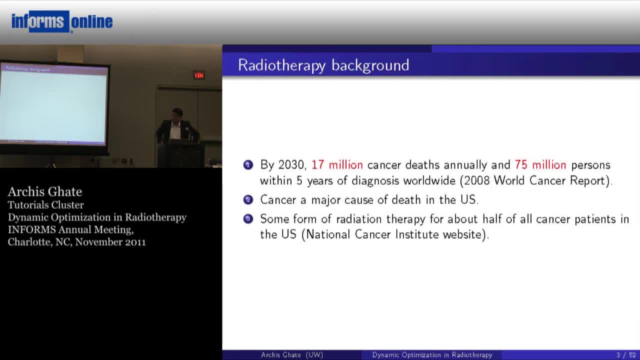 radiation therapy. so I'm going to start out with some basics, not spend too much time, but at least talk about it enough, such that everybody is on the same page when I use certain words or terminology or notation later on in my talk. some basic background in radiation therapy, so. 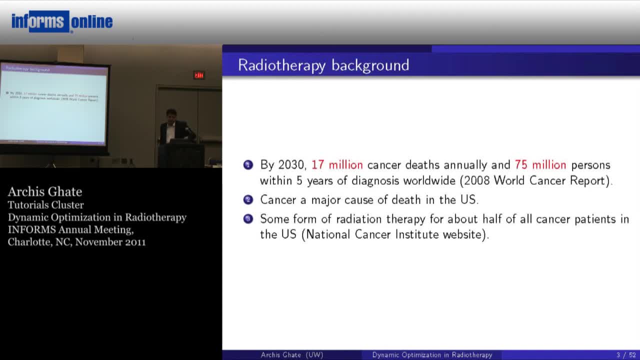 millions of people have cancer and will continue to have cancer all over the world. so World Cancer Report we put 2008, predicts these two numbers: 17 million and 75 million in the us. I believe cancer is the second leading cause of death. I believe second only to. 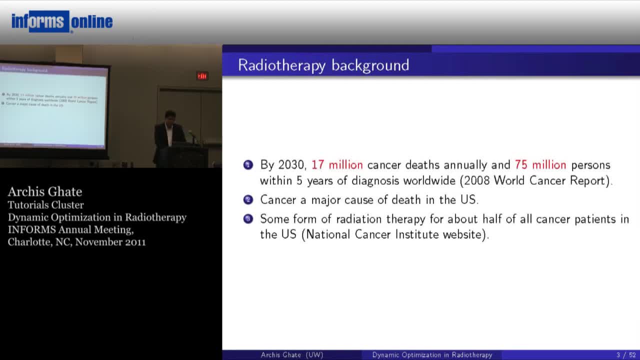 heart disease. so in the us also a lot of people are do have cancer and in the And in the US about half of people who have cancer actually receive some kind of radiation therapy. So, as you know, there are different ways in which you can treat cancer, For example, chemotherapy, surgery, radiation therapy. So about half of them actually receive some form of radiation therapy. 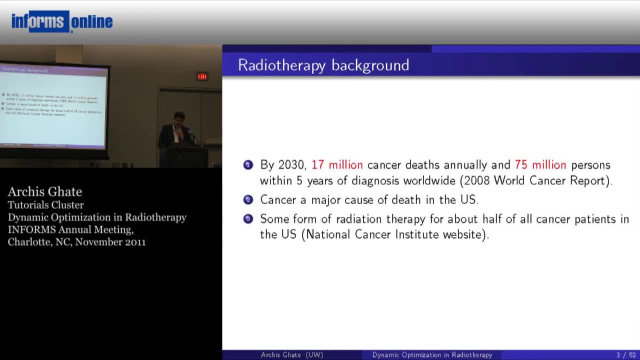 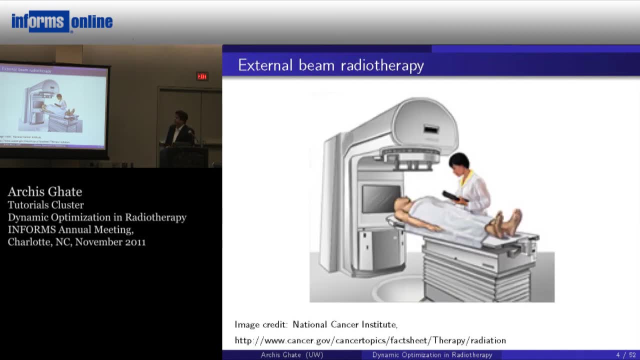 So all this stuff- you can read that from the National Cancer Institute website. So the talk today actually is going to focus on one particular kind of radiation therapy, which is external beam radiation therapy and, as the name suggests, you can guess that that basically means that the beam- so radiation beam- is going to come from outside the patient's body. 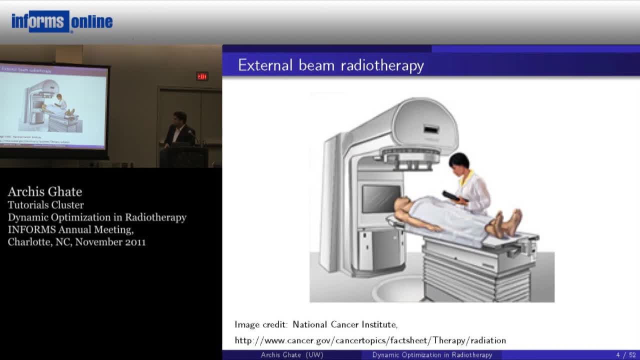 So that's what external beam means, And this is a picture I found on, again, National Cancer Institute website that basically shows you know the basic setup of how this works. So there's a couch on which the patient is actually up there and there is a machine which basically is connected to a linear accelerator. 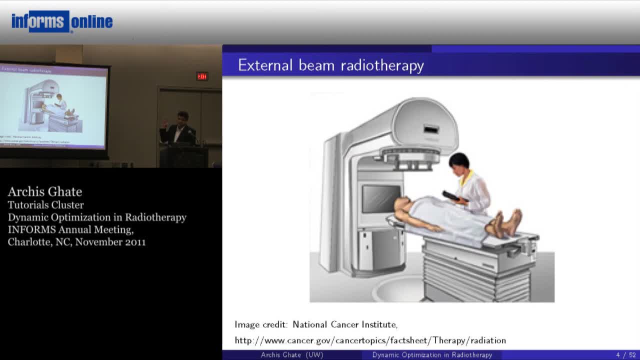 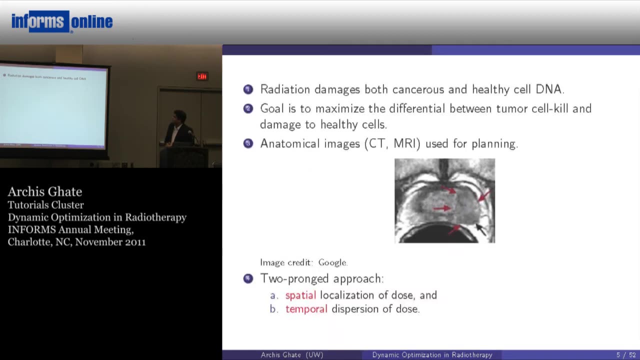 It's called a gantry which can rotate and pass radiation through the patient's body. So that's the idea in external beam radiation therapy. So that's the basic setup. So what are some of the key issues in radiation therapy? So I think most of you know this. 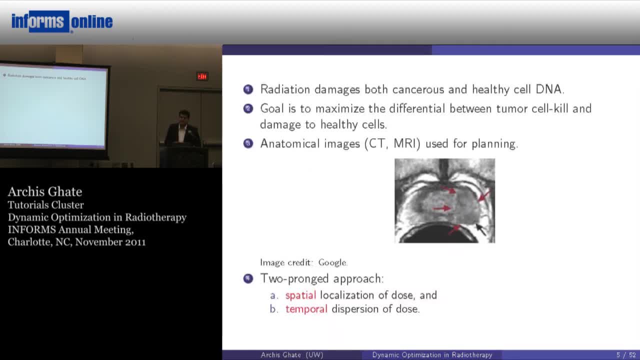 But the idea is that radiation is going to kill tumour cells, and that's good, but unfortunately it's also going to kill healthy cells that are right next to the tumour cells, for example. Okay, so that's a big problem, And therefore the goal in general is to maximise essentially some kind of a differential between how much tumour you kill and how much damage you actually do to the healthy cells. 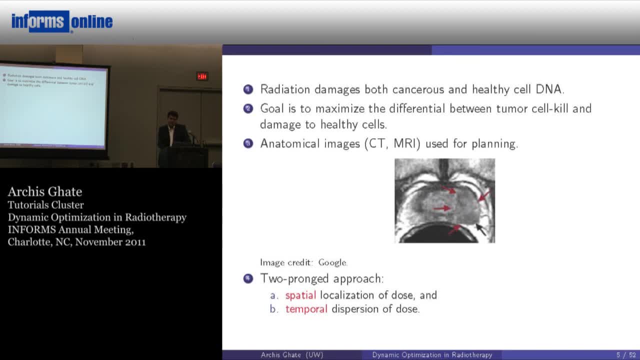 That makes sense right. So that's the key high level idea in radiation therapy And in particular, external beam radiation therapy. So the way this typically works at a high level, conceptually at least, is that you have to plan treatment for a patient. 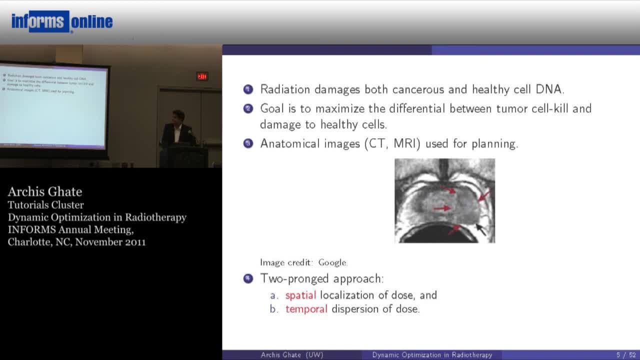 And you can start off by taking an image, so a CT scan or an MRI scan, And the image will basically show you roughly where the tumour is in relation to the patient anatomies or other parts of the patient's body, And this is something I found on Google. 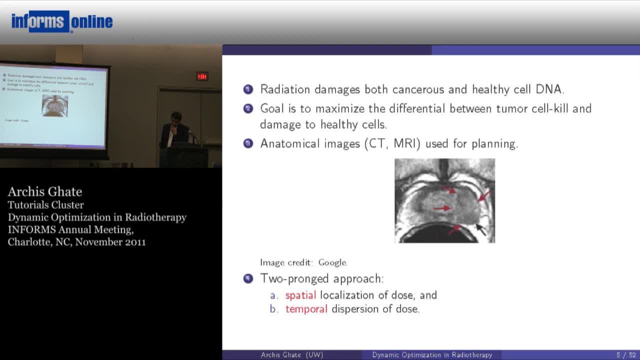 So this is, I believe, an MRI scan of prostate cancer, and the arrows basically kind of delineate a darker grey portion which is basically the cancerous region. Okay, so that's how you can kind of see cancer or tumour in an image which is an anatomical image. 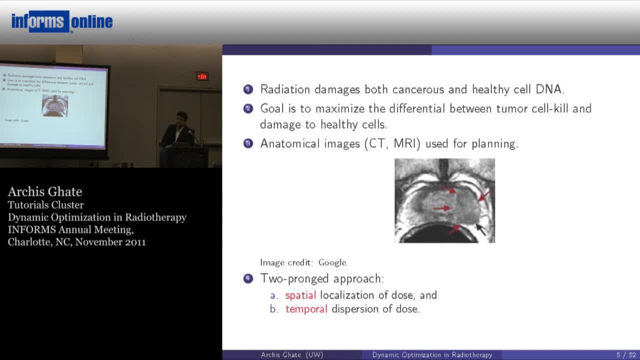 And I am kind of emphasising this word anatomical here, because later on in the talk I am actually going to talk about something called biological images, which are going to be different from these kinds of images, And when you see this image you can see that it's not just an anatomical image. 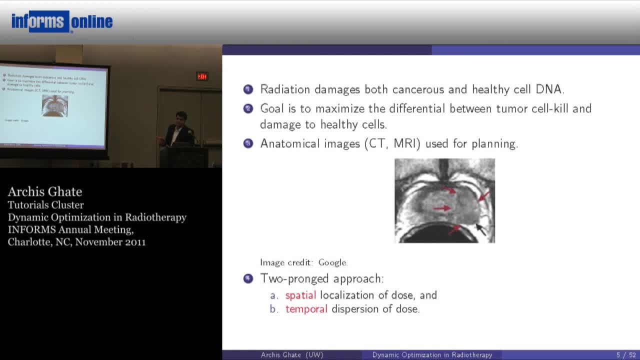 It's an anatomical image And when you see this image you can see that it's not just an anatomical image. But if you see the picture that I show you later on, you will notice the difference. So keep this picture in mind. 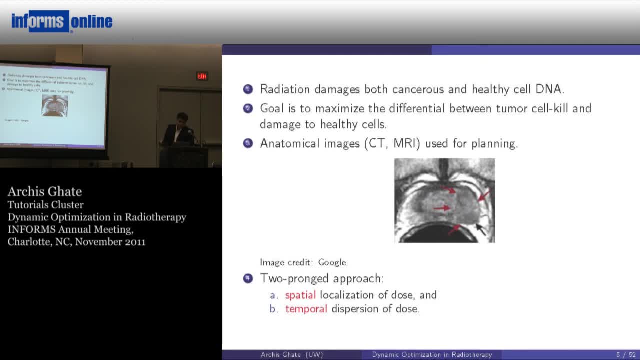 You can contrast that later with something else that I'm going to show you. So once you have an idea about where the tumour is in relation to the patient anatomies or other parts of the body, The way the goal is, kind of the group maximising the differential, the goal kind of is attempted to reach that goal. 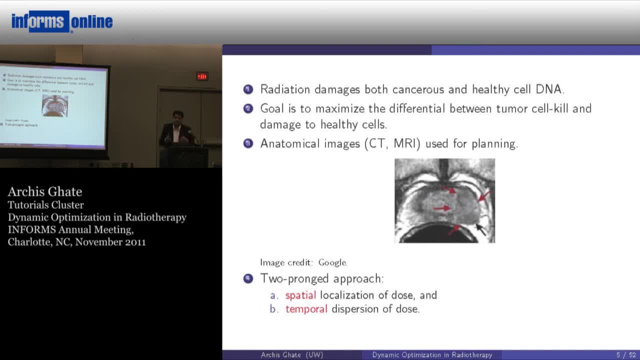 The way the goal of maximising the differential, the goal kind of, is attempted. So to reach that goal, What people do is follow two principles, two pronged approach. So basically it had to do two different things to reach that goal. 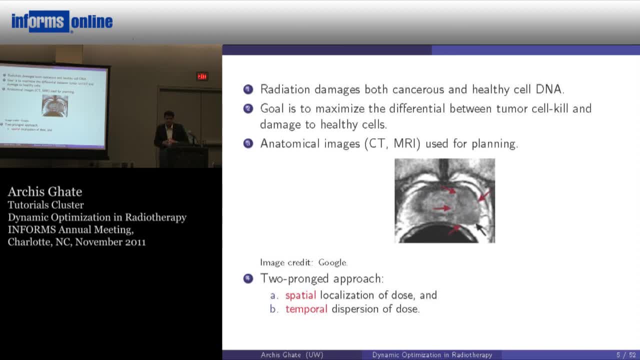 And the first is called spatial localization of dose And, as the name suggests, this has to do with space. And the second is temporal dispersion of dose, So the second, of course, has to do with time. So, on this two pronged approach, the idea is that. so in the first, 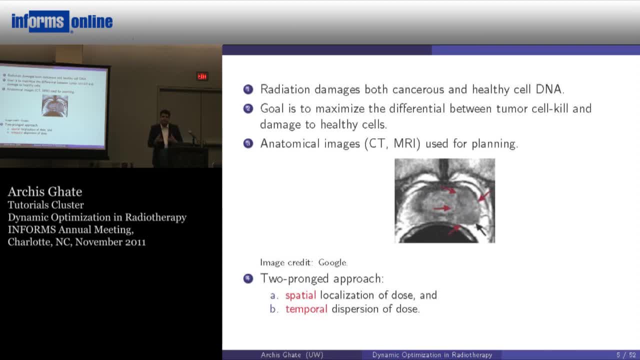 search bullet, A spatial localization. So the idea is that you give more radiation to the cancerous tumor as compared to the healthy cells. So you somehow manage that. So you design your treatment such that the dose- so in this context dose means energy per unit- 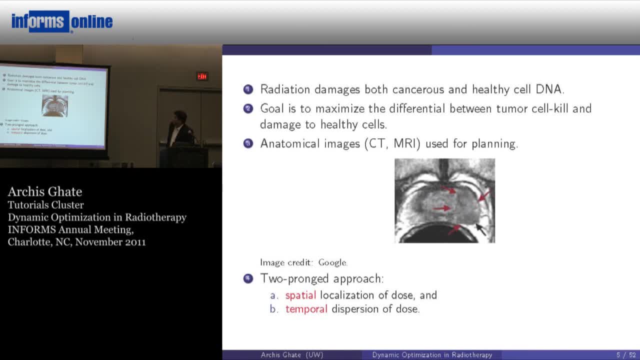 mass And the unit for that is gray. So the dose is localized or it conforms to the shape of the tumor. So that's the high level idea. So that's spatial localization And temporal dispersion, and I talk about these two in detail. basically relates to 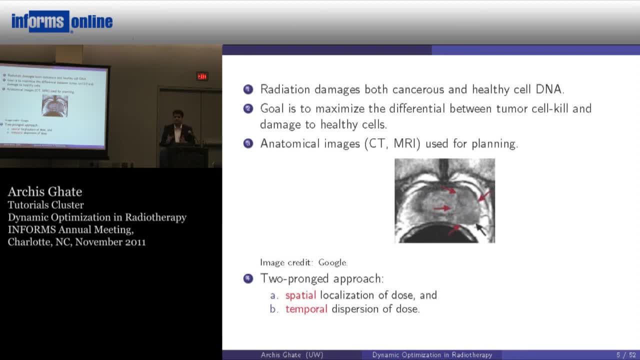 the fact that you're actually not going to give the entire treatment in one shot, but you're going to give it over time, okay, in smaller portions, essentially Okay. so that relates to temporal dispersion And we'll see why that is done after a few minutes in. 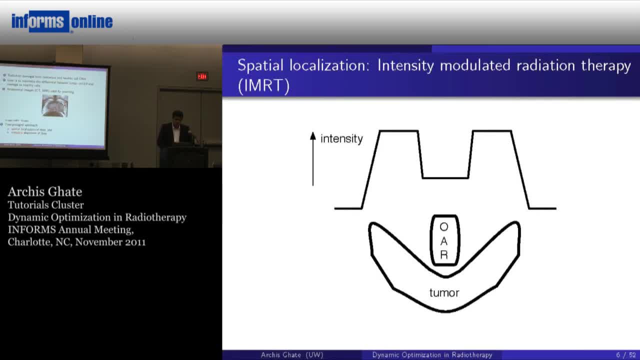 the talk today. Okay, so I'm going to talk about spatial localization for a little bit, just as background- some basic high level- And then go on to temporal dispersion. So spatial localization, this is just a simple picture that I drew to give you intuition behind the key idea here. So the picture shows: 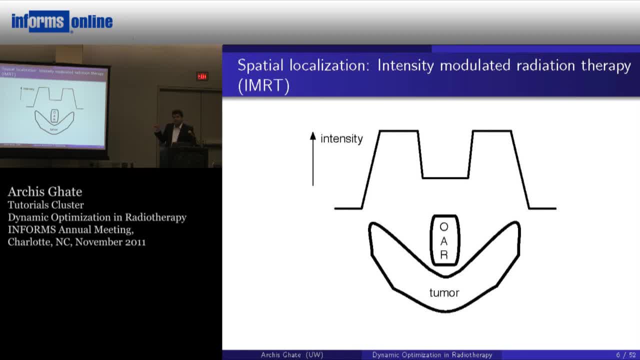 a boomerang shaped tumor And the letters OAR stand for organ at risk. Okay, so that's basically healthy anatomy in the patient's body. I'm going to use different kind of names for OAR, So I just interchangeably use words like normal tissue or healthy tissue And. 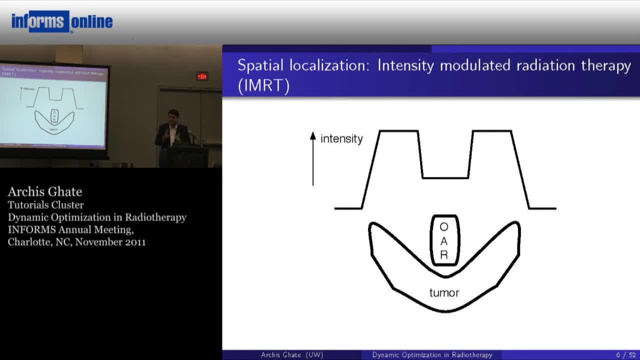 I'm going to use healthy cells, normal structure, organ at risk. all these things I'm going to use interchangeably, But basically that is something that will be damaged if too much radiation is given to that. Okay, so that's something that you want to protect, And tumor. 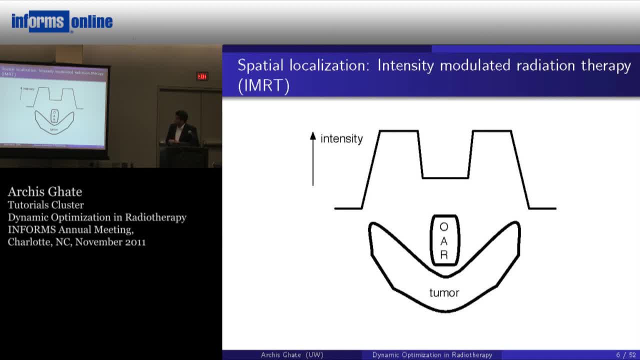 is something that you want to kill. So the idea of spatial localization, as you can see in this picture, is that you do something called intensity modulated radiation therapy, which basically means that you're going to modulate the intensity of your radiation field or radiation. 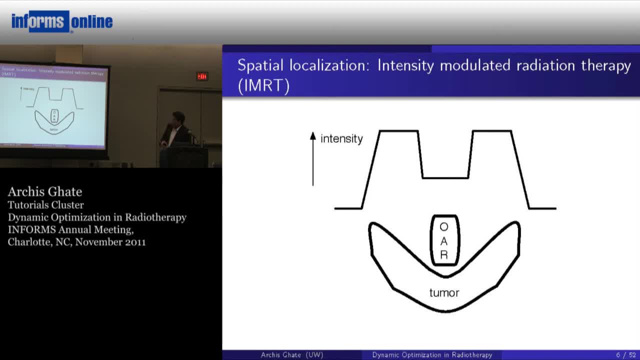 beam. This is shown in the picture. So what I'm trying to show there is that the intensity. so the arrow goes up so high that way. So, as you can see, the idea is that you have a dip in your intensity profile near the OAR, near the organ at risk, right, So you want. 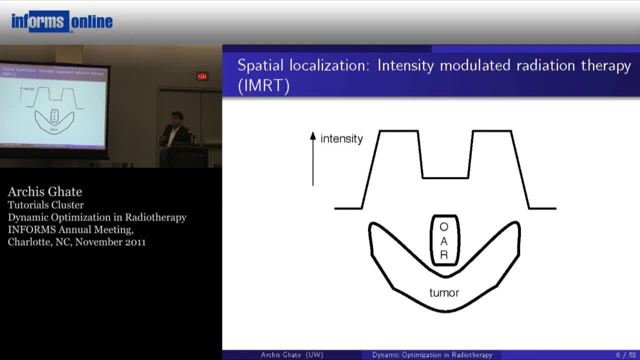 to give very high intensity to the tumor and low intensity to the OAR, Making sense right, So that the OAR will be protected. So that's what is shown in the picture, So that's the basic idea in intensity modulated radiation therapy. So I'm giving as you can. 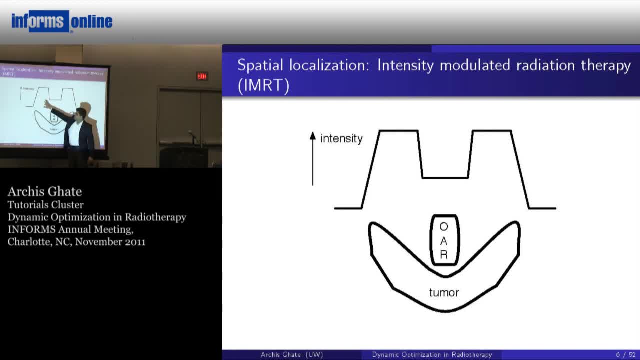 see, go here, high radiation here and high radiation there, And I'm trying to avoid giving too much radiation here. okay, because there is an organ at risk. If you want more concrete example of where this can actually happen, so something like this can actually happen. 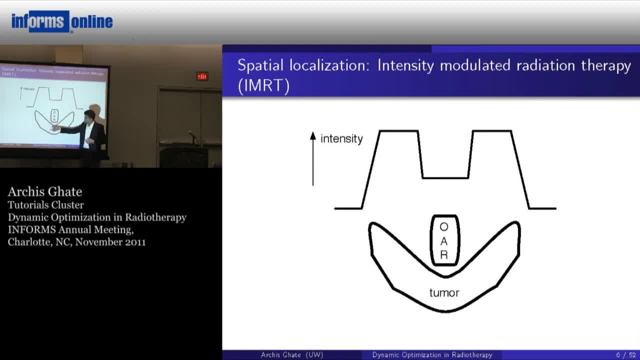 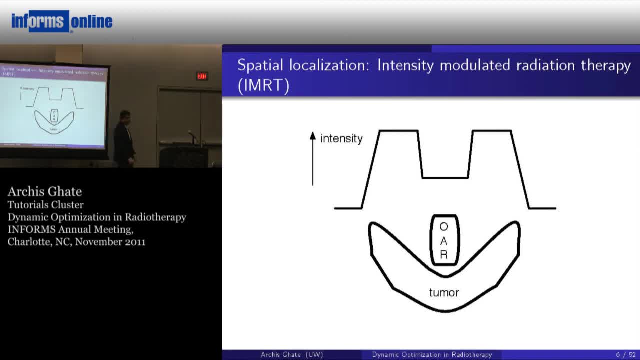 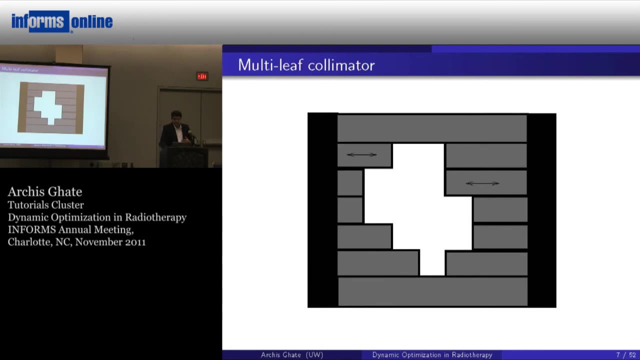 cord looking from top. The reason I did not draw a circle because it was hard to fit the three letters OAR in that circle. But it is easier to imagine a circle for spinal cord looking from top. okay, So that's the idea, And then, so how is this done? So how? 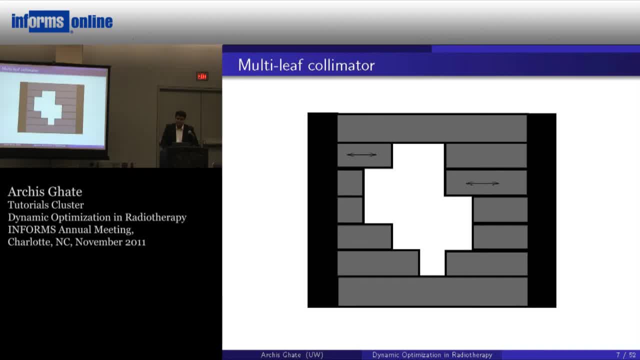 do you actually modulate this intensity profile, And that is done by something called a multileaf polymerator. So this is basically a bunch of leaves that can move like this, as shown by the direction of the different arrows, the two arrows, and basically the radiation is going to come. 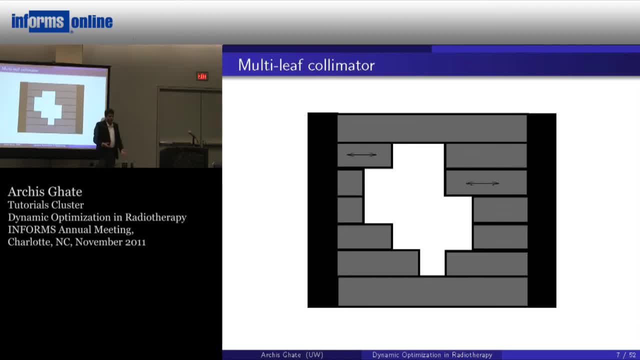 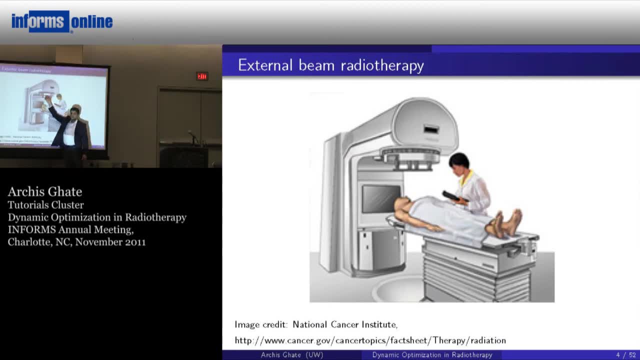 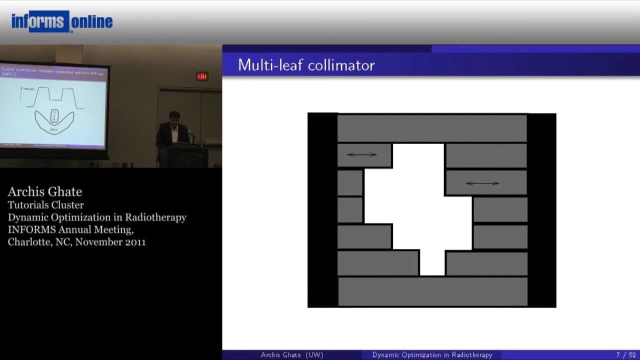 from here, for example. right, so this is an opening in my machine, so in my gantry. if i go back, this is going to be somewhere over here, right, and radiation is going to come from top right and the idea is that the leaves that you have, so these leaves, are going to move such that you shape the beam appropriately, so that right it. 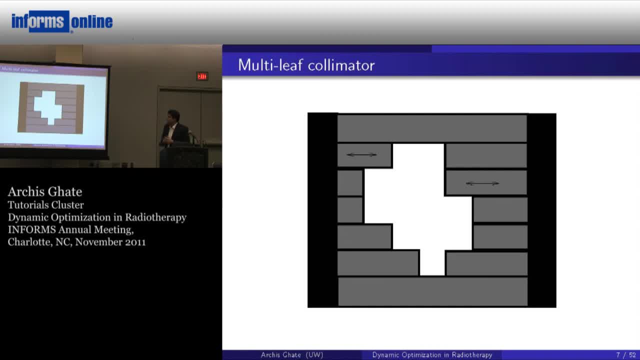 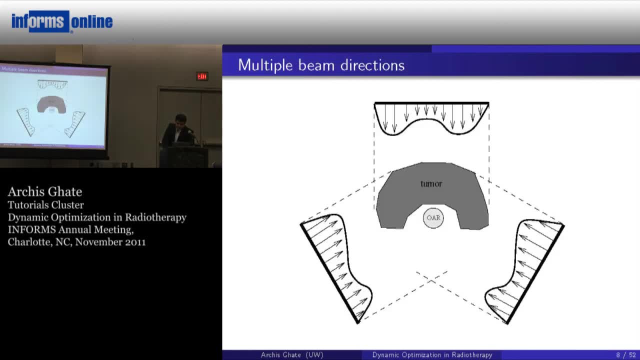 conforms. so the radiation that you give conforms to the shape of the tumor. that's the idea, basically, and that can be done using this collimator, for instance. okay, so that's the basic technology in imrt. and then this picture actually gives you some intuition behind why people actually use. 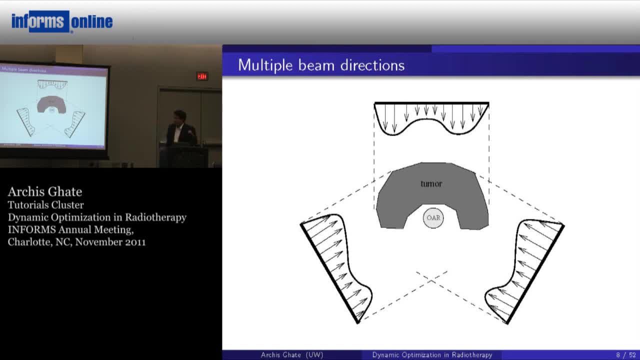 multiple beam directions rather than just one direction while giving treatment. so this is just something that i drew. so again, i'm trying to show, you know, the head and neck kind of example that i gave you. so this is that tumor wrapped around. if you want think of this as the spinal cord, so organ at risk, something that you want to. 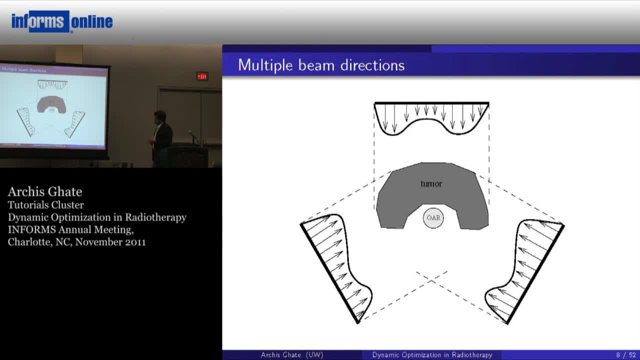 protect, not damage too much. so the idea is that if you look at the top beam, top field, you would want to have this kind of a radiation profile for that intensity profile for that. and the reason is, just like in my earlier picture, you don't want to pass too much radiation through this part, right? 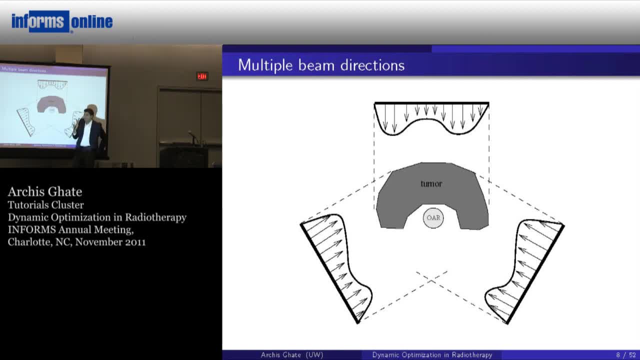 so that's why there is the dip there. but the bad thing about that dip is that you will actually end up giving less dose than you want to this part of the tumor make sense because there is that low intensity portion there and that is called a cold spot- just not enough radiation to kill tumor. 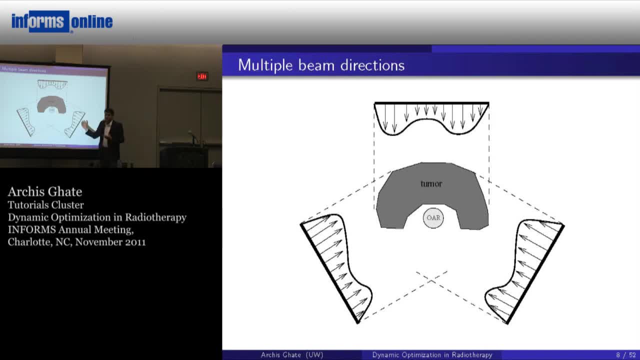 so the idea is that, to avoid something like that, you're actually using multiple directions. so, being from multiple directions, so this is another beam and, as you can see, i'm actually using high radiation here. so the hope is that you know this will compensate for this cold spot, essentially, okay. so whatever was you know kind of lacking, this will make up. 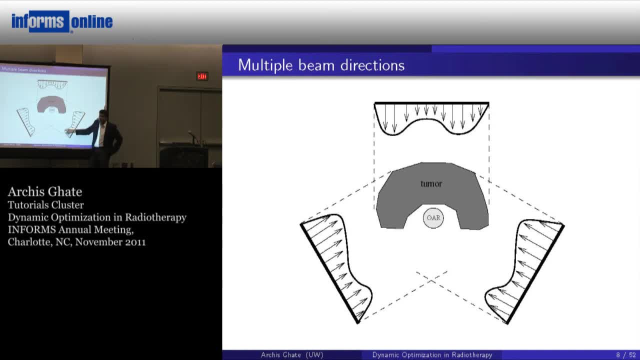 for that, and of course, i have to have a tip here as well, because i don't want to have a high intensity here to protect this oar. okay, right, and the same idea with that beam as well. so that's basically the whole idea of the oar and the same idea with that beam as well. so that's basically. 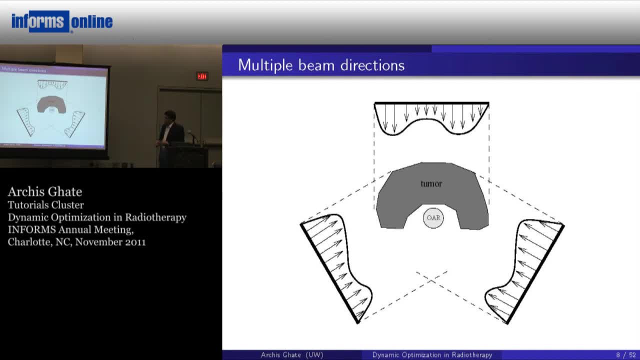 why you would use multiple beams and that kind of depends on the geometry of the tumor in relation to your organs at risk. so for something like this, you know, this concave kind of geometry with an oar that is hidden inside, multiple beams will actually make sense, okay. so any questions so far? 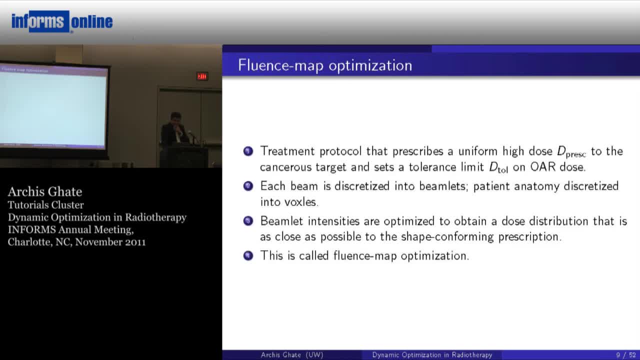 okay, okay. so that's the basic idea. so the? so the way treatment is planned is by doing something called fluence mapping. and what is that means? if you have an oar that is hidden inside multiple beams, map optimization. So fluence map is basically the radiation intensity profile. So this 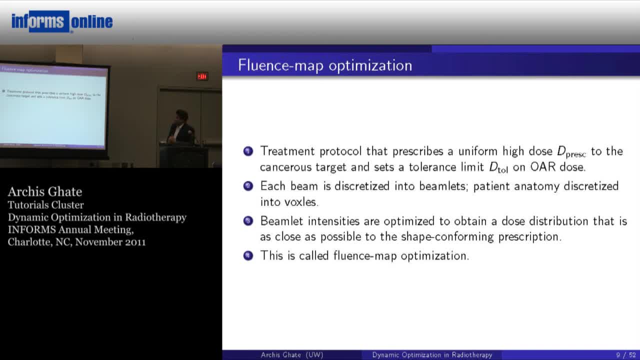 is actually called inverse treatment planning. It is called inverse for the following reason: So you actually start off by specifying a treatment protocol- and a doctor can do this- That is based on empirical, so clinical evidence and experience and other guidelines and so on. But basically you start off with a protocol that describes, let us say, a uniformly high 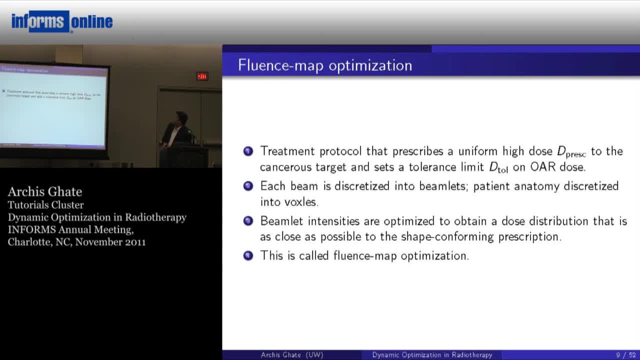 dose, called prescription dose, So the risk to the cancerous target, so the genital tumor area, and basically set some kind of a tolerance limit and I am going to call that DTOL for tolerance, So limit on the OAR dose. So the idea is that I want to give, so ideally. 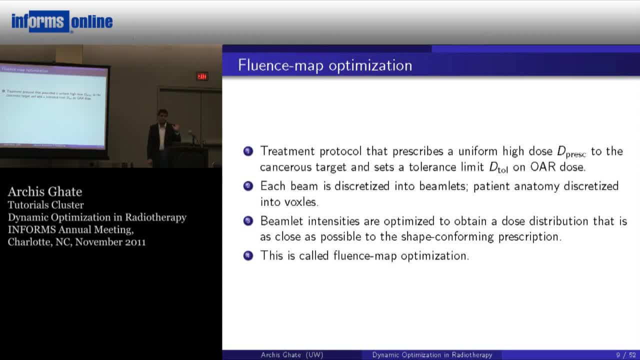 speaking, I want to give as much dose as possible really to the tumor without giving too much dose to the organ at risk. That is the rough idea at a high level. But here there is a prescription, So the doctor is saying that, okay, give this dose to tumor and do not give more than. 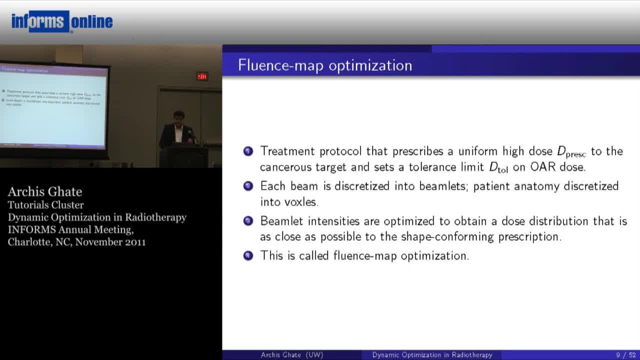 DTOL to the OAR. So that is one example of a simple, really the simplest protocol probably. And then, if you start thinking about how actually you do this, in mathematical models of these kinds of problems, each beam is actually discretized into smaller segments called beamlets, and 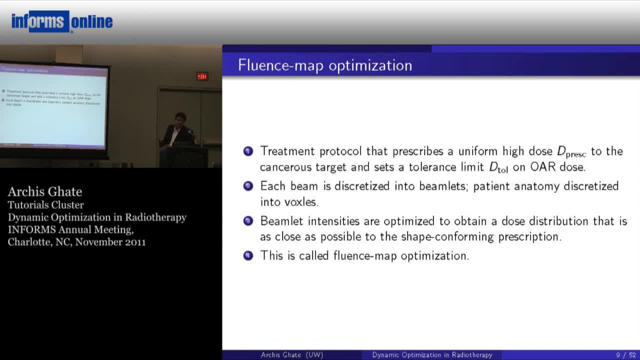 the patient's body, tumor region, other anatomy nearby is discretized into something called voxels. So voxel is just like a pixel, but three-dimensional, So three-dimensional cubes, you can think of them like that. So that is done in mathematical models. And then the beamlet intensities of 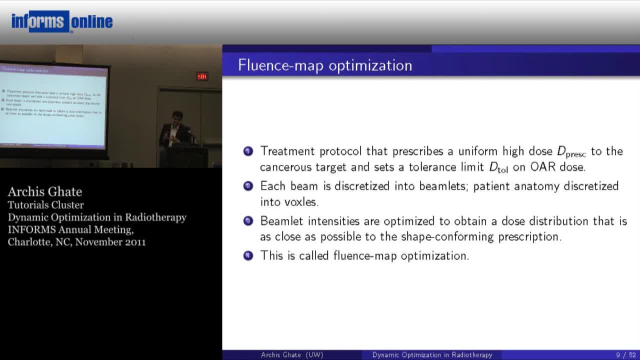 these small portions of the beams, so the intensities there are actually optimized to obtain a dose distribution that is as close as possible to the prescription right. So doctor is saying: do this. perfectly achieving that may not be possible, So you are trying. 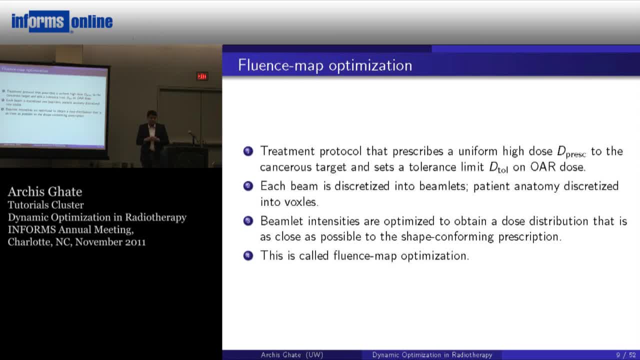 to do as close as possible. So that is how kind of optimization comes into play, because you are trying to do something as close as possible to this prescription. And this is basically- you can think of this as a basic fluence map optimization problem. 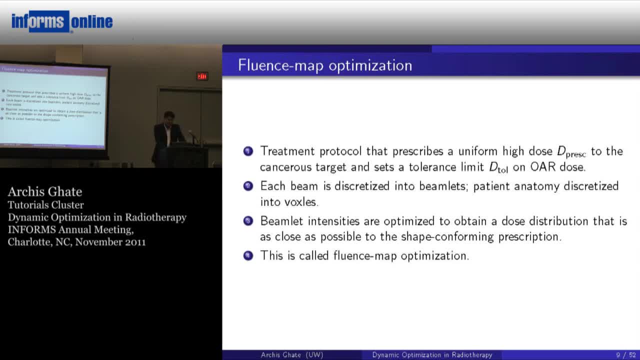 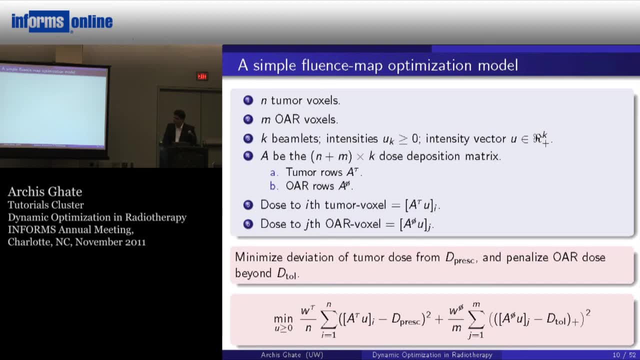 So what I will do is actually just to get started. I will give you a very simple example of a fluence map problem. This was one of the very first models that I think was formulated in the mid-90s, I believe. 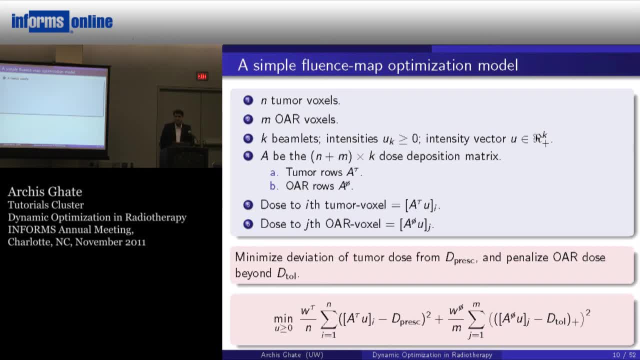 So let me give you some basic notation. So this is a tutorial as opposed to a 20-minute talk. So I am going to have some math here with notation and so on, much more detailed than a typical 20-minute talk. okay, So I am going to start with some basic notation. 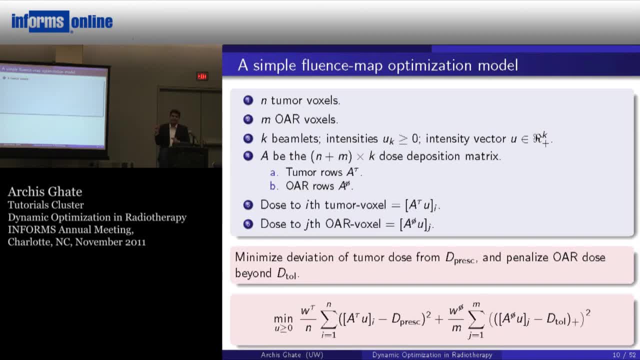 So remember I talked about voxels, so small 3D cubes in the patient's body. So let's say that we have N tumor voxels, M, OAR voxels, K beamlets, And let's use the letter U here. 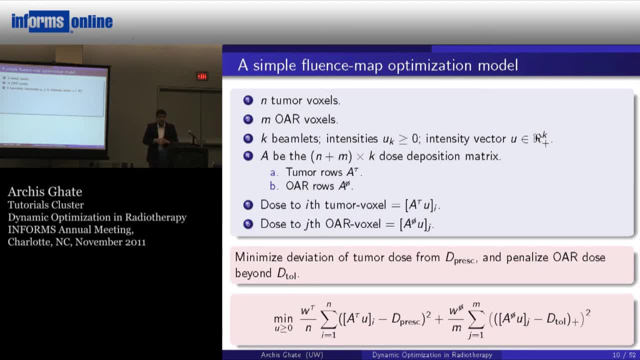 that is the U throughout this talk to represent intensities. So I am going to have intensity vector U. intensities have to be non-negative, So that intensity vector is in R plus K dimensional because I have K beamlets make sense. So that is the basic notation of 3 things. 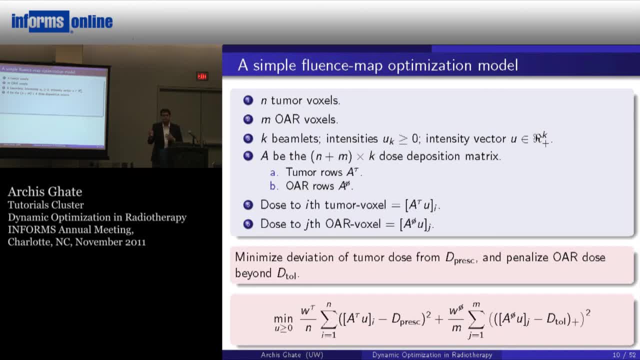 And then think about it. if you want to plan treatment, if you want to start thinking about formulating an optimization problem, what you will need is: somehow you will need to. if I use these intensities right, how much dose will actually be delivered to the patient, right? 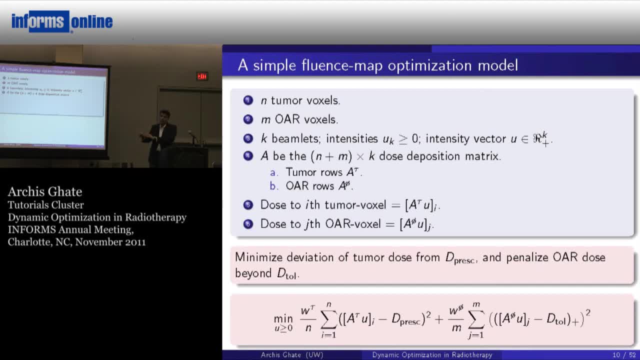 different parts of the patient's body. so how much dose will go to that corner of the tumor versus how much dose will go to that corner of the organ at risk, right? so you want something that transforms the intensities into dose, which is energy per unit mass. okay, and that's called. 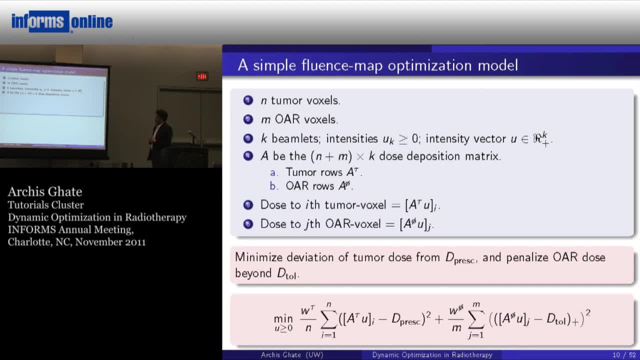 a dose deposition matrix. so the transformation is going to be linear, basically. so a is the letter I'm going to use for my dose deposition matrix, and the matrix is basically n plus m times k. okay, so it's going to have k columns, n plus m rows, and the idea is that I take this a, multiply my u, which. 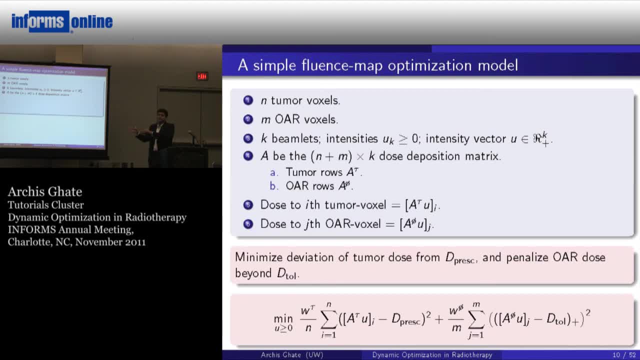 is the intensity vector with this a right, and what I get will be the dose. okay, and so I'm going to use letter tau throughout this talk to represent things that have to do with tumor and the letter phi to represent things that have anything to do with the OAR or normal tissue. so basically, if you want to think, 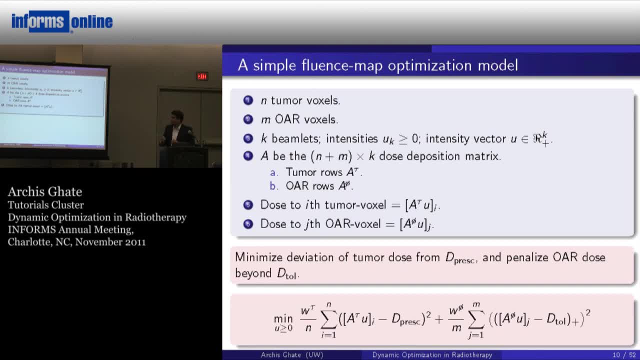 about what dose will be given to the ith tumor voxel. it's going to be my tumor dose deposition matrix times my intensity vector. so I do that product and pick up the ith component of that. okay, so that will give me the dose that is deposited to the ith little cube inside my tumor. 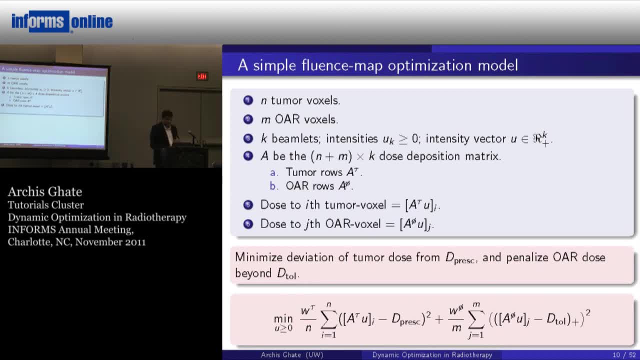 okay, so that's the idea, and then you can imagine exact same thing for the tumor, and then you can see that everything will be true for that a phi, which is my OAR dose deposition matrix. so I multiply that with u and take the jth component to figure out how much dose will be delivered to the jth OAR. 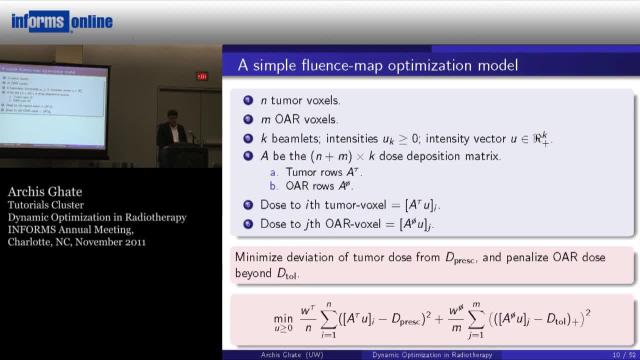 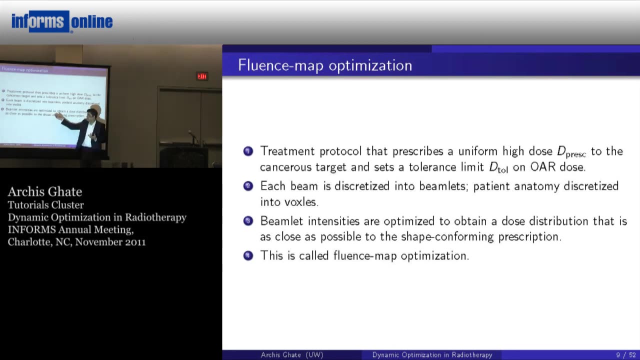 voxel. okay, so that's basic terminology that I will use again and again throughout this talk in different contexts. so let's go back to what I had said a minute ago. so remember I had said: you know, the big kind of the basic idea is to somehow figure out, you know, an optimal intensity vector. 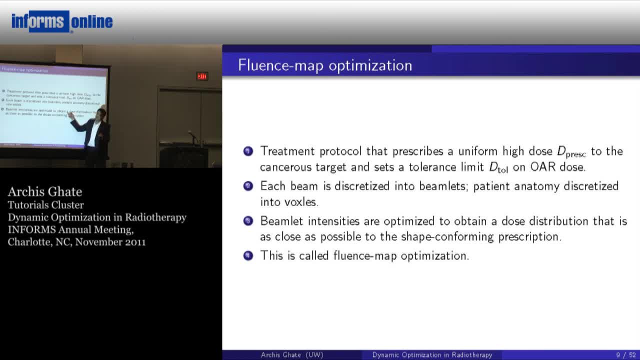 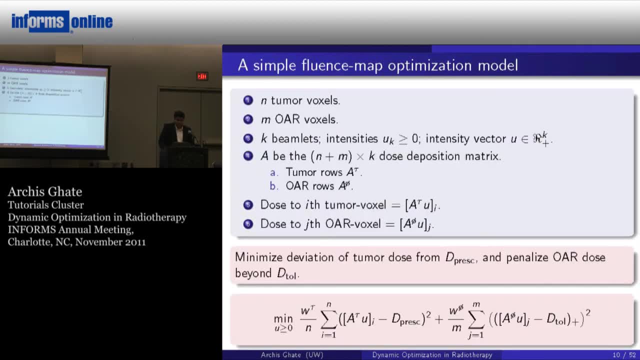 such that what is delivered to the patient will be as close as possible to the prescription. okay, so I'm going to write down a very simple optimization formulation for that problem. so what I'm going to do is I'm going to minimize deviation of the tumor dose from the prescription dose that the doctor 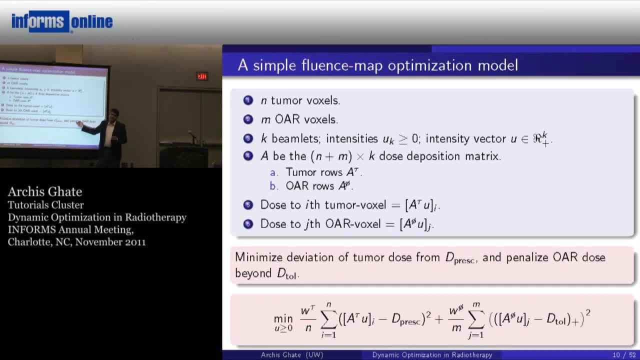 told me right, and I'm going to penalize anything to the OAR that is above the tolerance limit, right? yeah, do you worry about like discretization errors on the boundary? so some voxels are going to be both, I guess. sure, in some sense, I think the 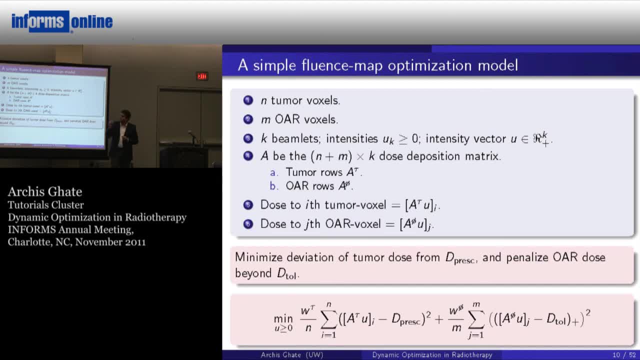 voxels are very small, like five millimeter by five millimeter, one centimeter by five centimeters, but there will be small errors, I guess. yeah, does that. well, you could correct me, but I think you do identification of tissue, or at least you could do identification of tissue before you do the. 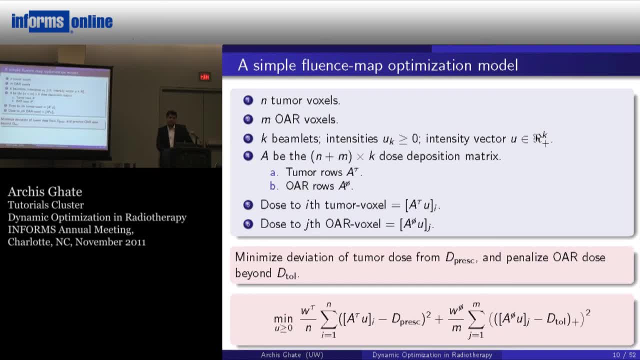 discretization, but you know, in some cases it's not a sensitization. there are some walks if you have lung cancer. some muscles are cancers, but they're part of the one. So in that, a formulation for that would look like this. So here what I'm doing is, like I said, I'm going to minimize. 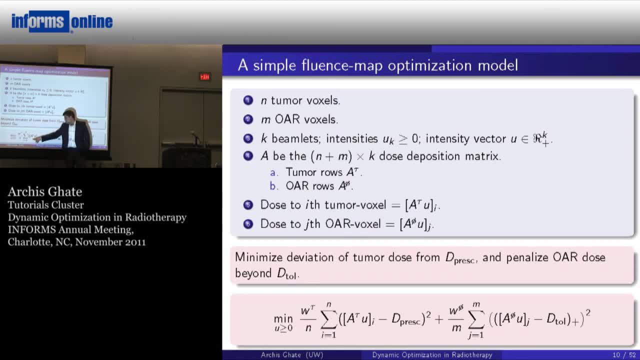 Squared deviation. So this, as I said, is the dose to the I Tumor voxel. so I'm subtracting the description from that square and summing up over all tumor voxels. That's the squared deviations sum, And talk about these things in a minute. So let's ignore that for now and go here. 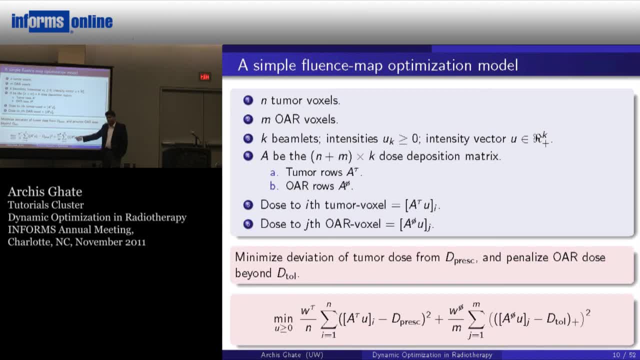 This is similar. So again, I'm calculating the deviation Again. so the dose to the OER jth voxel Subtracting the tolerance dose. The only difference is that I'm putting a plus sign here and what that is going to do is basically, it's going to take the maximum of this number and 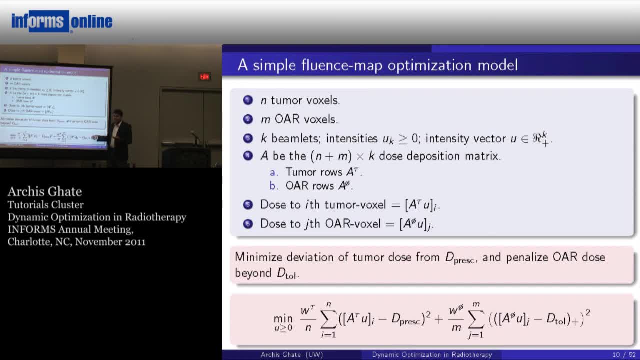 0 and then square that, and the intuition behind that is that I only want to penalize things that are About p-tall, but I don't want to penalize things that are below. Okay, so that's the idea and I sum again over all OER voxels. 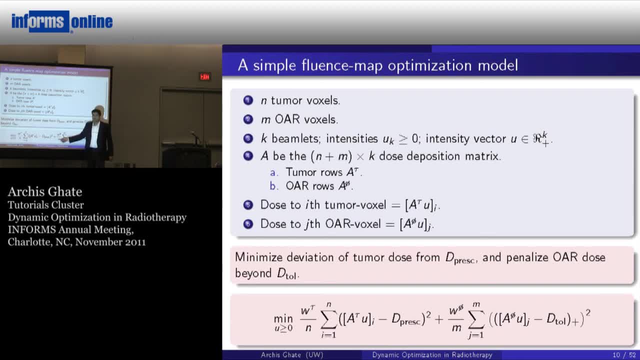 This N and M remember N tumor voxels, M OER voxels. So these are just normalizations, Basically, and these are weights, so we can think of these as importance weights in some sense. This is a multi-objective problem, So you can think of those as importance weights being attached to the tumor versus the OER. 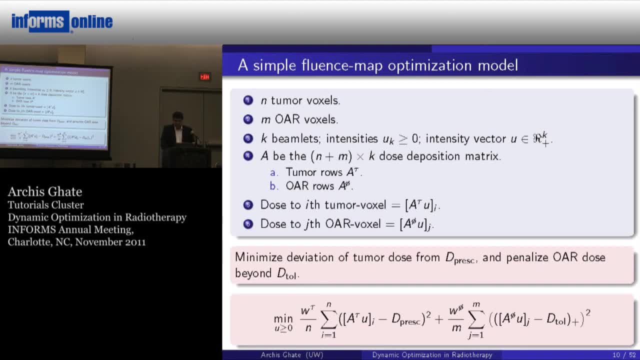 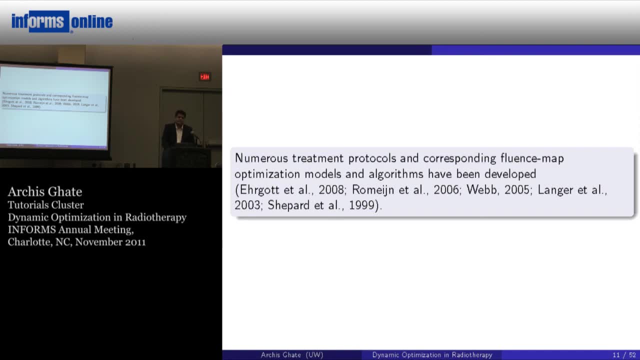 So that's one of the, I think, early Models for this fluence map optimization. and then since then, so since mid to late 90s, Millions and millions of different models have actually come out, I believe, different kinds of treatment protocols. When you have a different treatment protocol, your model will correspondingly change. right, then your algorithm for solving that might change. 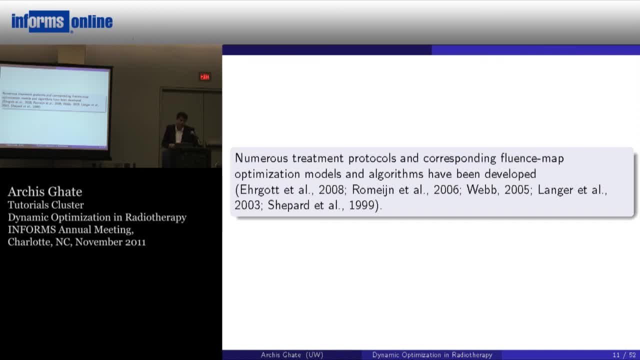 And so on. so these are some of the surveys that I found that talk about different Protocols and the corresponding different models. Okay, so you can take a look at those later if you want. One thing I want to mention is something called dose volume protocol. 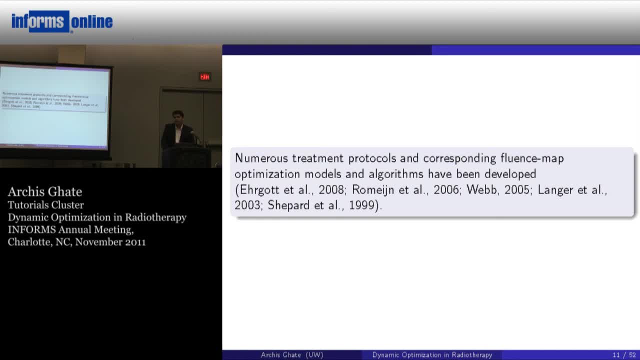 Which is commonly used. so that says something like: not more than 30% of the organ at risk should receive more Than a certain amount of dose. Okay, so that's the dose volume protocol, And typically I believe that is a model using some kind of a mixed integer programming formulation. that makes the problem difficult to solve. 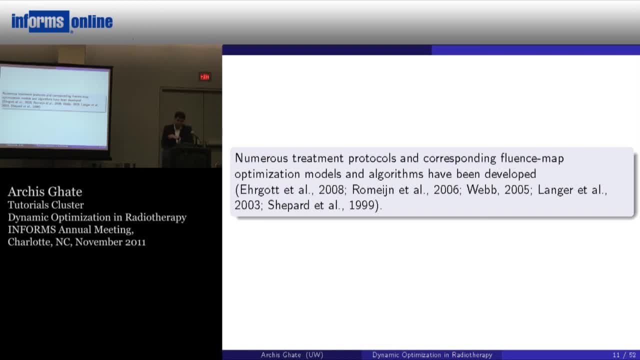 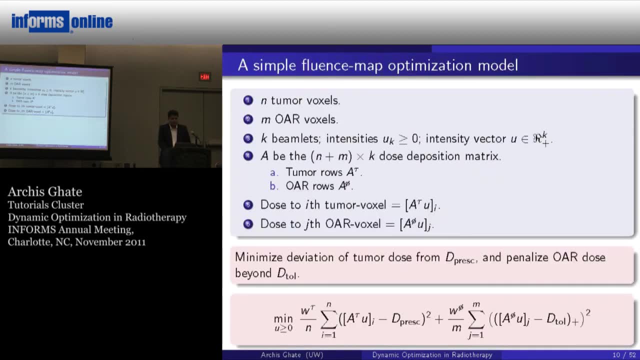 But that's one thing. that is not a part of what I showed you earlier. What people have also done, and briefly touch upon this later on, is that- remember I mentioned Uniformly high dose in my protocol for the tumor. people have used non-uniform protocols based on some more sophisticated. 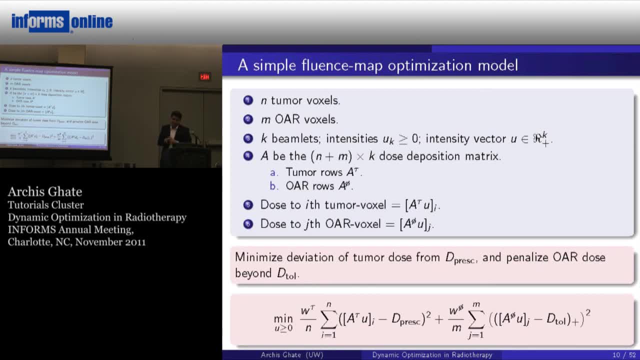 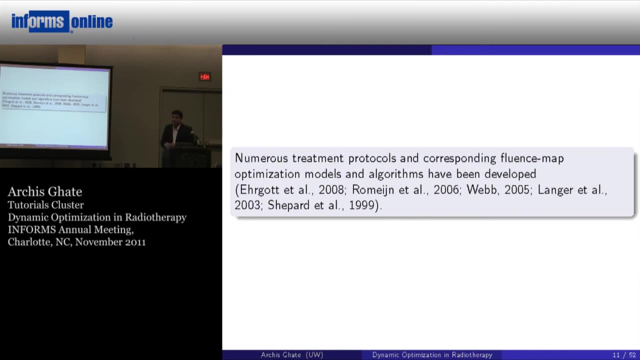 Images called biological images, and I talk about that a little bit later on Because those kinds of images are going to be relevant for the rest of my talk later on anyway. okay, So basically lots of different kinds of formulations of these spatial localization problems. yeah, Your objective function. is there a difference between using 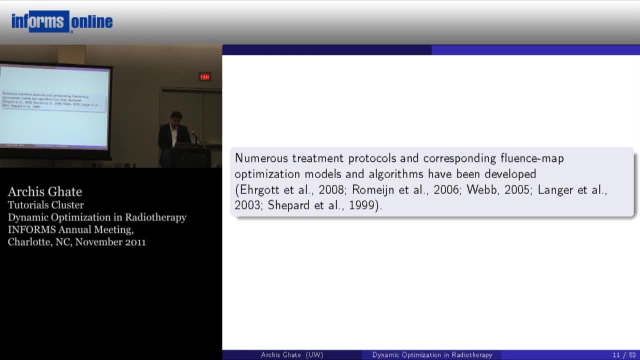 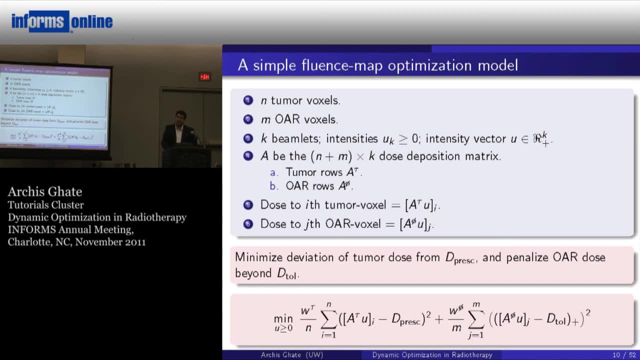 absolute value as objective function. Absolute value where, Where the number of pixels are involved. Yes, that could be done And in fact you can format that of a linear program also. Yeah, this is really just one example. like I said, there are millions there, But you're right, I could use other things as well. 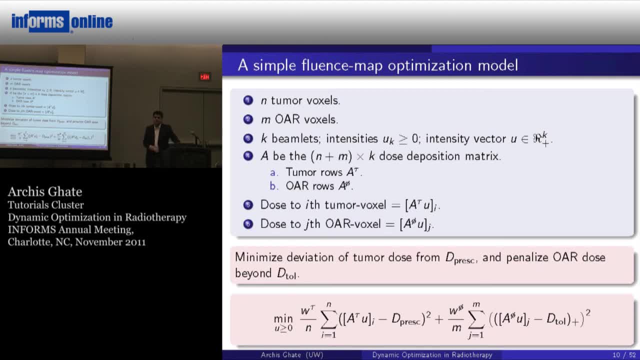 In fact, you know, sometimes some of these things can even go into the constraints Right, where I put that as a hard constraint instead of doing something like this and so on. Okay, So that supports spatial localization. so the second component is actually temporal dispersion of dose. So let me talk a little bit about that. 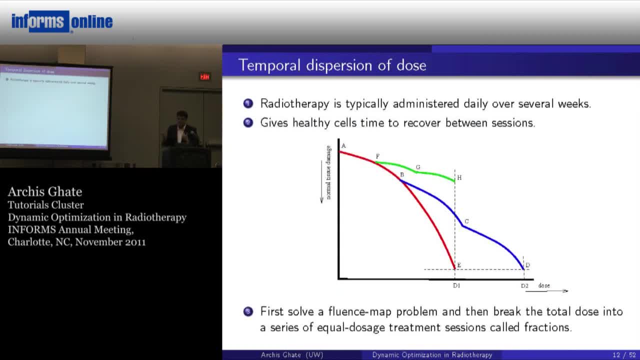 So, as I said before briefly, this radiotherapy is basically administered daily over several weeks, so let's say five to nine weeks. so the patient comes back again and again and a little bit of the dose is actually given every time, and the one of the reasons for this is that so healthy cells actually have 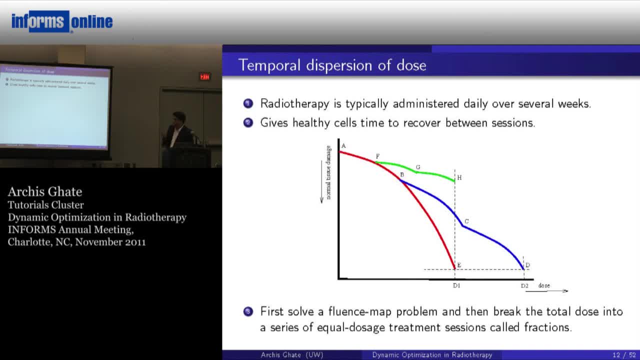 better ability to recover from damage than tumors. so the idea is that if you give eight to twelve hours between two treatment sessions, by the time the patient comes back, whatever damage was done to the healthy cells they would have actually recovered from that. So that's one of the reasons you actually 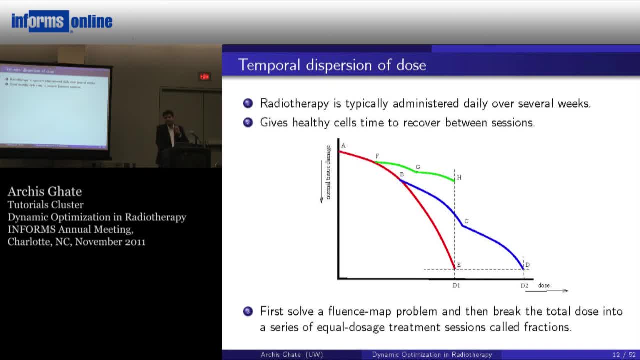 do this temporal dispersion. so rather than giving the whole thing one shot, you actually give it over several weeks. okay, I also want to talk about this picture that I drew in this context, because this picture will actually become important later on in my talk. So this picture basically shows conceptually: 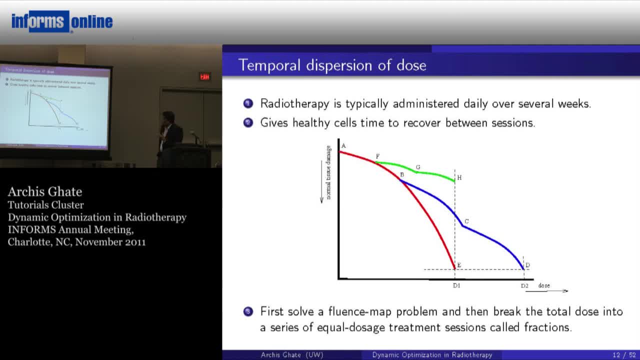 something like this. So this picture basically shows conceptually some thing called a cell survival curve or normal tissue damage curve. so let's just look at this. so the x-axis here is dose, so those increases this way, okay, and the y-axis is normal tissue or OAR damage, so that increases that way, right, so more. 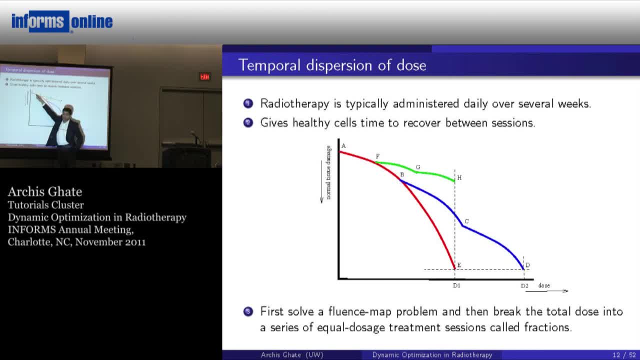 damage here as compared to up top there. okay, and so first you should look at the red line, which is this line. so basically, this says that if I give, let's say, this much dose in one treatment session, this much damage will be done to the OAR. okay, that's how you can think of this picture. so that's the 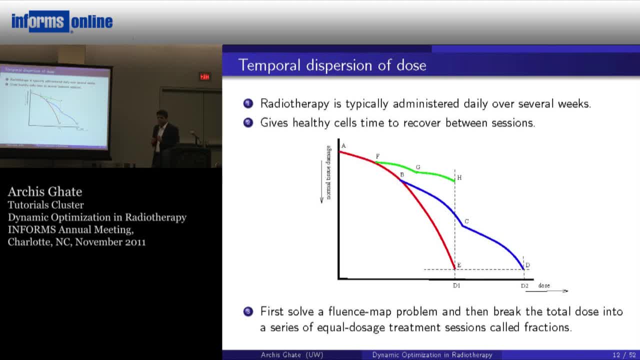 first red curve. what I'm trying to show here is that what happens if you actually break the dose into smaller portions, right, so two or three portions, let's say three portions, I believe, in this picture, and then you give that. so I'm trying to show two kinds of things in this picture, So the first one is the 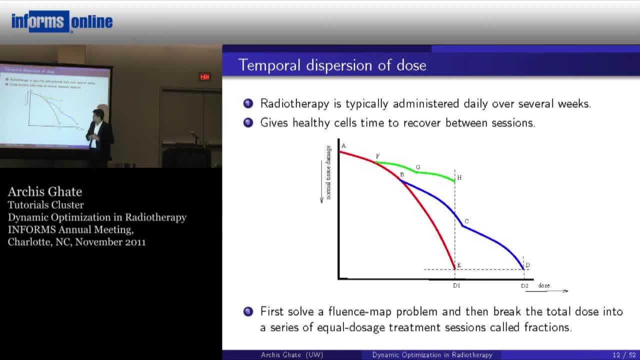 green part of the picture and the blue part of the picture. so if you look at the green part, you can see that, because the dotted line is vertical, right, the dose that I'm giving is actually the same as this D1, right? however, you can see that the damage that is done is significantly less right, and that's. 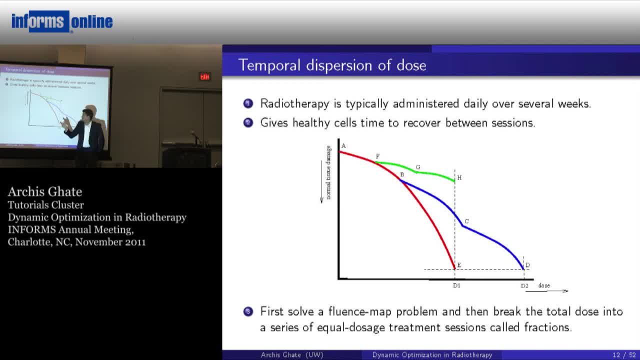 because that same amount of those D1 is actually broken into smaller portions and these are actually called fractions. okay, and I talk about that more later on. so that's one way to look at that. the other dual way to look at this is that, again, if I again broke my dose into smaller fractions, so three fractions, you. 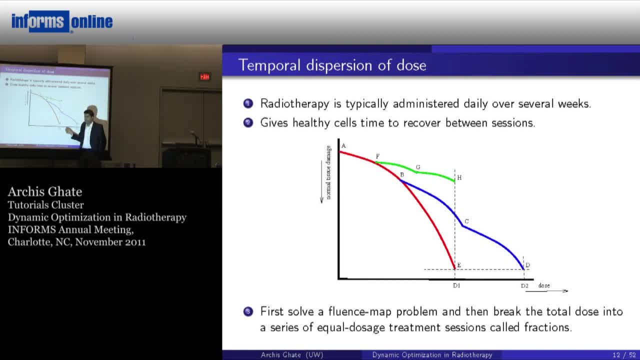 can see that I can give much more dose, which I'm calling D2, for the same amount of damage to the organ at risk. okay, so that's the dual of that earlier situation and that's important because I want to give as much as possible. really sense, right, because the more the dose to the tumor, the better it will be right. so 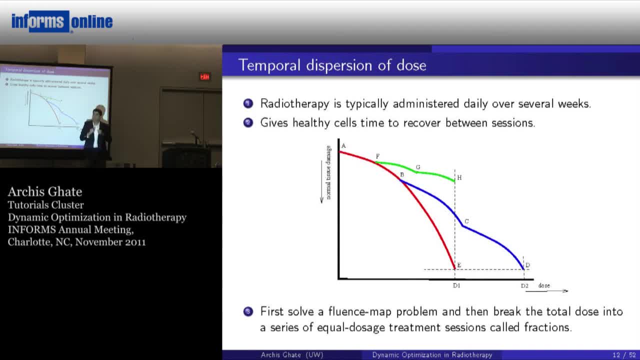 that's. that's why the dual part is also important. So why don't you assume that tumor cells are equally good at recovering? Equally good at recovering? I think that goes. that the reason is- I've just read this in radiobiology books- so just because tumor cells, I guess, behave differently from 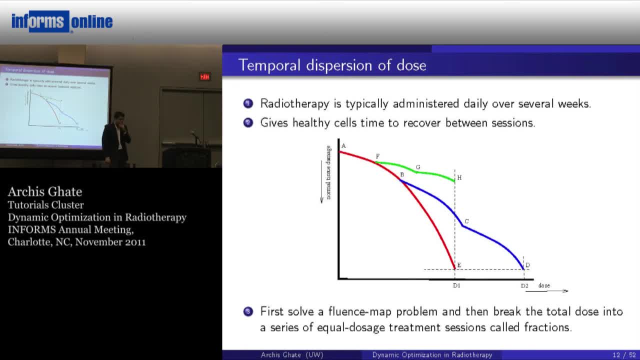 normal, healthy cells. that's the reason, basically, But I don't know more than that. I'm not a biologist, But that's, I think, correct. So that's this picture. I will come back to this picture again later on, but I think the basic idea is clear from the picture and in fact I will actually use a. 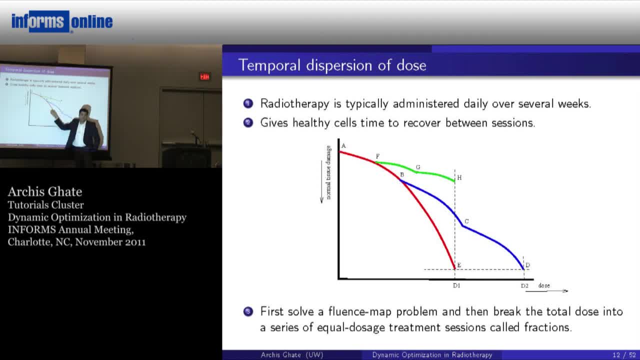 particular functional form later on to represent this curve that I drew here. I talk about that when I get there. So that's the idea in this temporal dispersion. so the way this is typically done is that you first solve a fluence map optimization problem, which will give you intensities and those. 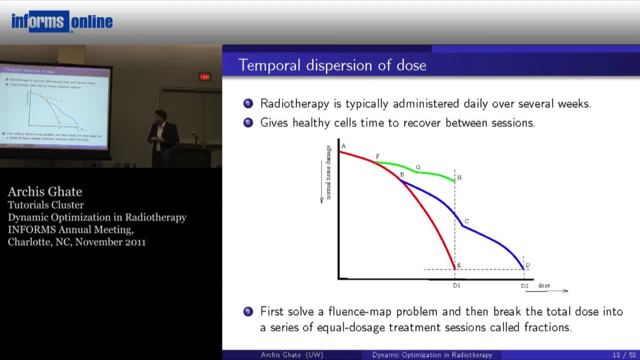 basically, and then you kind of break that total dose up into a series of typically equal dose fractions for treatment sessions and then deliver that okay. so for example, people say: this treatment is 2g per fraction for 15 fractions or 1.5g per fraction for 20 fractions, something like that. so 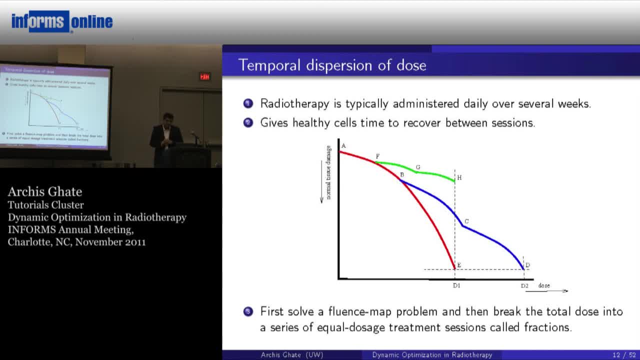 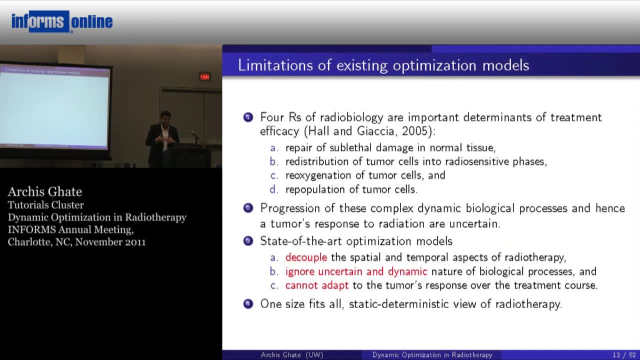 that's the most typical. there have been some variations of that, of course, but that's common, okay. so now let's talk about start getting closer to actually my work, so our work. so what are the limitations of some of these things that I talked about? so you can kind of guess what those are. but in radiobiology, 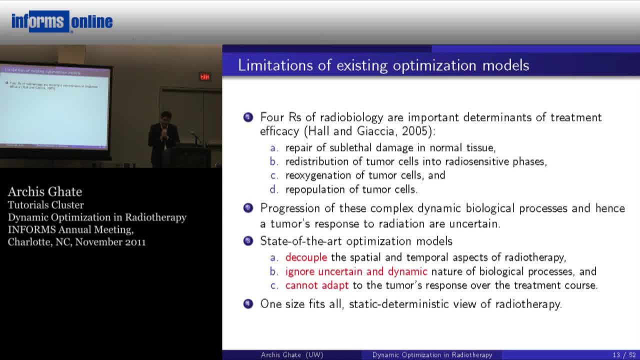 actually there are something called four R's of radiobiology, and so this is a bible of radiobiology. this is where I learned what little I know about radiobiology. but that book basically says that. so repair of subluxation, damage in normal tissue. so basically cell repair in normal tissue. so that's. 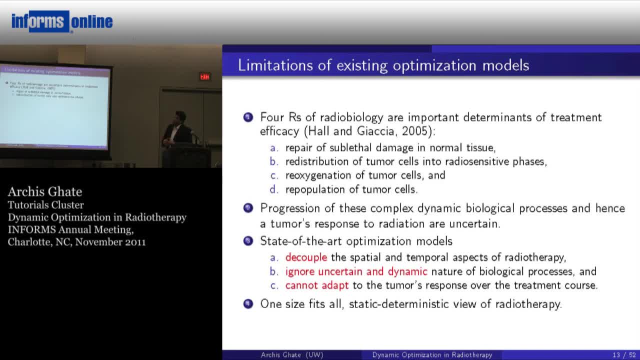 the first R, redistribution of tumor cells into radiosensitive phases. so cells lifecycle in different phases of that lifecycle are different in terms of radiosensitivity. okay, so tumor might be more radiosensitive in one phase of the cycle as compared to another. okay, so in a sense, what you want to do is really catch the tumor in the most. 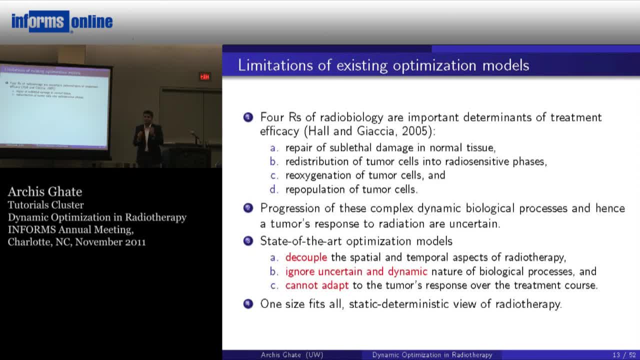 radiosensitive phase of the lifecycle, so that you will be able to kill the tumor with the least amount of dose in some sense right? so that's the second R, and the third R is actually reoxygenation, so oxygen content near the tumor actually becomes important in determining efficacy of treatment. 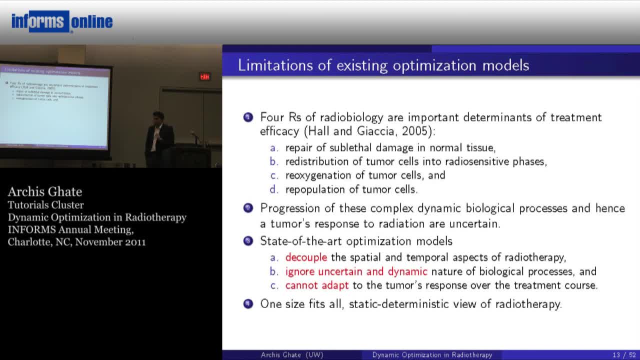 because if you have low oxygen near the tumor, that actually makes the tumor less radiosensitive, okay, and that's called hypoxia and there was a talk in fact yesterday about that in the evening session and I will talk about that a little bit later on also. but so oxygen content near 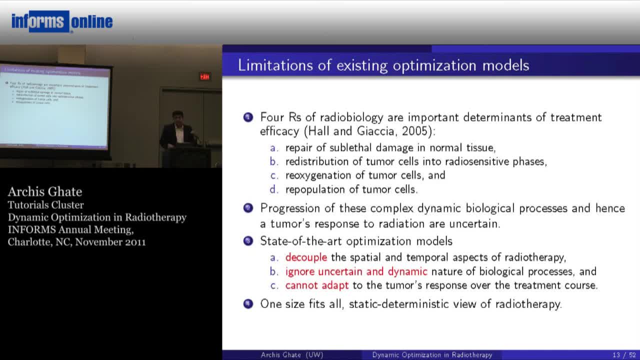 the tumor is also important. so that's the third R. and then repopulation, so tumor cells grow, and so on, so that's the fourth R. so these four things, basically, are going to determine the treatment efficacy and, as you can see, these are extremely complex biological processes that we don't really understand. 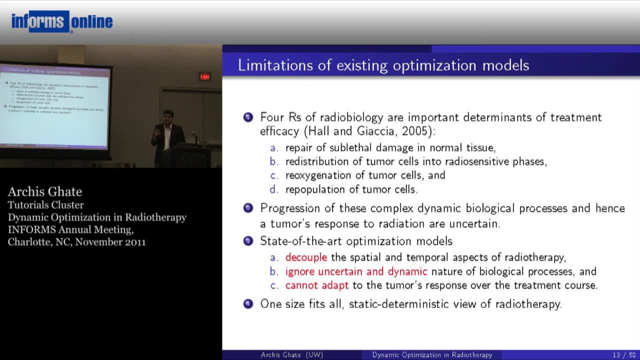 completely. people have tried and people are trying, so our understanding of this is improving, but these are still complex and, because of essentially insufficient information, there is a lot of uncertainty in how and whether we can model these things. okay, so what state of the art optimization models do? I just showed you very basic models, but essentially all variations of 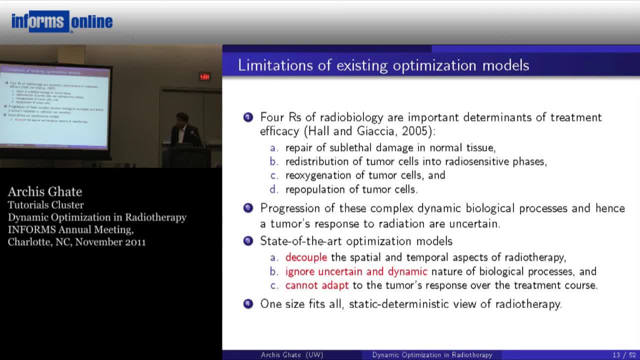 those models, or almost all variations of those models, I believe, decouple the space component, so the spatial component of the problem, with the temporal component of the problem, in the sense that, like I said, you first solve the spatial component of the problem and then break it up into equal dose. 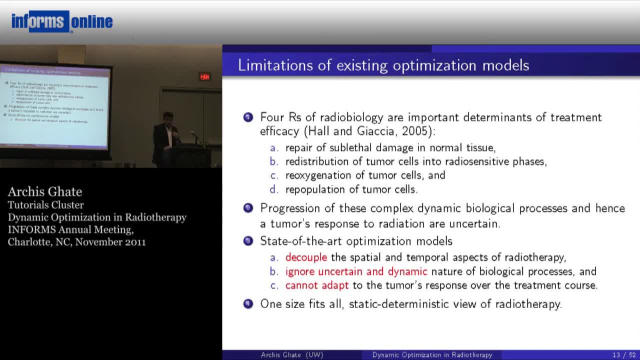 fractions, so essentially in some sense decoupling the two and in a sense you're ignoring uncertainty in response. so tumor response of how tumor will actually respond to treatment, how these things will progress in response to radiation treatment, and the uncertainty in that that is being ignored and because 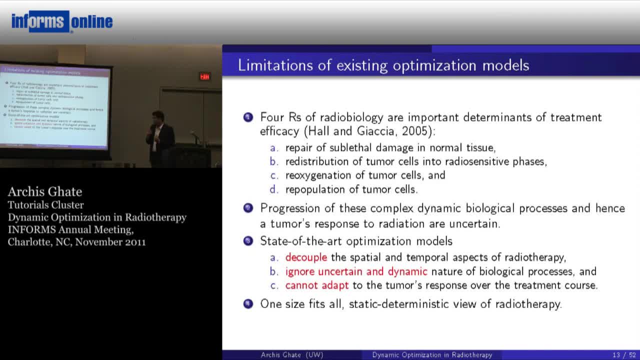 of that, the treatment is not really adaptive to how the tumour is responding or how these biological processes are happening over the course of the 5 to 9 week treatment. So in that sense the state of the art models are not adaptive. So let's keep these three things in mind and the way I view this is actually one size. 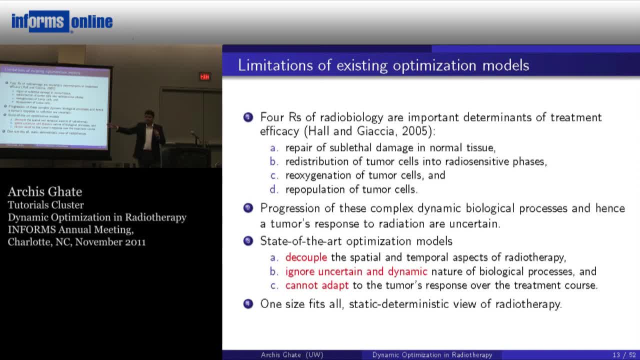 fits all. Remember I said 2 grape per fraction for 20 fractions. so you give that to a particular kind of tumour, let's say head and neck tumour or something like that. So I kind of personally view that as one size fits all, or in other words the static. 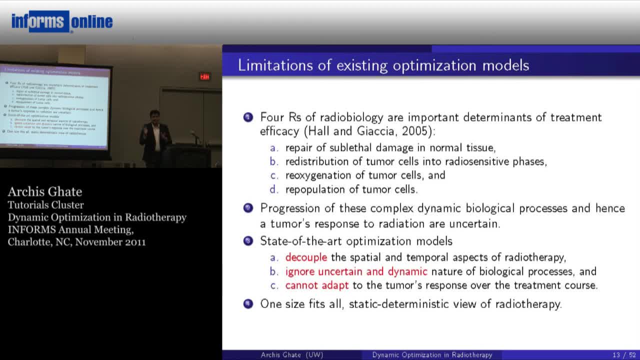 deterministic view of radiotherapy. Static deterministic meaning, like I said, I am ignoring uncertainty and I am solving the problem at the beginning. so one shot, I am solving the problem and then breaking the dose up into several fractions. So that is the static way, in my view, of thinking about this problem. 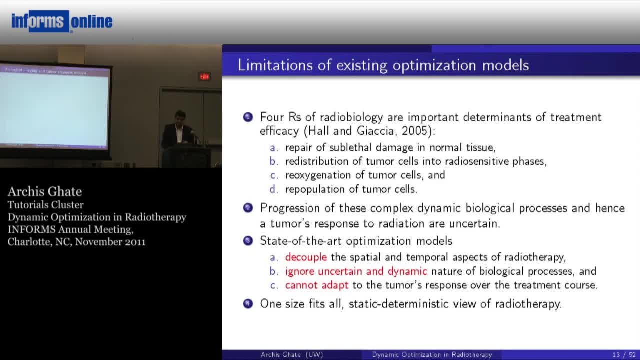 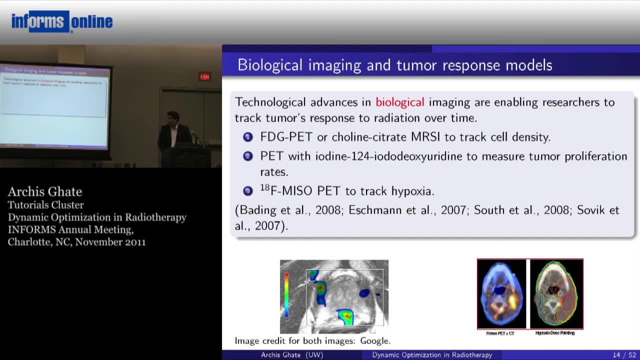 So can this be changed or is this changing? And the answer to that is actually yes, and there are 2 things that are at the heart of why that is happening. So the biggest issue or the biggest contributing factor to that change is technological improvements, basically. 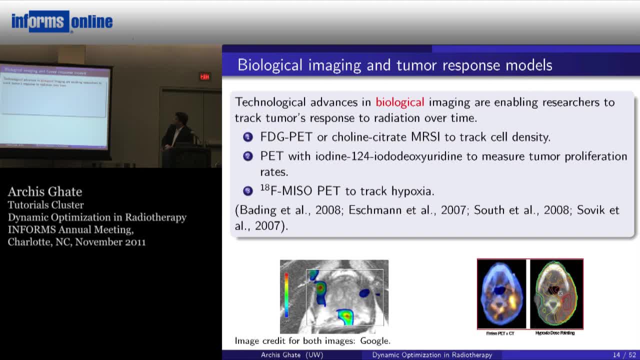 So there is something called biological imaging. So because of biological images, you can actually understand a lot more about the tumour's behaviour these days than you could a while ago. So these are names that I found in different books and papers and so on. 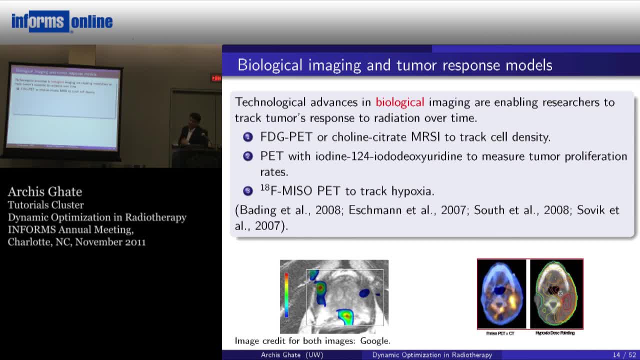 So FDG, PET, so positron emission technology, that is PET and FDG is basically fluorine tracer, or trace or tracer, or choline citrate, MRSI, so magnetic disturbance, spectroscopic imaging. Choline citrate is again another tracer, So these things can be used to track cell density and I actually have a picture, I believe, of 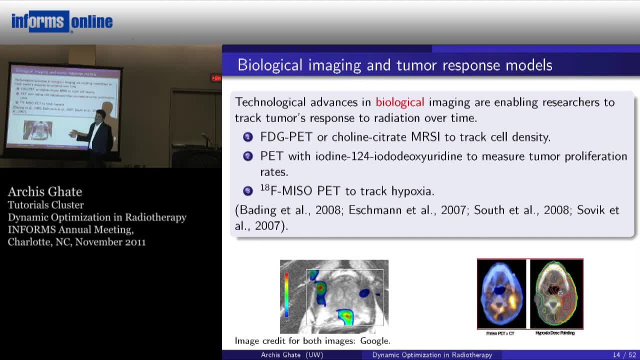 that that I found on Google. So this is in contrast with- remember, the earlier picture that I showed you was kind of similar to this. This is MRSI, which was an anatomical image, but this is MRSI with a choline citrate, I guess. 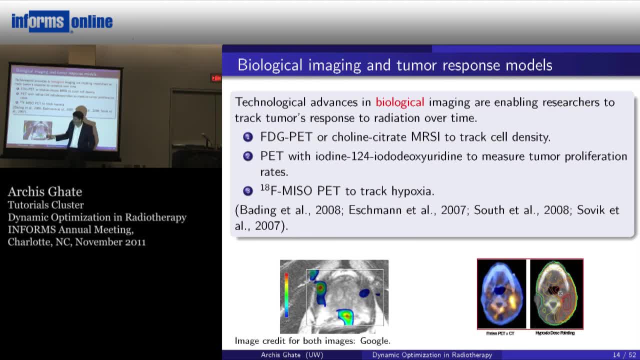 tracer, which basically in some sense tells you how much tumour density is there in different parts of the tumour, And it is quantitative, meaning that these colours so, blue means low, red means high, but in this picture that I found on Google there is also this scale that goes with it. 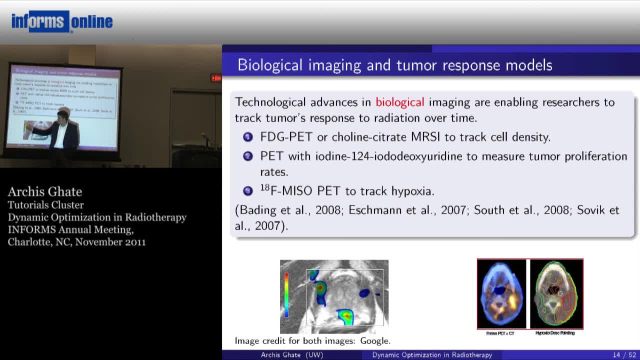 meaning that for every colour I have a number that goes with it. So there is a 4 point, something here versus a 0.01 there. So this is a quantitative information that I can get from this image about where the high density of the tumour is versus low density. 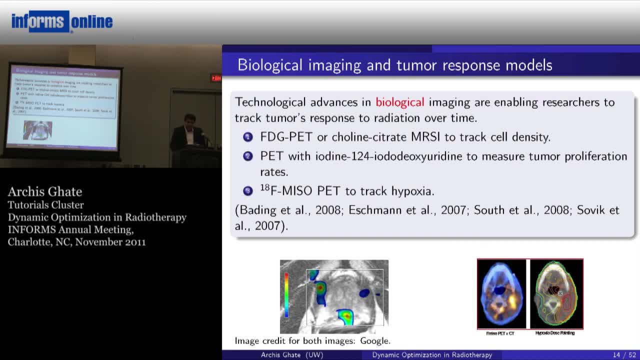 So that's one example. FDG PET also does something similar. I have other examples here. so now there is another kind of image with an iodine tracer which can tell you the rate at which the tumour is proliferating. So the tumour is growing in a particular region. 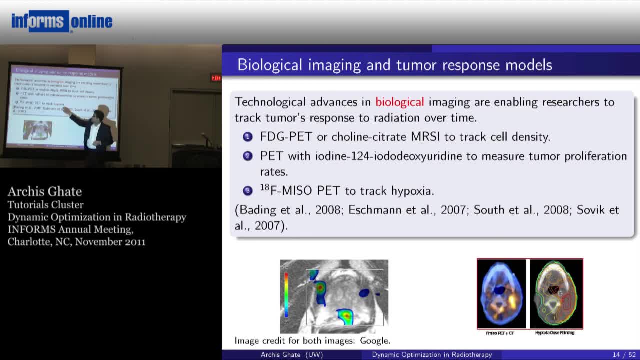 I mentioned hypoxia. I also mentioned another talk yesterday. So hypoxia means hypo oxygen, so less oxygen, so lack of oxygen near the tumour. So you can actually see where that is in this kind of a biological image. And this is another thing I found on Google. 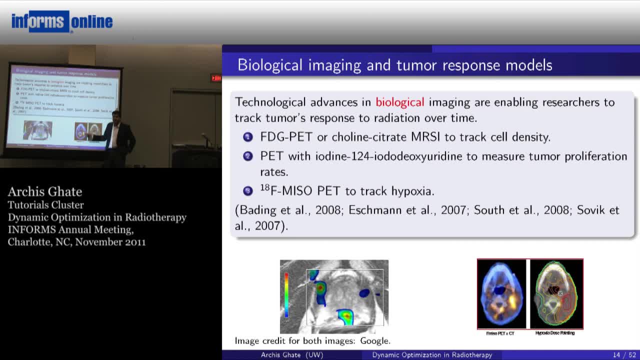 So this is actually this yellow thing here. it basically lights up. okay, so the image lights up in some sense where there is hypoxia, so less oxygen in this portion. So how intuitively, How can I use this kind of an- you know, this kind of an image? 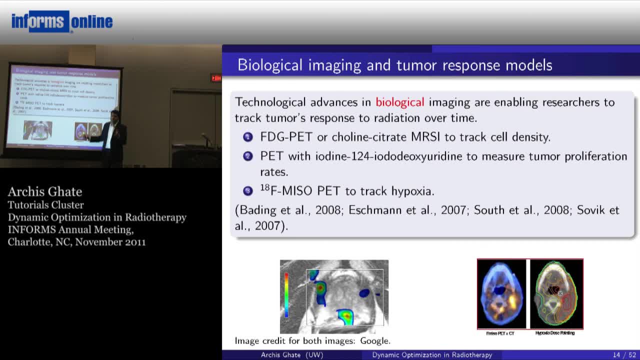 Of course, because I know that there is less oxygen here. I will somehow try to come up with a dose prescription, for instance, that gives higher prescription dose to this region of the tumour right perhaps, as compared to other regions of the tumour right. And of course you don't want to give a very high prescription everywhere because that 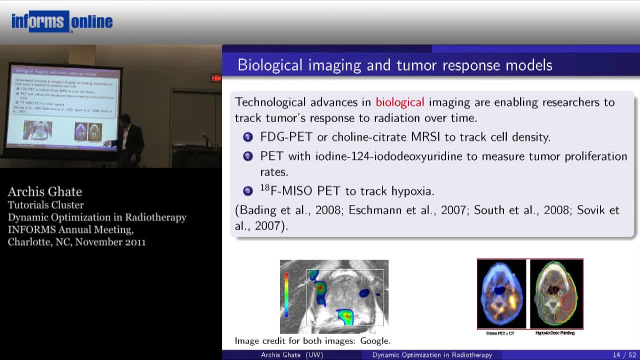 might be too harmful to the OER right. So that's called dose painting and this also is you know from the same place in Google. Basically, it's trying to show that you know, if you have a very high dosing rate, you can give a very high dosing rate to the OER right. 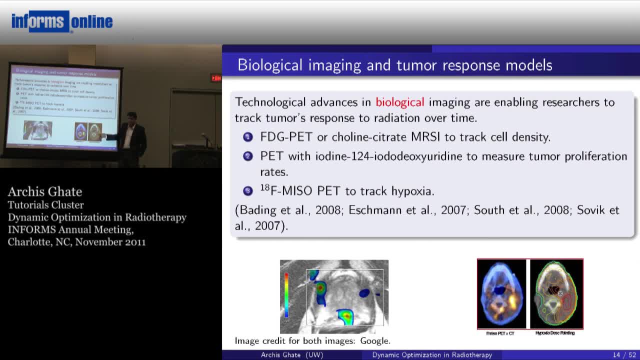 So that's called dose painting and this also is, you know, from the same place in Google, So that's called the OER, right? So this is a very high dosing rate that I can. so these are red circles, so I saw those curves. so I am giving basically a very high radiation in the place where I am seeing hypoxia. 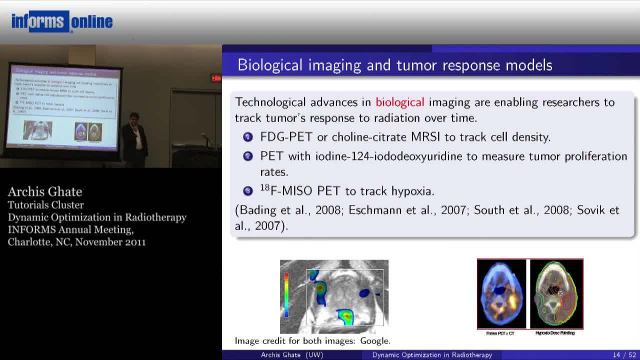 okay, Did you have a question? Yeah, so how stable is that hypoxia status? Hypoxia is So like. so if I take a PET scan and I see whatever that is, Yeah, whatever that is, yeah, Yeah, and you see that yellow spot is, is it presumably going to be there for a while? 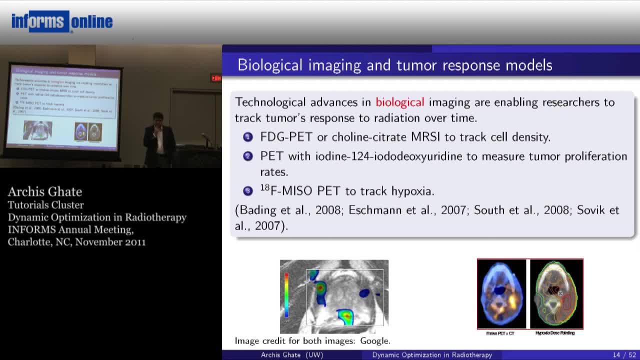 No, it's very unstable in fact, it's very dynamic in fact. So you know what I mean. So you have a very high dosing rate, Yeah, So how stable is that? hypoxia status? So if I take a PET scan and I see, whatever that is, 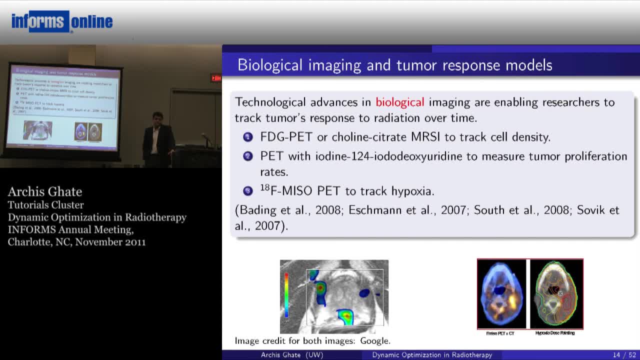 Yeah, and you see that yellow spot is. is it presumably going to be there for a while? No, it's very unstable, in fact, it's very dynamic, in fact. So this, So what kind of science are you talking about? So it can change. so, over the course of the treatment, this does actually change, so so 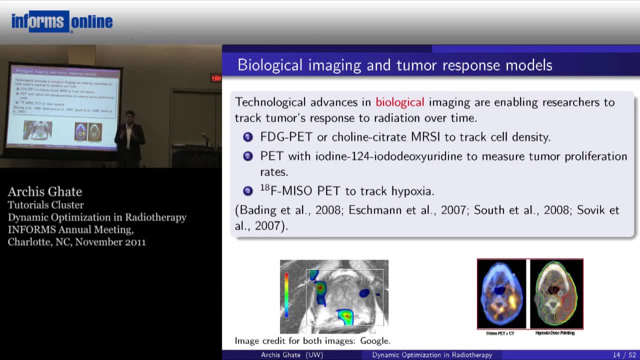 as you see, my research and what I'm going to try and do is somehow try to model how this may change, or use what other people may have done in radiobiology as to how this will change. So I'm going to incorporate that into my model so that I can treat dynamically accordingly. 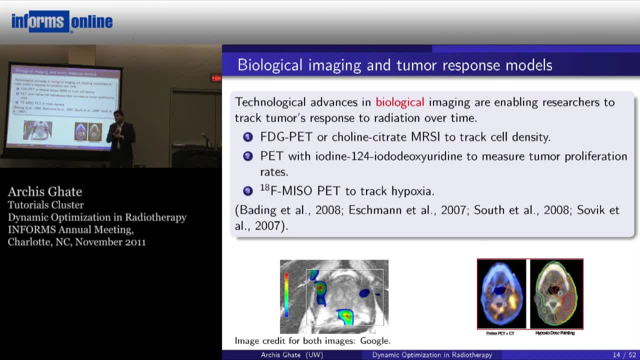 Right, Okay, Excuse me, I think the PET identified is not hypoxia area. It seems like BG to identify most metabolic activities. Right, I mean different. with different kinds of tracers I think you can identify different things. So this particular tracer, I believe, can identify hypoxia. 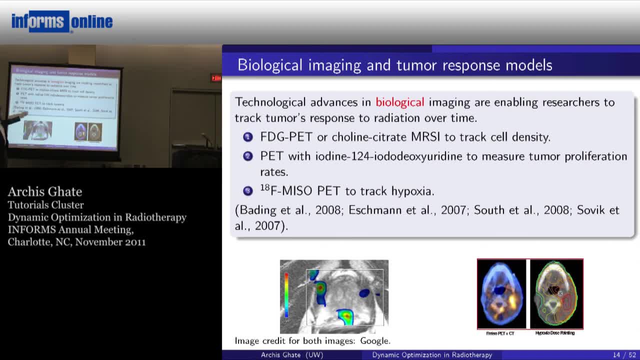 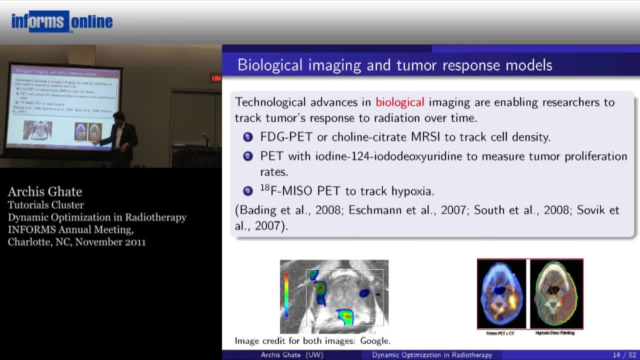 I think this is a picture that talked about hypoxia. So I mean, this is not something I wrote, This is something I found, So I'm not an imaging expert, but there are images out there which will show you where there is higher levels of hypoxia versus lower levels of hypoxia, or different proliferation. 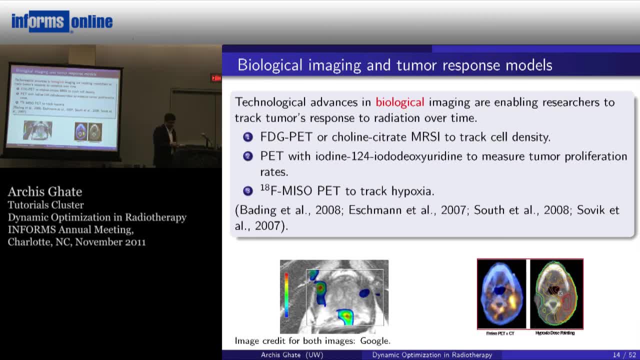 rates or metabolic activity and so on. Okay, Using different kinds of tracers, and I think you also had a similar picture in your talk yesterday for hypoxia. yeah, so this is dynamic, but this is just one picture, so one shot, okay. so so that's one part of you know the two pieces on this slide. so biological imaging. 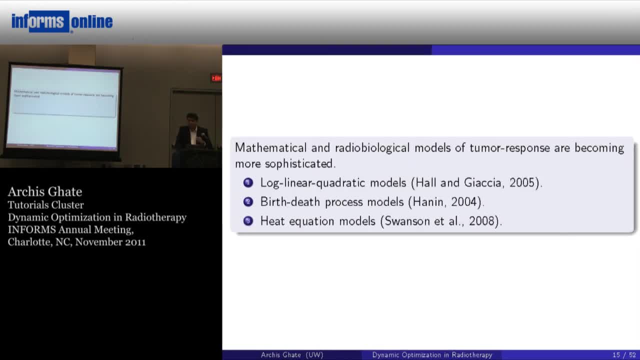 and tumor response models. so the second part is that tumor response models are also becoming kind of sophisticated. so the most classic, so the most well-known one is log linear quadratic, and that's also in that book that i mentioned earlier, and i will talk about that in that model in detail later on. but there are other more sophisticated. 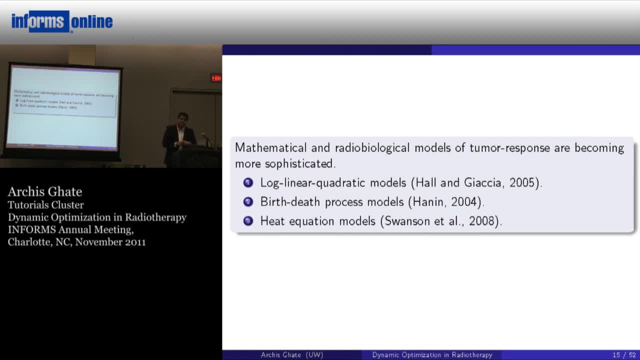 models that i also found. so there is. there are birth death process models of tumors. so basically you model the tumor's behavior as a birth and death process, for you know how the cells are going to die and you know there's cell birth and so on. there are also heat equation types of models. 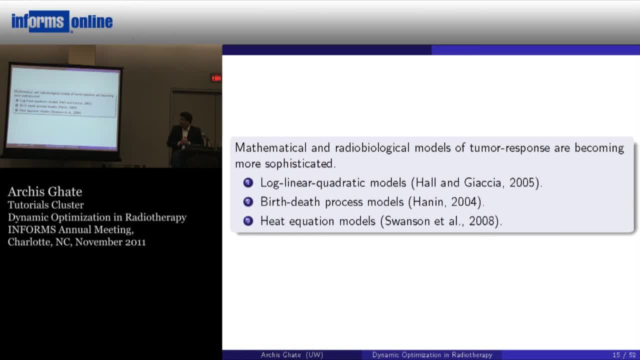 so julie swanson is actually at university of washington- and heat, heat equation. so basically that is a diffusion equation which talks about how the tumor will actually grow okay in the patient's body. so that's another point. so it's basically a different, partial, differential equation. so those kinds of models. 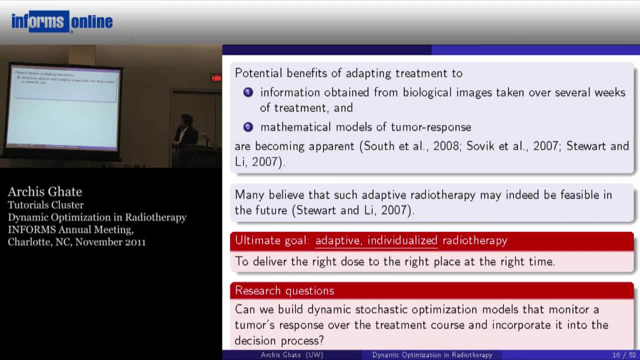 are also becoming available. so the idea is: are there benefits to potentially adapting treatment to information that you can obtain from these kinds of images over several weeks of treatment, so perhaps by taking multiple images over the 50 days of treatment, for instance, right, rather than just one. and can you combine those things also with mathematical models of tumor response? 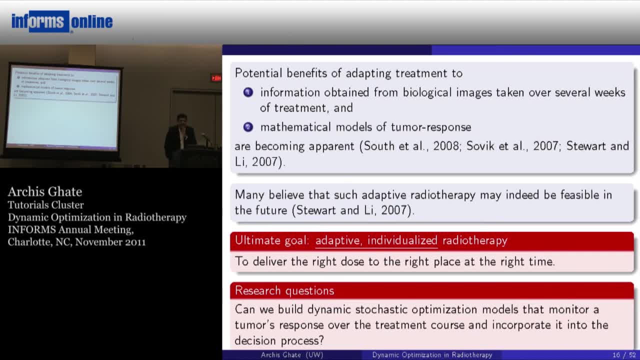 and there is clinical work in this area. so people are doing this clinically a little bit. so here are some papers where there are clinical examples of how people have taken these images and tried to use information in these images or to come up with treatment plans. okay, that can change over time, for instance, so somewhat adaptive. 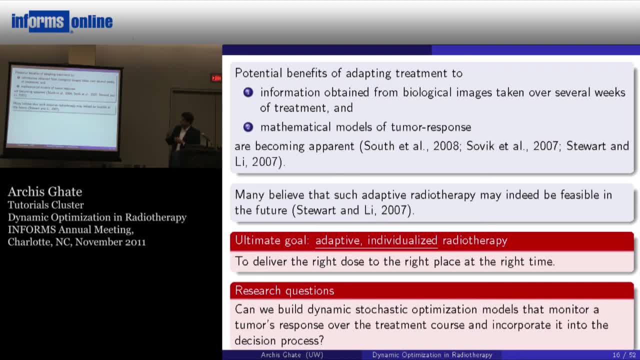 and in fact, many believe so. this is a paper in medical physics, so many doctors and others believe that this will be actually not only feasible but in fact common in the future. okay, so use of models, along with more sophisticated- you know- advanced imaging to come up with adaptive treatment plans. 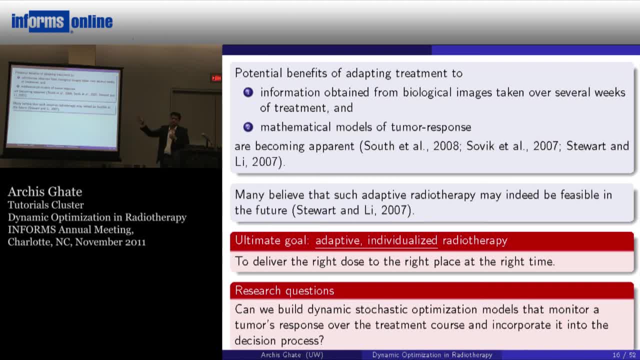 will actually be common in the future. so there's something called a 2020 vision for radiotherapy. so what's going to happen over the next 20 years, and so on? so there are papers like that where people talk about this being a possibility. okay, so the ultimate goal. 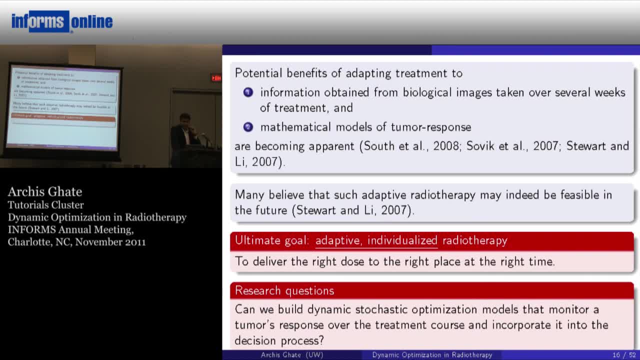 i think, in my view, would be to come up with adaptive and completely individualized radio therapy. so right now, the way i think about these problems is: you know, the idea is to deliver the right amount of dose at the right place, right? so all the pictures, everything i 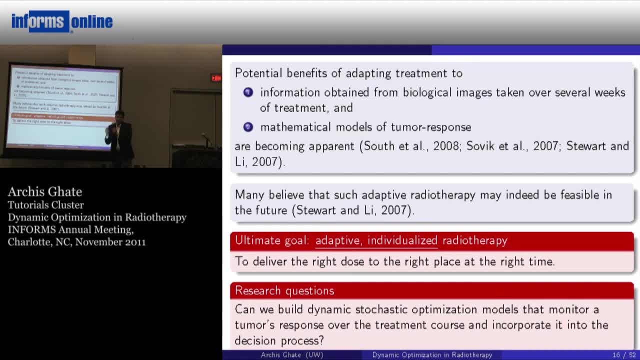 talked about is right amount of those at the right location, but i think the goal would be that you could add at the right time to this: okay, so, the right amount of those at the right place at the right time. okay, so that could be an ultimate goal and that is something i would view as 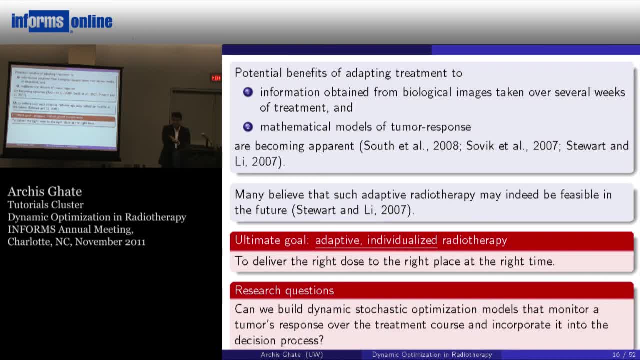 individualized radiotherapy right, really tailored to what is happening inside the patient's body over time? and i am not a biologist. so as an operations research person, my research question or my interest is really: can i come up with some kind of stochastic dynamic optimization models can start thinking about in the future getting here, okay, so as i said, the models that are more 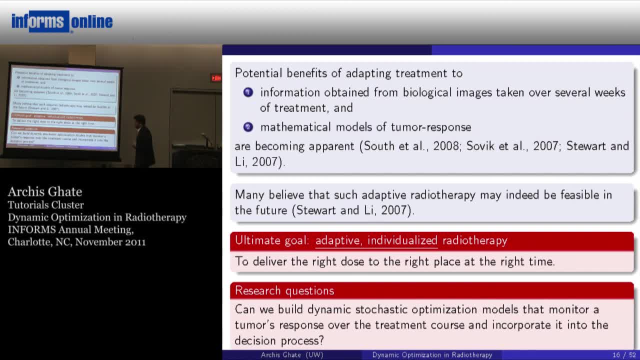 common are static deterministic. so my research question is actually: can i make you know, can i build dynamic stochastic optimization models that will eventually perhaps help us get here? okay, we are long way from there, but in my tutorial today i'm going to show you some basic, simple models that we will build to start thinking about doing that. okay, 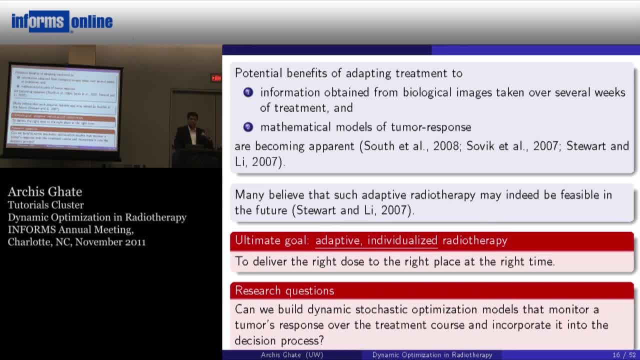 so it's the overall idea, overall framework, roughly clear as to where the field is and where i'm trying to go with these toy models that i'm going to show you today. okay, so i'm going to show you two attempts that we did for building dynamic stochastic models. okay, so the first attempt: 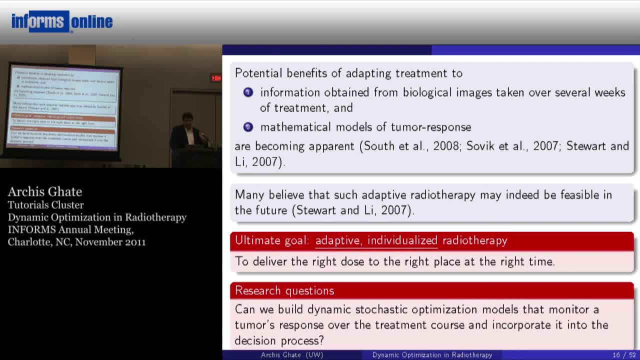 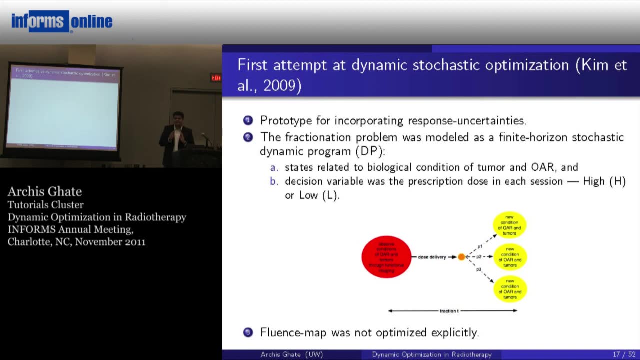 is just one or two slides. there is not much in it, so that will be slide 18. so the rest of the talk is about the second attempt that we did at building these kinds of stochastic dynamic models. so the first attempt. we said, okay, so let's step back and make this as simple as toy as possible. 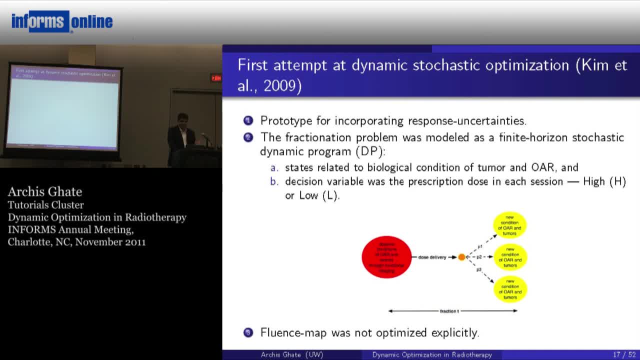 okay, so at the heart of this, what is there at the heart of this? you basically somehow so: operations, research, people. you basically somehow want to- let's think about it this way- take a picture, get the information that is there in the picture, right, have some kind of a model that will tell me. 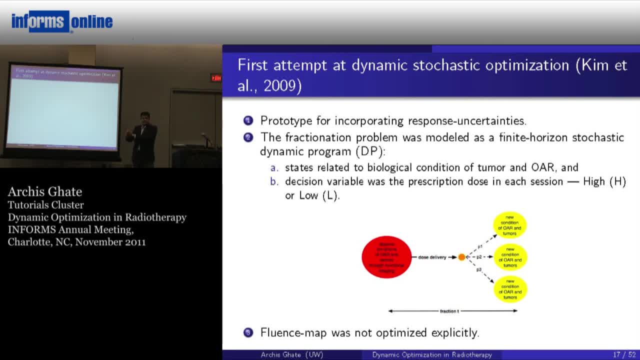 how the next picture will be essentially right, some kind of a probabilistic model right, and then keep doing that over the course of the treatment and somehow build some kind of an optimization model that will optimize my treatment or treatment efficacy right, using this basic, very simple idea. 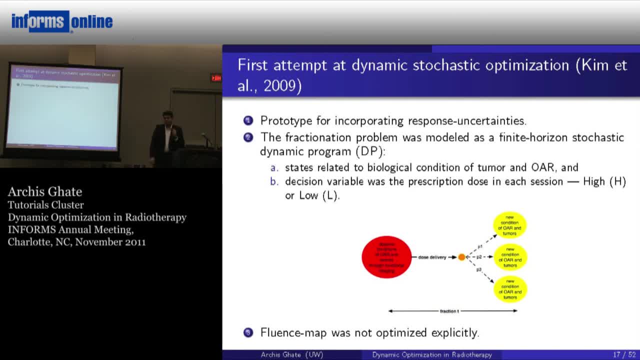 okay, so we tried to do that. so we built the easiest possible, the simplest possible product prototype that we could build, which had only these two features essentially. so basically a finite horizon problem. okay, finite horizon because typically you know the treatment will be 30 days, right, patient will come back 30 times. so finite horizon problem. 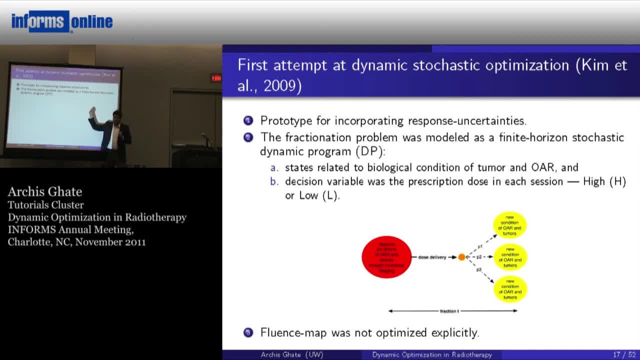 you're all in operations research. so stochastic dynamic program, right? so very simple, stochastic dynamic program where you have only two things, so you'll have states that relate to the condition of the tumor and the condition of the organ at risk. okay, so at a very high abstract. 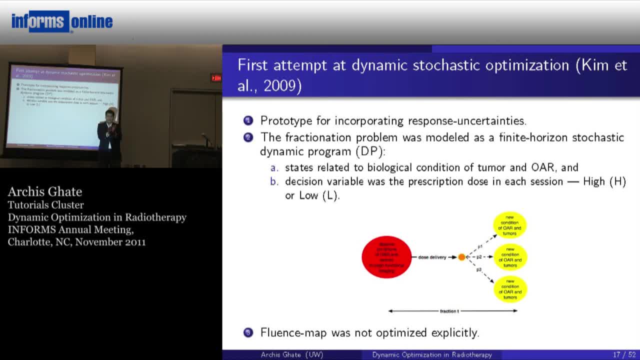 level. i'm going to take a picture that tells me the condition of the tumor, the condition of the organ at risk, right, and i'm going to have some kind of a probabilistic model for how this condition is going to evolve over time. right, i'm going to use that to build a stochastic dynamic program. 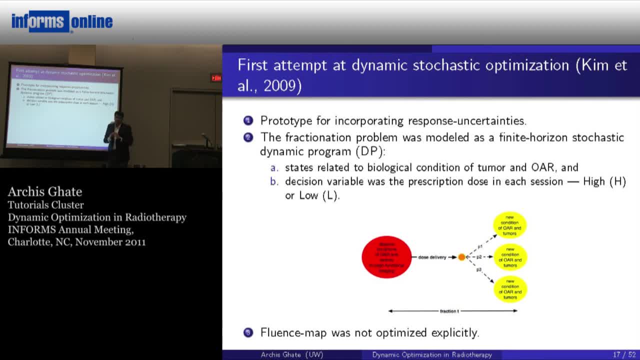 okay, and in that really simple stochastic dynamic program i'm going to have a very simple decision variable and i'm going to call that prescription dose and i'm going to only allow for two values: high or low. okay, so, very high dose or very, let's say, low dose. 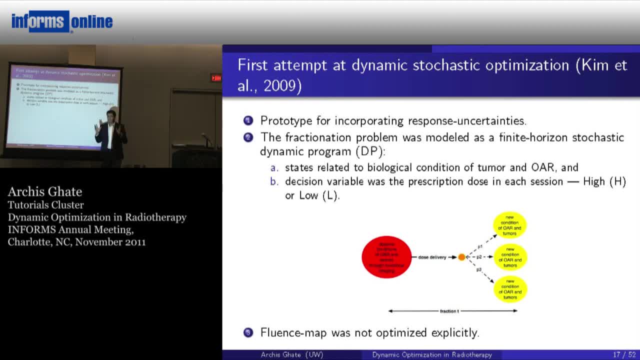 okay, and the probabilistic model, as you can imagine, is going to depend on the dose, right. so if I give high dose, right, the image will change probabilistically in a certain way, versus if I give a low dose, the image will change or the condition will change probabilistically. 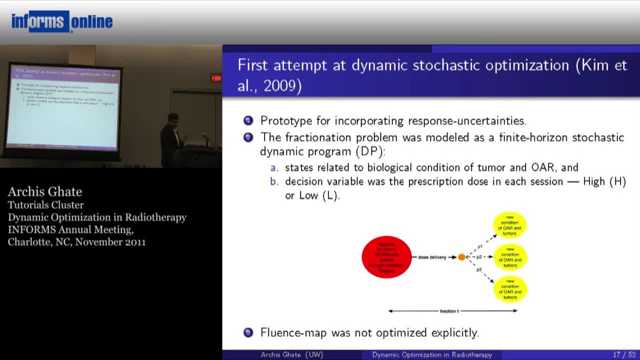 in a certain different way. right, so that's going to be my really simple prototype and this is the idea. basically, you know, this is I'm showing one fraction here, so one treatment session: observe conditions of OER and tumors through biological or functional imaging. right, give your. 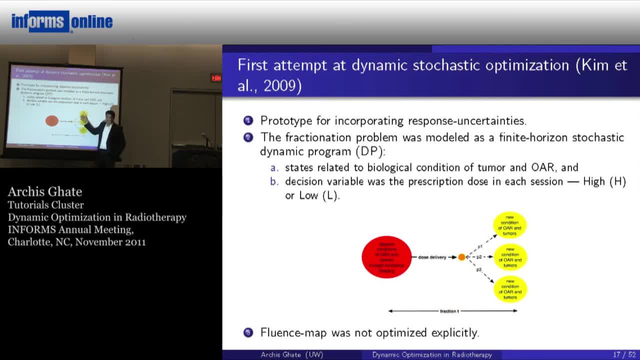 dose. the system will evolve probabilistically right to different states- this state, this state with certain probability, this state with certain probability, and so on, and keep doing this right and use this idea to somehow build a simple stochastic dynamic program. okay, so that was our first paper and I was actually in a sense surprised that this paper was accepted, because 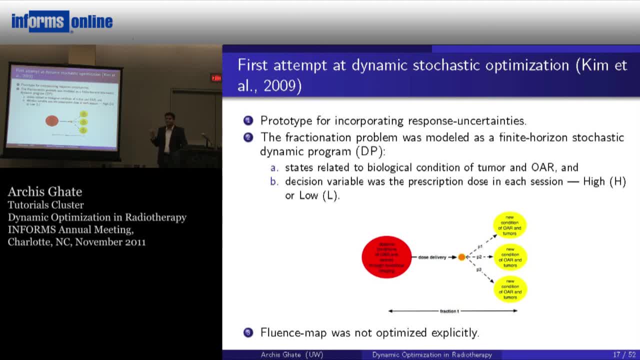 this is not practical. okay, this is really really, really simple and this was actually accepted in a medicine journal. so physics in medicine and biology, and I think the reason was that I think the idea was interesting because I had not seen stochastic dynamic programs for this kind of. 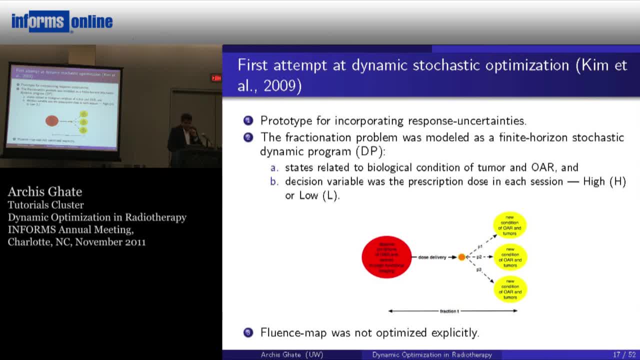 context before. okay, in particular, in this really simple prototype, there was no fluence map optimization whatsoever. okay, meaning that essentially, you can think about it like this: I'm still actually decoupling the temporal and the spatial component of the problem in some sense, but I'm still trying to incorporate uncertainty. so am I decoupling the two? what I'm thinking? 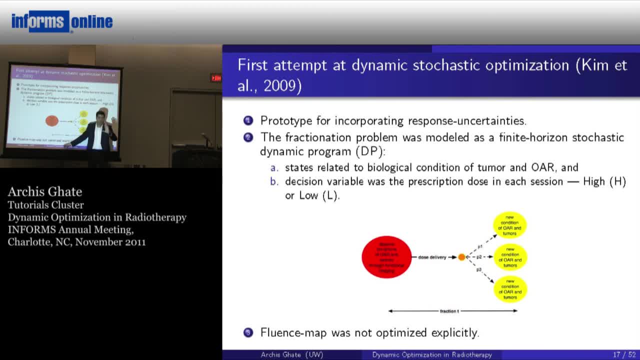 about- and we actually did not do this in the paper, but we wrote it in the text of the paper- that the idea could be that I use this lower high dose right as my prescription dose and we solve a fluence map optimization problem in every treatment session, right in the most. 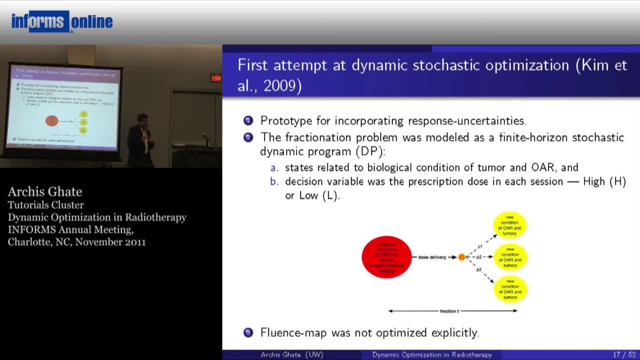 extreme case, right. so in that sense we still kind of have to think about this problem and we kind of decoupled the two okay, but did try to incorporate uncertainty okay. and then I'm not going to show you the details of that particular paper, I'm going to show you the second attempt. 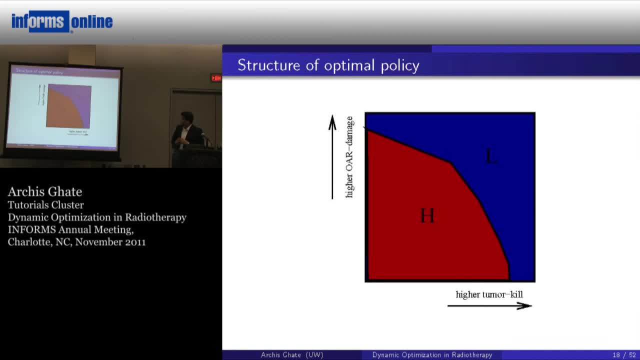 but I'm going to only show you one picture, and that is actually this picture. so, in the paper, what we did was a really simple model where I said: okay, let's have an ordered set of states for my tumor- ordered, meaning I can draw a picture like this: 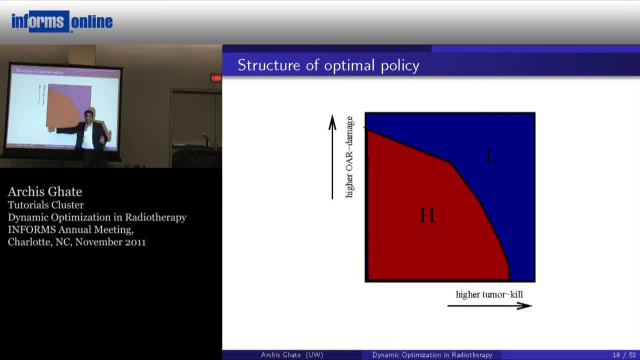 where on this left corner there is less tumor kill and on the right corner there is high tumor kill right. so think about it, as most of the tumor is dead here right versus none of the tumor is dead there, make sense. so I can order states like that and that is actually not uncommon in medicine. 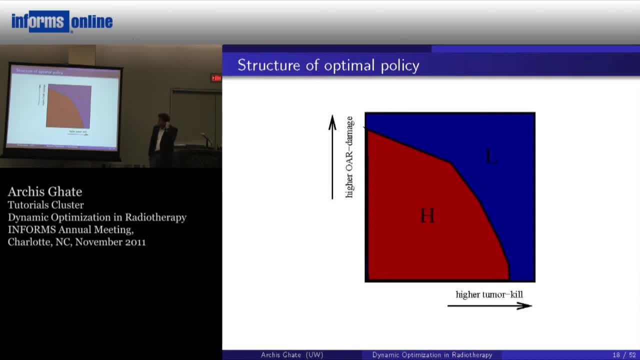 okay, there are other papers by Andrew Schaefer's group and other groups where they talk about ordered health states and use that in the context of stochastic dynamic program. okay, it's only that this was used, as far as I know, for the first time in the radiotherapy context. 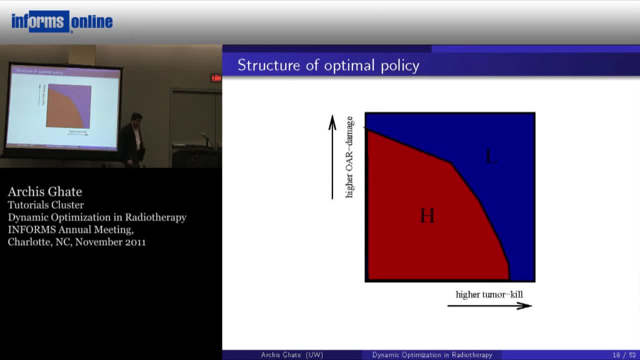 okay, so that's the x-axis, and the same idea for my y-axis, and this picture just gives you some basic intuition about the structure of the optimal policy that we observe in our paper. and let's see why this is intuitive. so, remember, I had only two dose levels: high or low, right? so the 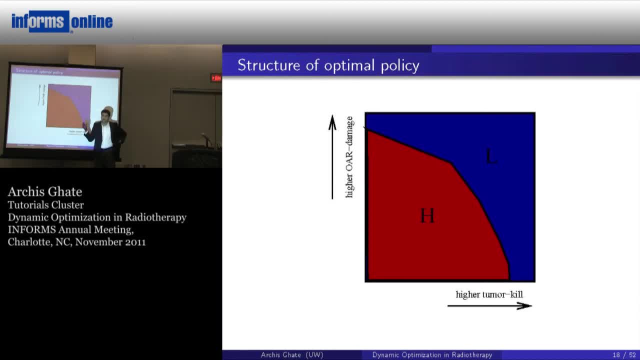 dose is high in this region. so there is a region where the dose is high and there is an envelope like this one, and then there is a region where the dose is low. okay, and that is intuitive why? because if you take any fixed level of OAR damage right, so let's say this level, right, the dose is high, high, high once. 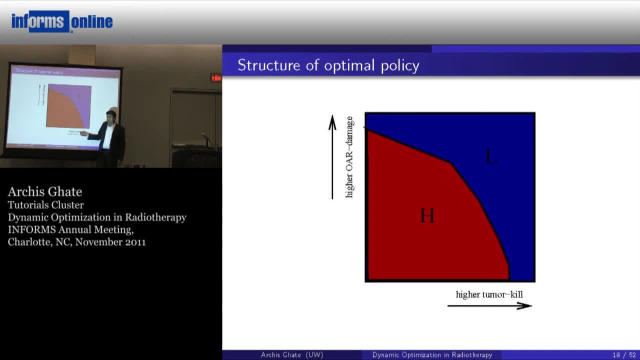 you cross a certain threshold, right, sufficient tumor has already been killed, right, because the tumor cell kill is higher this way. so sufficient tumor has already been killed. so then there is no point in giving high dose anymore, because you are in some sense unnecessarily damaging those OAR, right? so the dose actually drops after that threshold to a low value. makes sense going that. 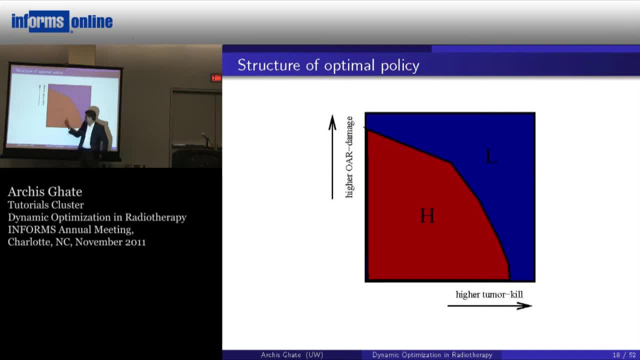 way and the same idea. you can think of it going this way because if you're going this way, that tumor cell kill is constant, right, but OAR damage increases. so once you cross a threshold you don't want to give high dose, so the dose actually drops after that threshold. okay, so that's basically. 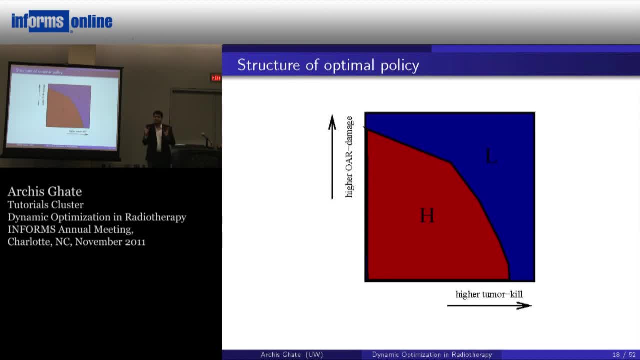 the structure of the optimal policy that we empirically observe, empirically meaningly, in the examples that we constructed. okay, none of this is treating real patients or anything like that, but the examples that we constructed. we have tried hard to prove right that this is actually optimal. okay, but we have been unsuccessful. so if you are interested, please, 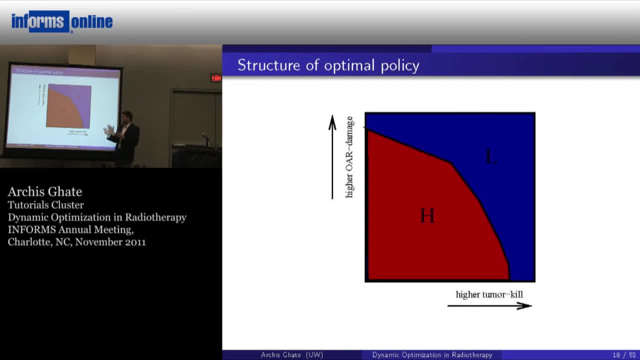 take a look at my paper and see if there is a way to prove that this kind of a structure will be optimal. okay, there are standard ways for doing these proofs, but the proof is not working. okay, that's a very interesting problem, i think. but okay, there is a question, i think. 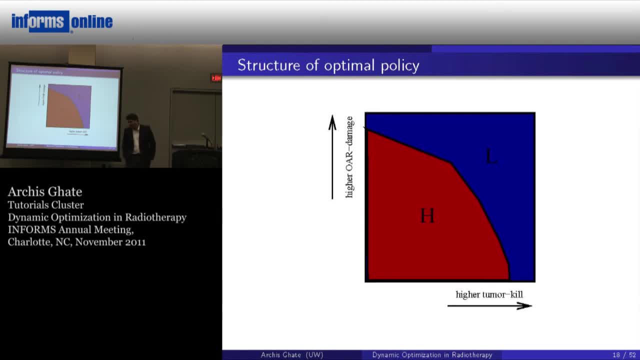 there is a question in the chat: so how many, how many states do you assume for tumor? yeah, so we don't need to assume a number. the only thing we assume that it was finite, so discretized, so some finite integer interval. basically, that's all we assume and that finiteness is just so that my 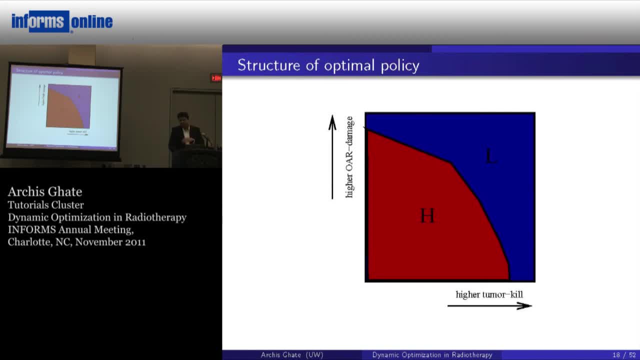 stochastic dp right is tractable and so on. yeah, in fact. so in my second attempt, right. so the remainder of the talk, my state space, is actually going to become continuous. the answer is actually uncountable. okay, but this very simple first prototype, it was finite, okay. 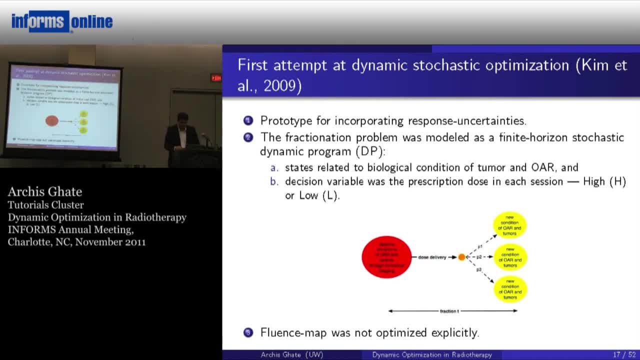 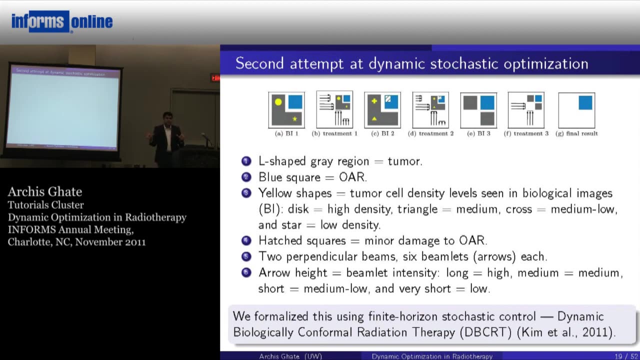 so okay, so that's my first attempt. this is a 2009 paper. if you want it, i can give it to you. you can easily find it. it's in the pmb. so let's actually go to what we really are trying going closer, or to what we really want to do. we don't want to decouple the two problems, right, so we? 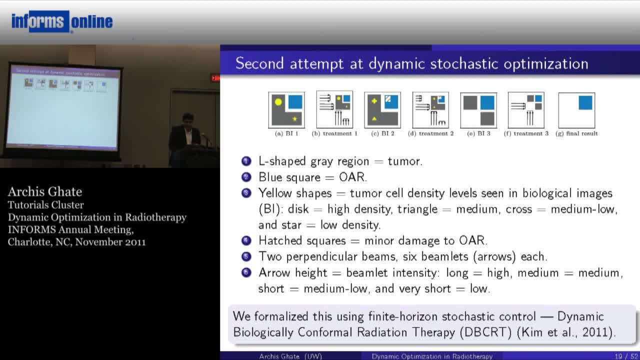 want to do the whole thing, uh, together, and that's our first attempt, so that's my first attempt, so i'm going to do our second attempt. so let's look at that, uh. so the idea here is basically, i'm just showing simple picture here, uh, so i have the gray region l shape as my tumor, the green, uh, the blue. 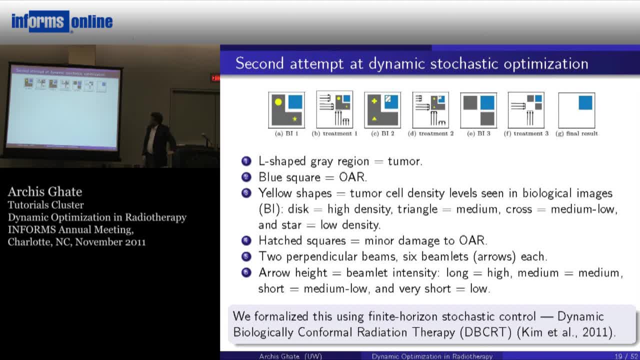 square is actually my organ at risk. so that's, that's my oar, uh, and the yellow shapes that i'm showing basically, uh, relate to what density i have in the tumor. okay, so, for example here, so yellow shapes, tumor density levels, so i'm just showing you a picture of my um, what i can imagine in my mind in this picture? some kind. 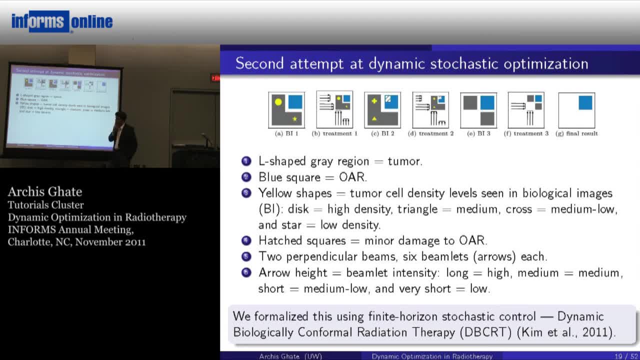 of a biological image. right, that will tell me, uh, what density. i have something like mrsi, for example, the pollen cited ratio that i showed earlier, but the disk is high density, triangle is medium, medium density and so on. okay, so the idea here is that you start the treatment, so you take this. 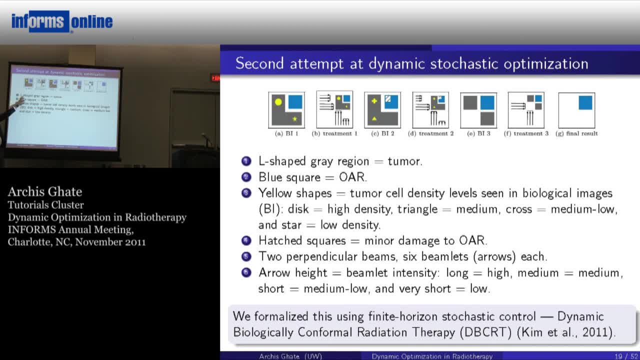 picture that shows you where the highest density is. that's my disc, and then then i have a star, which do is in my mind. I am trying to build again something like a stochastic dynamic program or stochastic control problem, where this picture tells me the state of the system, right and 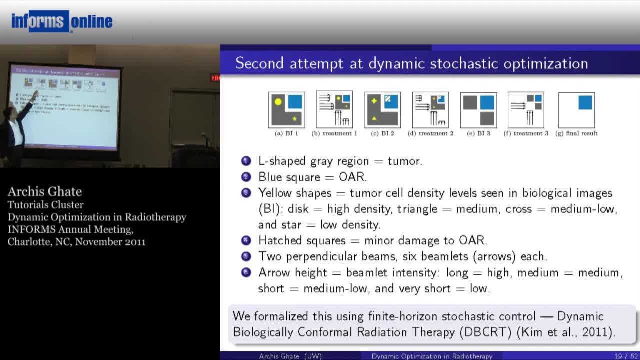 then I decide my treatment. so that's my treatment. so you can see the length of the arrows. length of the arrows, they basically tell me what the intensities are. so long arrow is high intensity and so on. so, if you think about it, these two so the northwest corner, so that's. 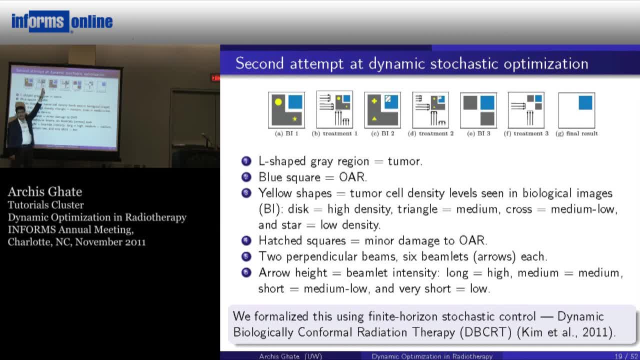 that at the top and this, okay, so those two are basically identical, right? so if I did not have the biological image, there is perfect symmetry between the two, okay. however, because I have the biological image and because it is telling me that the density is actually higher in the disk, 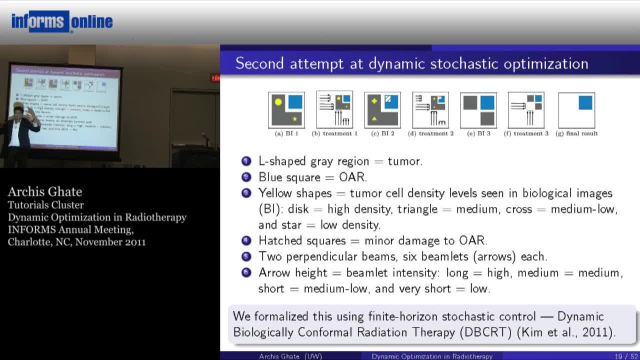 versus the star. I am actually using arrows of different lengths make sense, so that's kind of. I have that fluence map optimization problem in my mind there, so I'm using shorter arrow there and that is good. why is that good? because that is so. the OER is in direct beam. 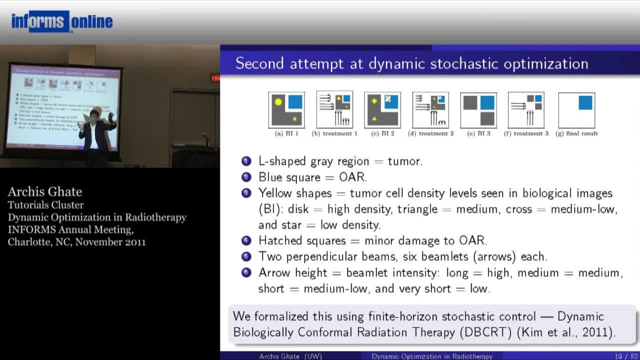 size view of those two right, so I don't want to give unnecessary dose or high intensity in that region. so then I mean I don't need to talk about the whole thing, but the idea is that you do something like this so that you can use the information that you are getting dynamically. 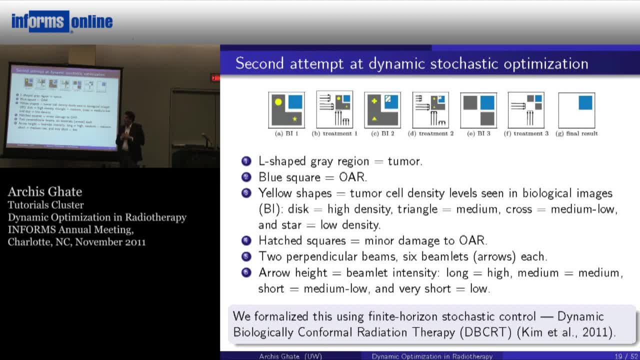 over time to adapt your treatment plans. okay, one important point that actually I think kind of gets lost in this picture is that this whole thing is interconnected right, meaning that I don't want to just take one picture and solve one problem that ends after that one period and then take another picture and solve a new problem. 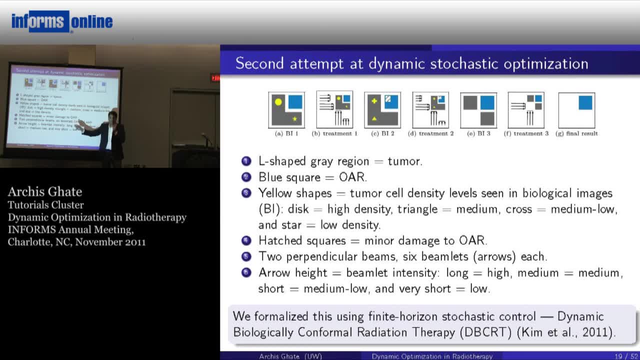 which is a one period problem, and then roll forward like that. that would be a simple way to solve this right or kind of heuristic to solve this. but that's not really what I want to do. I want to completely integrate this whole thing so that I have some kind of a stochastic. 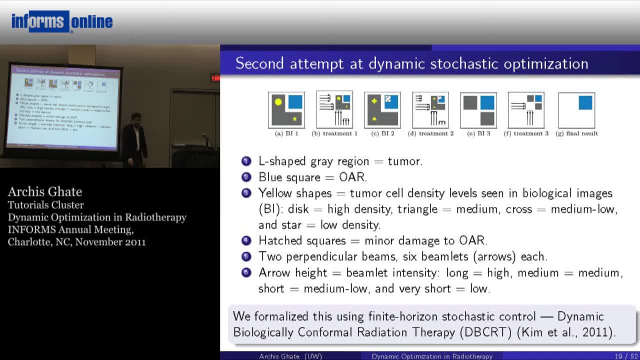 control stochastic nanome programming problem right, which has this temporal as well as spatial component embedded in it. okay, so that's the high level idea, and this is just intuitive idea that we had. so, from here to remember the red big goal that I showed you: adaptive, individualized. 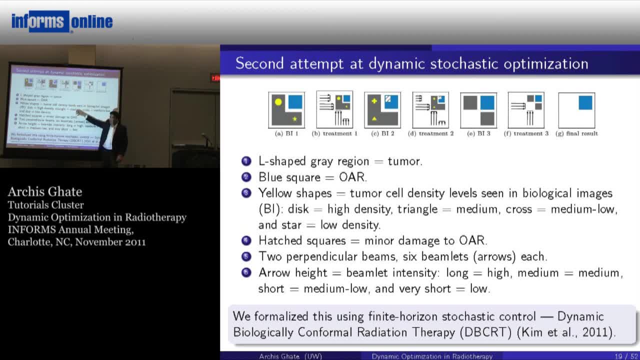 radiotherapy. so we are really far from that. but what we have started doing is we have started formalizing this in a finite horizon stochastic control formulation, right, starting to build at least some model that actually does this and solves some kind of a problem dynamically over time. okay, so that's our second paper in this area and this is actually in an OR type of. 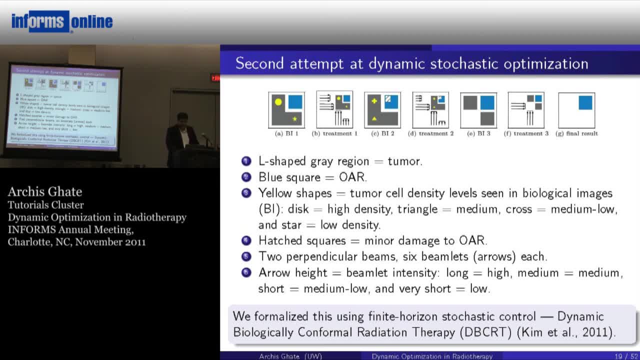 journal. so European journal of operations research has a issue on healthcare. that's where that paper is. so we call that dynamic biologically conformal radiation therapy. we have also called that adaptive biologically conformal radiation therapy. I think adaptive is more interesting than just the word dynamic. we have called it both, but in the paper we: 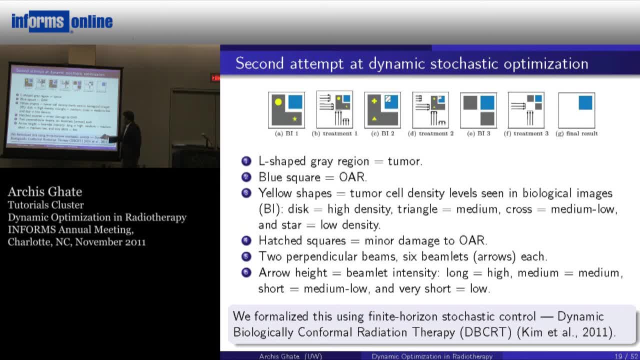 call it dynamic, biologically conformal radiation therapy. why do we call it dynamic, biologically conformal? because in our minds we have this idea that we are going to use biological images right, and we are going to come up with plans that conform to how these biological processes 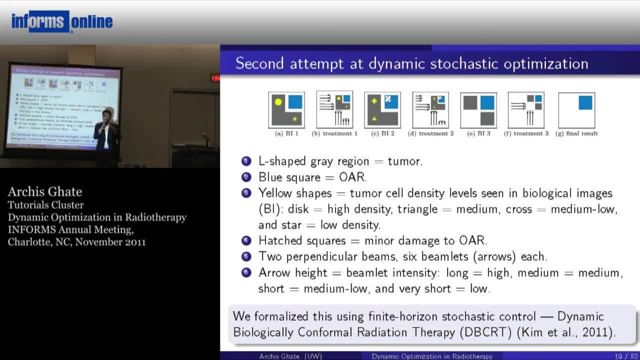 evolve over time right rather than just conforming to the shape of the tube when, for instance, right, so biologically conformal as opposed to physically conformal. okay, so that's the distinction we are basically trying to make in their okay. so now I'm going to start building. 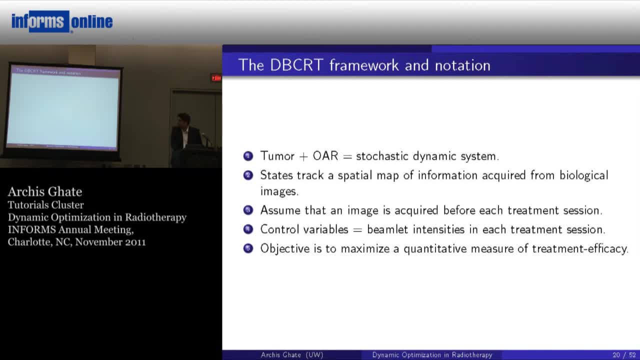 models on links, roughly 35 to 40 minutes. I'll show you some stochastic control formulations and some simple, heuristic ways to solve those problems. okay, so the basic tremor, as I said, is, you know, tumor plus over. I'm going to view that as a stochastic control formulation. right, and that is. 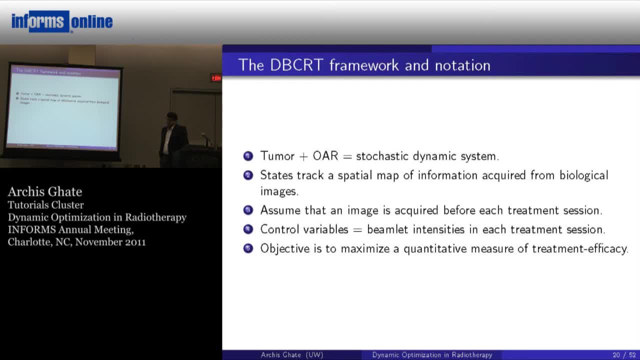 what we want to do when I am trying to solve, as simple as I have, a problem by drawing out about these problems, I can. so the basic framework, as I said, so in order to provide a basic framework, as I have Stochastic dynamic system, as I said before, the states will basically something that tracks. 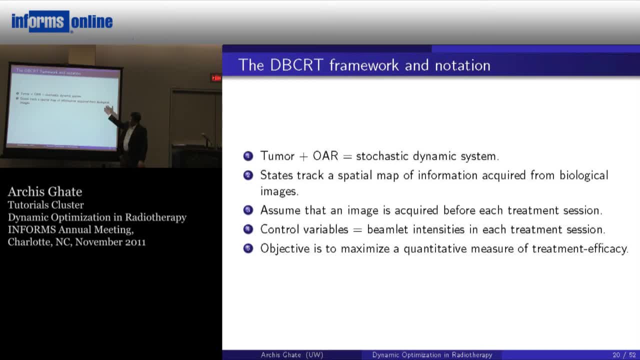 the spatial map of how this information that I acquired from biological images is changing over time. So, spatial map meaning going back to these pictures, right? So where is the high density right in terms of space and how is that changing over time? 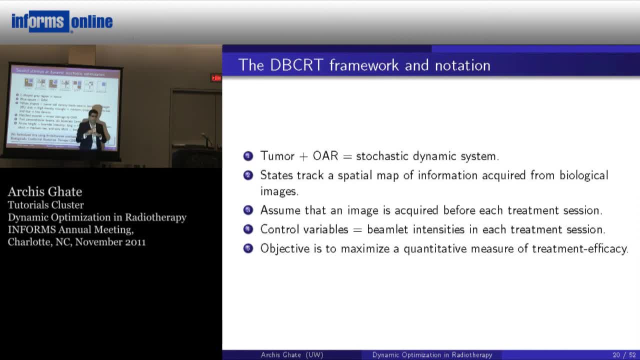 So that will somehow be incorporated in our state. okay, of this problem that I'm going to be dealing with And in the tutorial, at least except my last slide in the tutorial, everywhere I'm going to assume that I'm actually getting an image before every treatment session, okay. 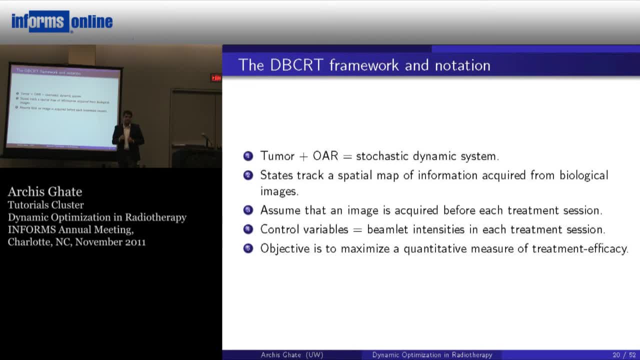 And that's essentially just so that my notation becomes simpler. okay, I can actually generalize this by saying that I take an image at every K sessions, or I don't have to decide beforehand when I'm going to take an image. I can come up with more general problems where that itself is a decision variable, and so 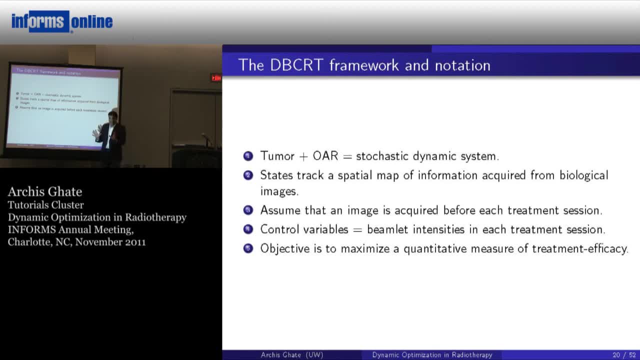 on So I can make this really sophisticated, in terms of modeling at least, but right now I'm just going to assume that I take an image every treatment session, just so that the notation is easy. Of course, there is a big issue here, meaning that this is going to have economic implications. 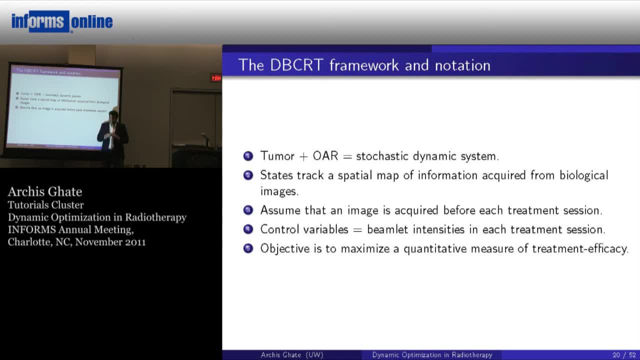 right because the images are expensive. inconvenience- right for the patient. right- taking an image every time the patient comes, essentially, and other clinical complications as well, right. So from a practical viewpoint, this is a big aspect, Okay. 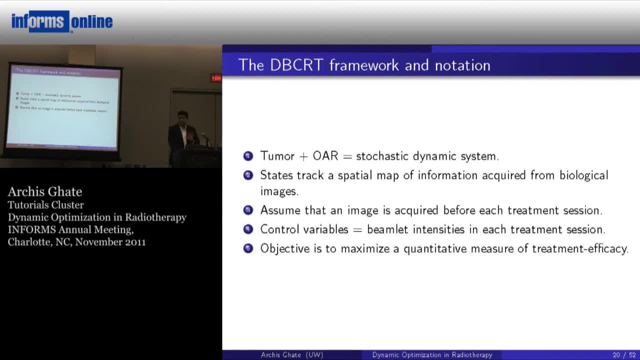 So I'm going to assume that this is a big assumption, but today I'm going to make that in terms of the math notation. Okay, At the end I'll show you a picture which tells you what is the effect of not taking an image in every session. 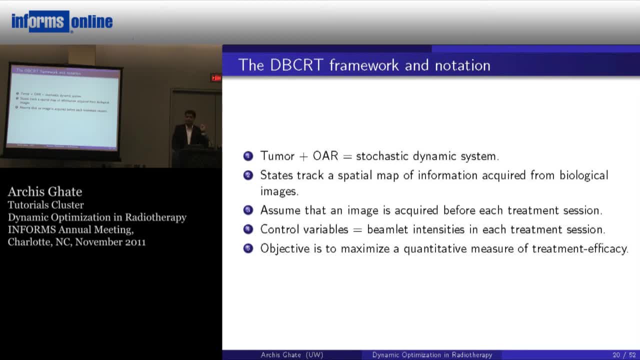 So I'm going to actually show you a picture of how much you're losing out by not taking images in every session. Okay, And that's how I'm going to basically close the talk later on And, as you can imagine, the control variables in the problem that I'm going to formulate. 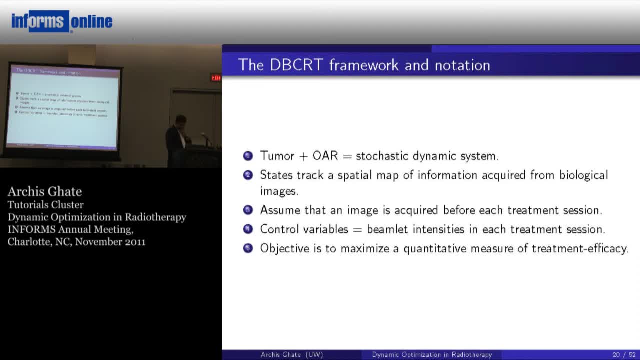 will be the Wimlet intensities, right? So the use will be my control variables, Hmm, And the objective is actually going to be the Wimlet intensities. Okay, And the objective is going to be something: some quantitative measure of treatment efficacy. 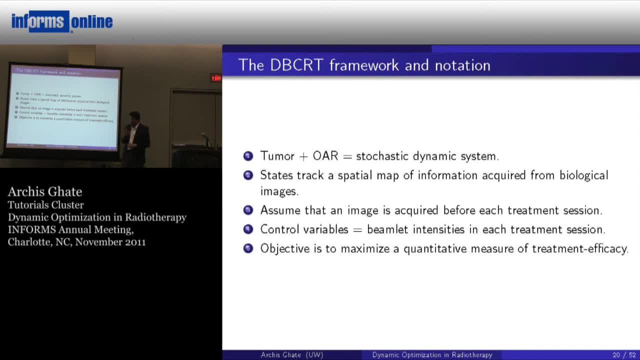 So I do this thing, do this dynamic treatment. So how good is this treatment? So I need some quantitative measure of that. So I'm going to actually have that in my objective. So that's the high-level framework. So let's start getting into notation and writing down some problems or models. 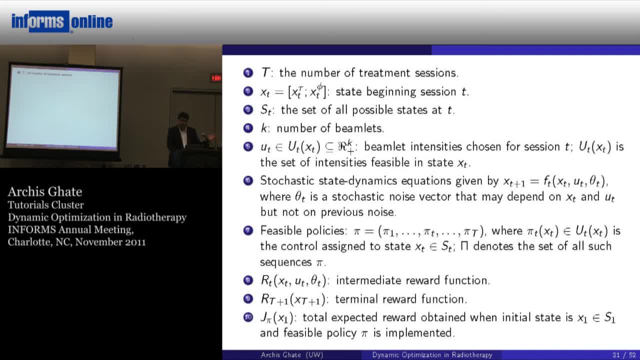 So T- I'm going to call that as the number of treatment sessions. We actually have a follow-on paper that we are working on where we don't even fix the T beforehand but we actually formulate an optimal stopping variation of this problem where I stop treatment when I think it is okay to stop treatment. 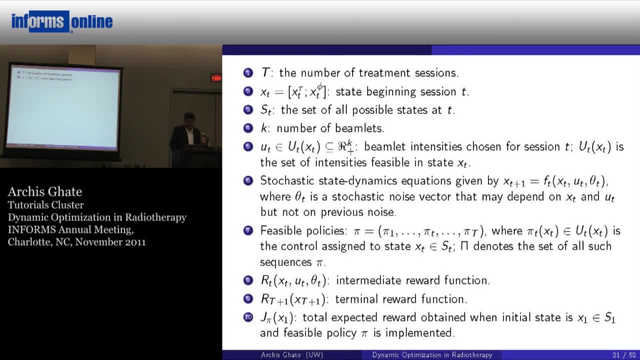 Okay, But right now I'm going to assume that I'm fixing capital T And then I'm going to have XT as my state at the beginning of the teeth treatment session And, I think, almost all my formulations. the state will have two major components: XT, tau. 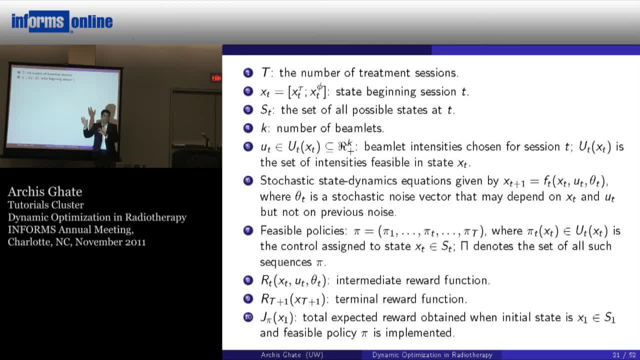 for the tumor information- Okay, And XT phi for the OER information- Okay. So it will have those two major components, But you'll see that this will actually be a long vector and we'll talk about that when we get there. 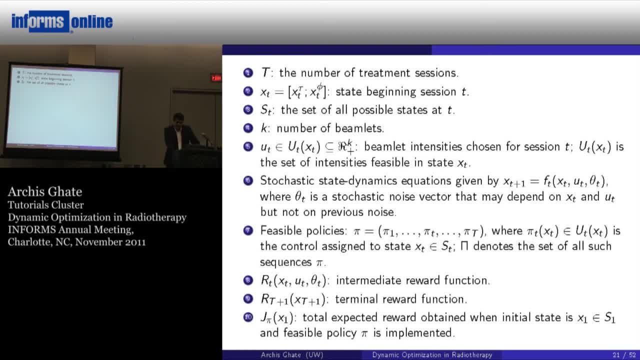 ST is just the set of all possible states. That's not that important. This notation is, by the way, standard for writing stochastic control problems. If you look at Bert Segas' book in 2007, Dynamic Programming and Optimal Control, this is exactly. 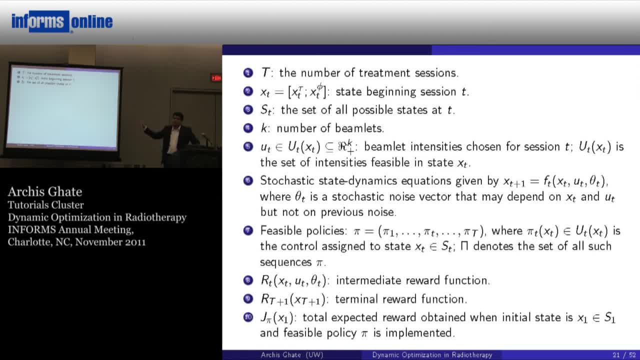 the notation in this book for writing any general stochastic control problem. Okay, So I'm just putting this in the context of radiation therapy by calling this as my tumor state, my OER state, and so on. Okay, So then the K is the same as before. number of beamlets. 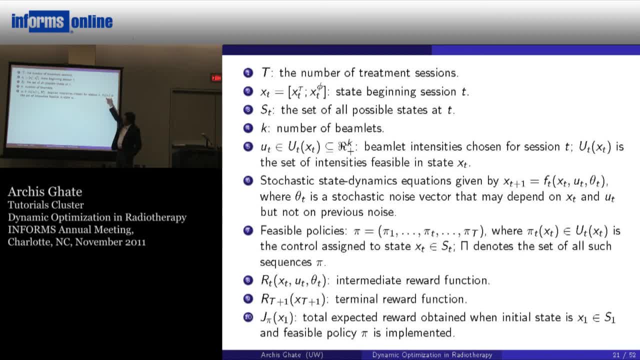 I will use something called UTXT, which is going to be the set of feasible intensities in state XT, And I will show you later on in my models that what is feasible given a particular state depends on that state. Okay, That's why I'm using this notation: UTXT for the set of feasible intensities in state XT. 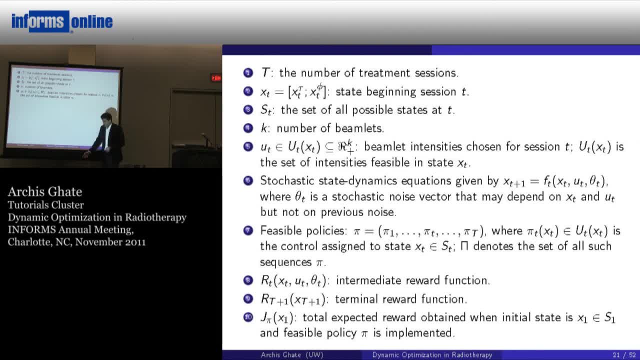 And I will show you later on in my models that what is feasible given a particular state depends on that state. Okay, That's why I'm using this notation, UTXT, for the set of feasible intensities in state XT, And therefore my UT, which is my intensity vector, is going to belong to that. 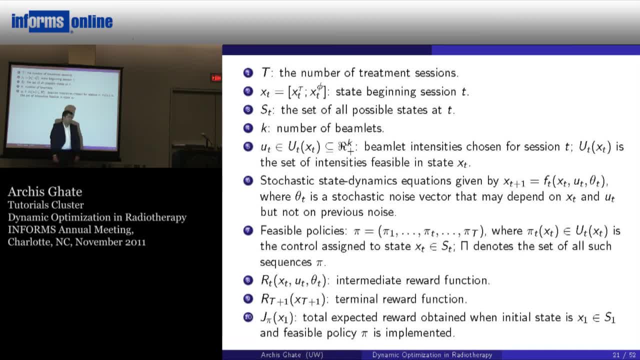 Okay, That's it. So that's going to be my control variables, And then I will need, as you can imagine, some kind of a stochastic state dynamics, Right? So given a state right now and given a treatment, right. 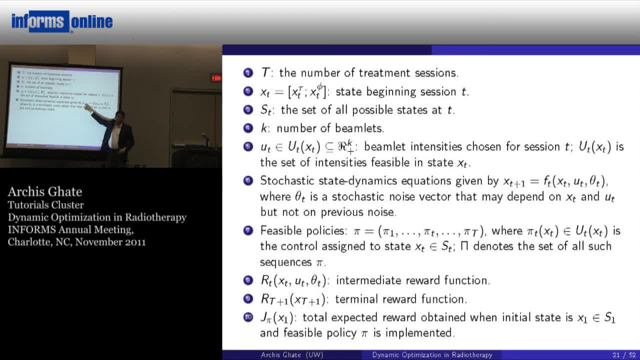 So, given an intensity vector, what will my next state be? So I will need something that tells me that, And then I'm going to have some uncertainty. So I'm going to have some uncertainty, So I'm going to have some uncertainty. 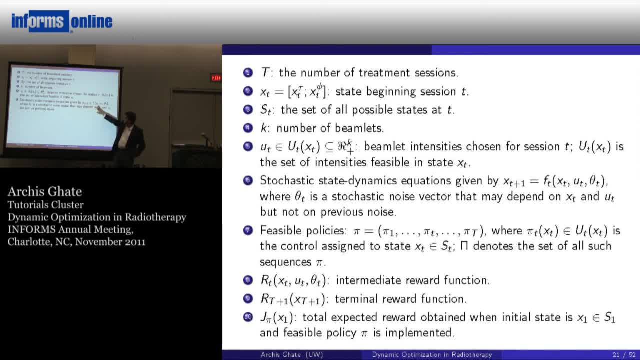 So this is again standard notation in stochastic control in Berserkas's book. This theta is going to be my noise vector or uncertainty vector basically, And the standard assumption in Berserkas's book, for instance, is that this theta t can depend or may depend on x, t and u? t, but not on cold values of the noise. 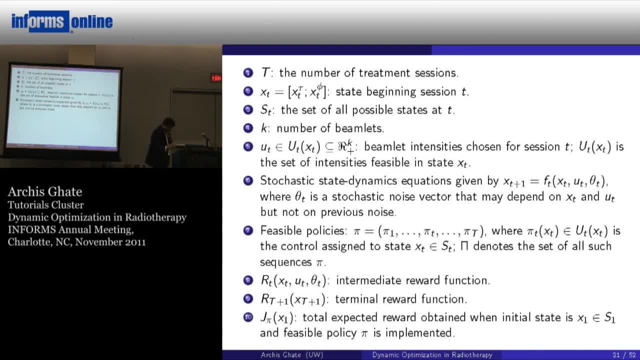 And that gives you basically a nice Markovian formulation. And then I believe most of you are from OR. So, as you know, if you have a stochastic dynamic program or stochastic control problem, you will need to find out optimal policies. So optimal policy meaning it is a mapping from states to decisions. 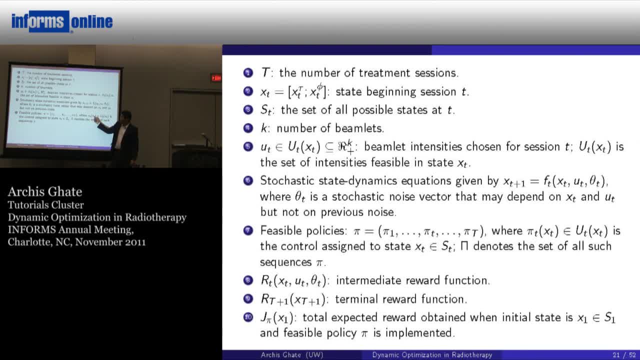 Meaning given a state. let's say x, t, pi t x t will be the decision that I am going to choose in that state. Okay, so that's an optimal policy. So the set of all possible policies will be pi. And then the typical way to think about this in stochastic control- again in Berserkas's book- is to have some kind of an intermediate reward function. 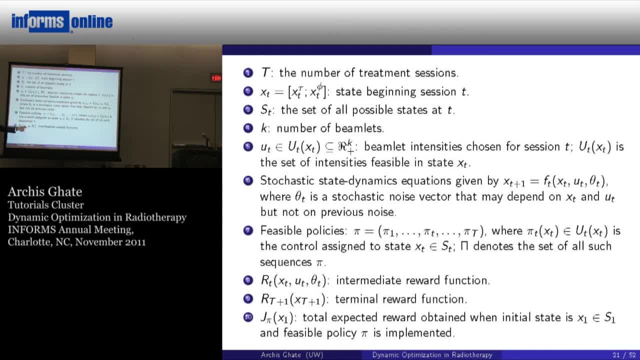 Meaning that if I choose intensity u in state x, t and if the noise is theta t, then this is the reward that I will collect in that period, Right in the stochastic control or stochastic BP language, But in this case in that treatment session. 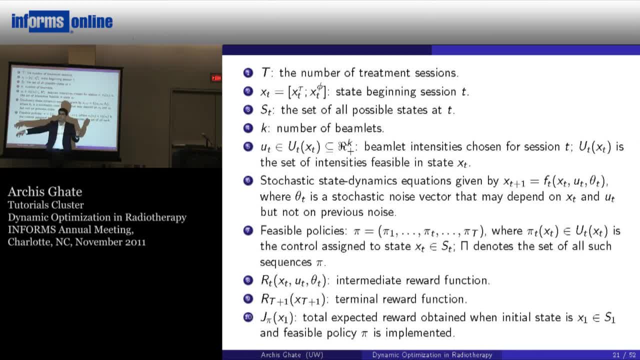 And when this whole thing is over, I am going to collect a terminal reward, Right? so when the treatment sessions are done, so treatment course is done, I will collect a terminal reward And that's going to be notation for that. Okay. 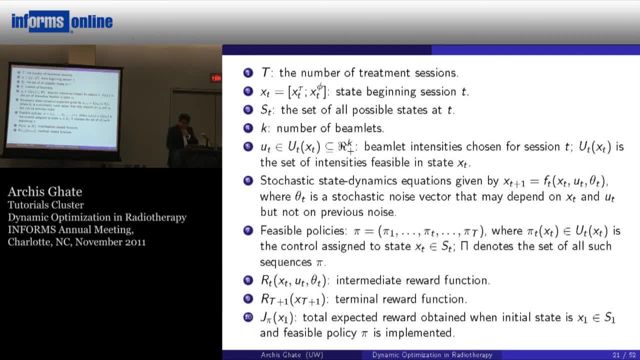 So is the notation at least roughly cleared or at a high level. Okay, so this is very abstract, Right? I have not told you anything about what these things are. This will become more concrete as we go, But I will need one more piece of notation. 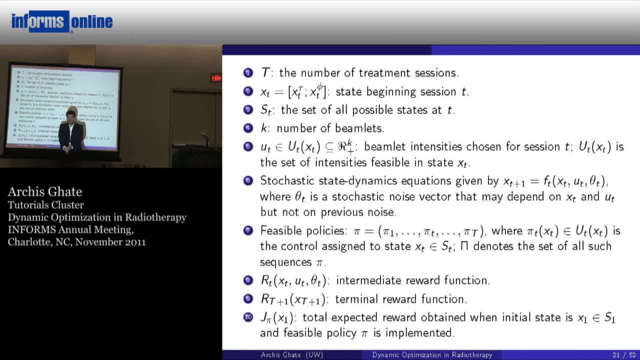 So if I start out in state x1,, so at the beginning of the first treatment session, if the state or the condition of the patient is x1. And if I choose to implement policy pi okay throughout my treatment course, what does that mean? 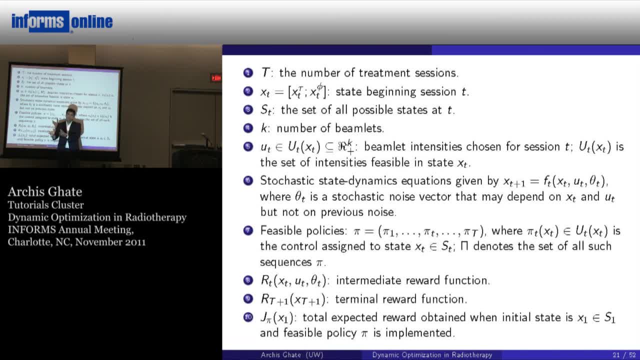 Policy pi will tell me what to do if I find my patient to be any particular state in any treatment session. Okay, so if I choose to use that policy pi, This j pi of x1 is going to be the total x1.. This is the expected reward that I will get over this treatment course. 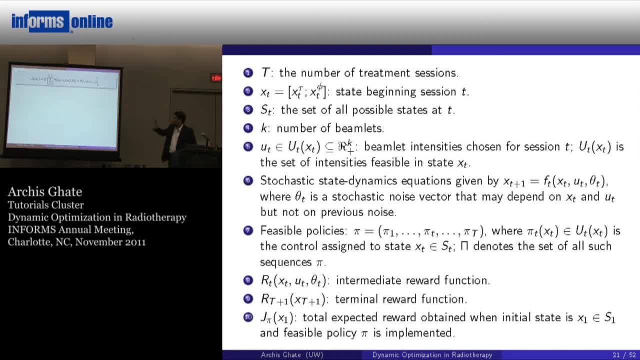 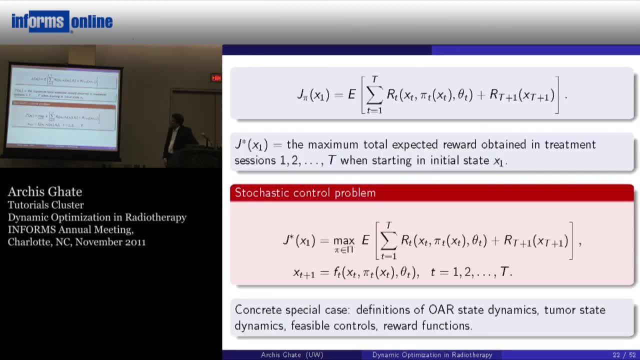 Okay, so that's my notation. And then, using this notation, you know this is the standard stochastic control formulation that you can write, So let me just quickly show you that. So j pi x1,, as you can see, is basically the expected reward over the entire treatment course. 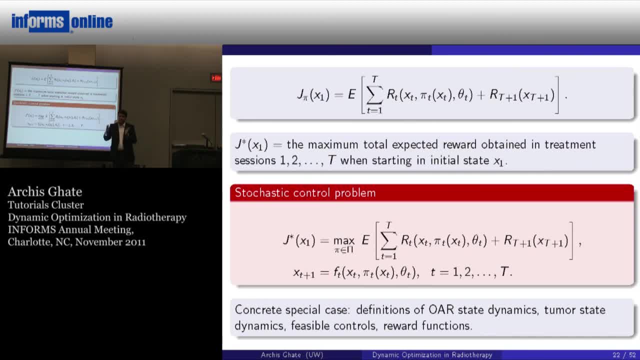 So all I'm doing there is I'm adding the reward that I collect over all treatment sessions Right, the intermediate rewards, So t equal to 1 to capital T, And then I'm adding the terminal reward right on top of that. 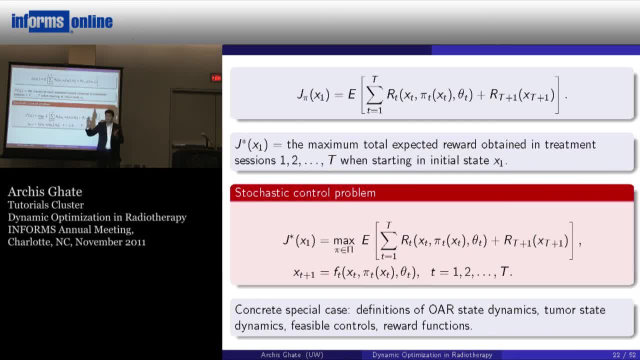 The expectation: right, so this state. right, so the state evolves stochastically. Right, so the expectation is with respect to how that state is going to evolve. basically Okay, so that's j pi, x1.. And what I want to figure out is basically the largest reward I can get, given that I'm starting in x1.. 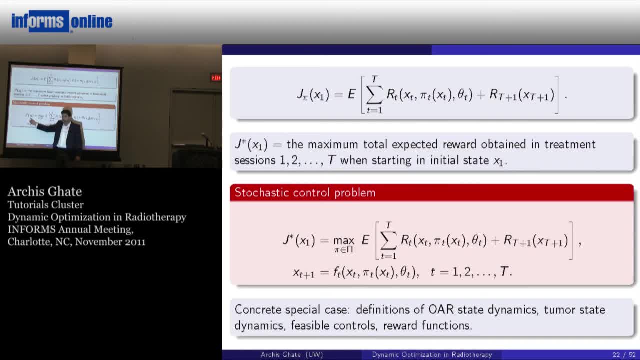 And the notation for that is j star of x1.. So that's the largest reward I can get, And that is simply the largest of this objective, which is that expected value. Right, it is the largest among all j pi x1s. 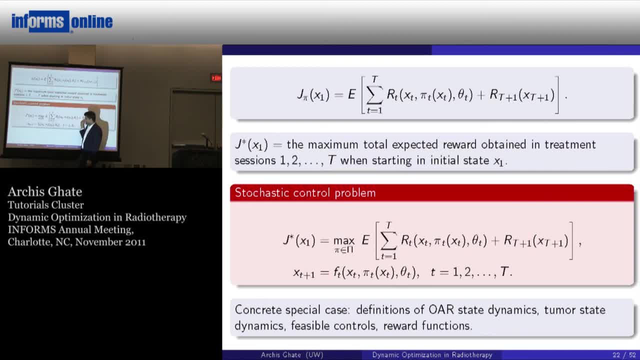 Right, so I want to find a policy that maximizes that subject to this dynamics. Okay, because this is how my state is going to evolve. So this is, of course, very abstract. You know, this is not even talking about radiation therapy, really. 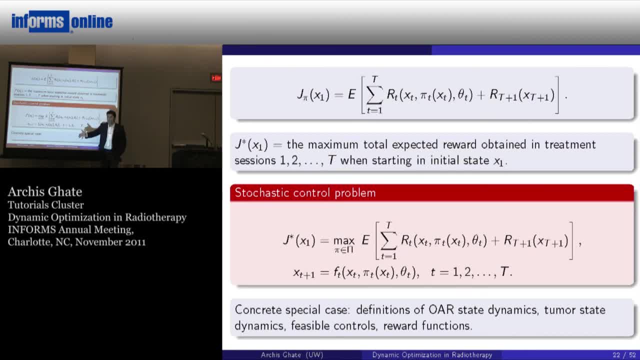 This is literally copying almost what Burtzikas had done. It's copying almost what Burtzikas has in his book right on this slide. But I need to give you a concrete special case of radiation therapy. And what I mean by concrete special case is I need to at least for us to write down the model. 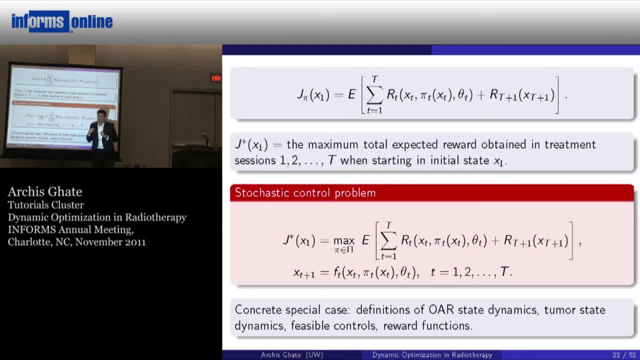 I need to give you what my states are for the OAR and the tumor. I need to explain what the set UTXT that I showed you, so what the set of feasible decisions is, And I need to talk about reward functions. So if I give you concrete examples or special cases of these, 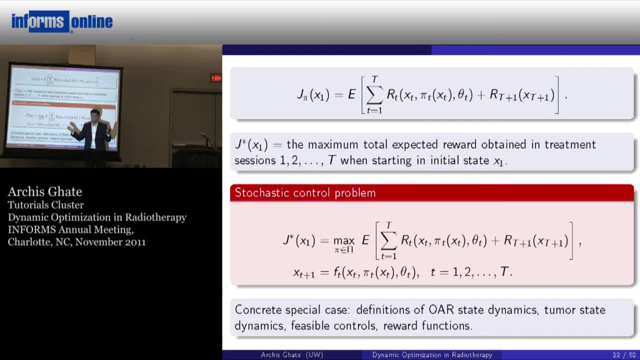 then that will be our stochastic control formulation of this radiation therapy problem. Okay, so the next 25 minutes roughly. I'm going to give you a special case for each of these. So I'm going to start with OAR dynamics. Okay, and by no means am I saying that this is the only way to do it, right. 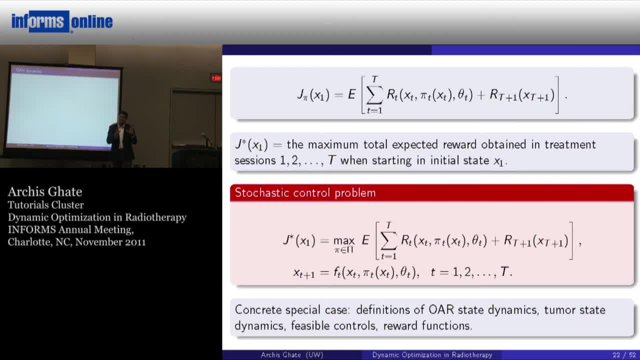 As you can see, my general stochastic control formulation and that's in our paper. it is extremely general. I have not said anything about what those things are, So, for example, your hypoxia that you talked about last night can be a special case of that. 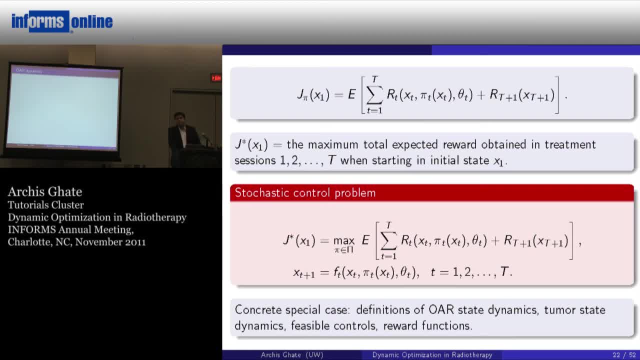 and we talked about that in the paper as well, But today I'm going to give you one way of doing it. Okay, my hope is that once people start reading the paper, hopefully people will come up with different ways of modeling this and perhaps there will be special cases or variations of that high-level stochastic control formulation. 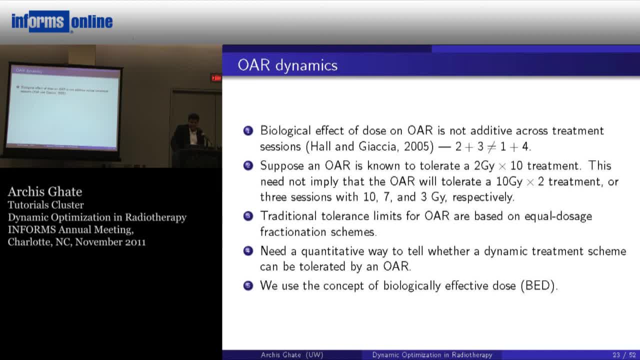 Okay, So let's start one by one. So OAR dynamics. So the difficulty in coming up with OAR dynamics is the following: So suppose I give some dose to my OAR, So the OAR receives some dose. The effect of that dose on the OAR is not additive over treatment sessions. 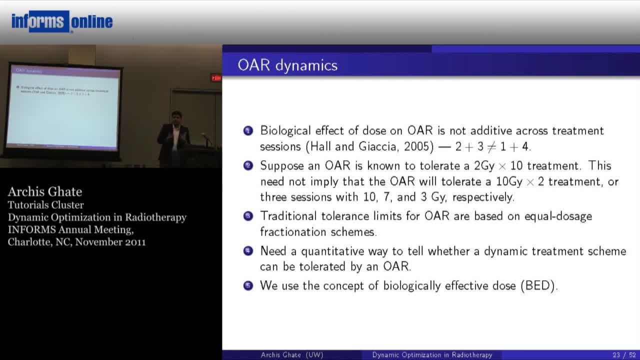 Okay, and that's in that book. What does that mean? That means 2 plus 3 is not equal to 1 plus 4.. Okay, so what does that mean? That means, simply speaking, that if I give a dose of 2 in the first treatment session, 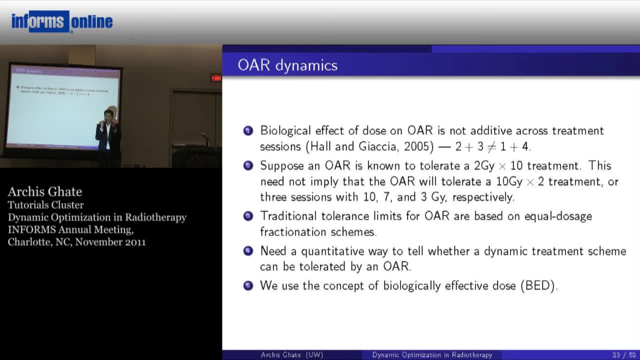 and dose of 3 in the second treatment session to my OAR. the damage that these two doses do to my OAR is not the same as the damage 1 and 4 will do to my OAR. Okay, And as you can imagine, that comes from the fact that 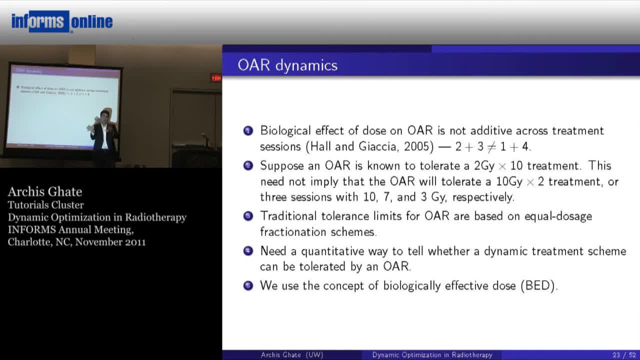 remember, a while ago I showed you that curve. that is a non-linear curve, right? So the doses are not quite additive on that curve. basically That's the basic reason for that, In other words, typically so. the difficulty is that you know. 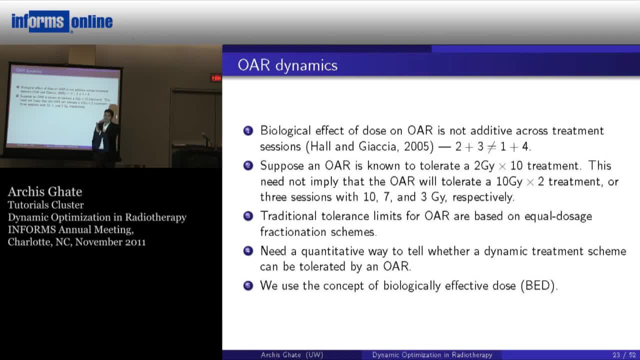 the conventional way of treating, as I said, typically, is equal dose fractions, right. So I have been using this: 2 grade per fraction for 10 fractions, or 1.5 grade per fraction for 15 fractions. Okay, So that is not the same as, let us say, 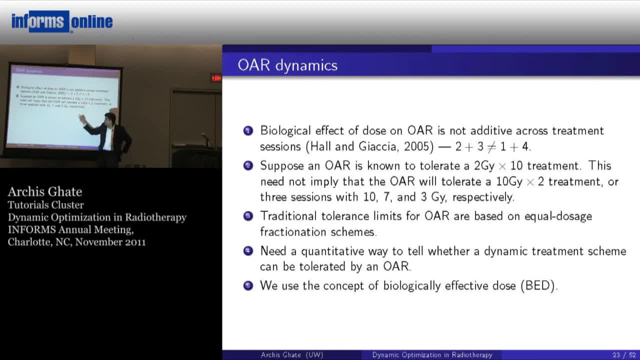 10 grade in 2 fractions right, Or it is not the same as 10,, 7,, 3, right, That is up to 20, but the effect is not the same right, And this creates a difficulty, as you can imagine. 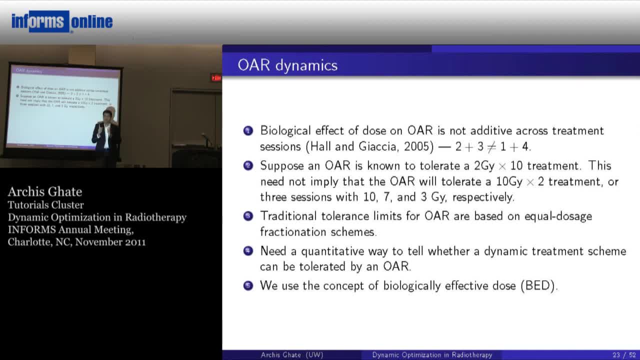 because I am not fixing my doses beforehand, right? So I do not know at the beginning how much dose I will give in the first treatment session, I do not know how much dose I will give in the second treatment session, and so on, right? 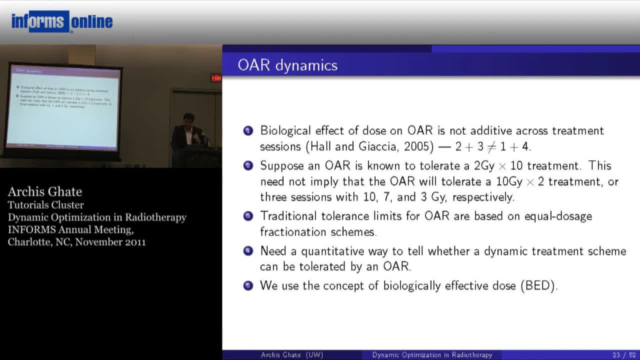 So this is completely, in fact, stochastic and non-stationary, so changes over time. So that's why initially we thought it was kind of difficult to actually come up with appropriate OAR dynamics and what the stage should be and so on. 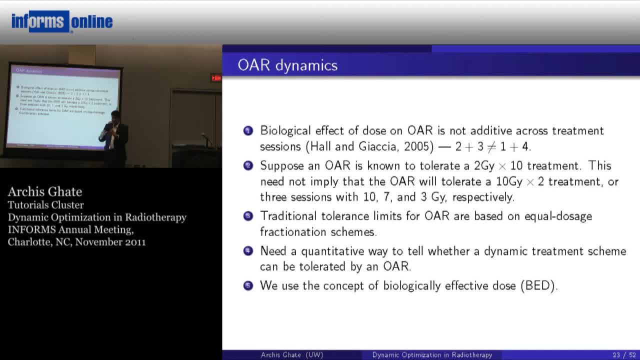 The other complication is that when somebody says that this particular organ at risk, so let us say the spinal cord, can tolerate 45 grade of dose, okay, Typically I believe they have some kind of a fractionation scheme in their mind, meaning so, for example, 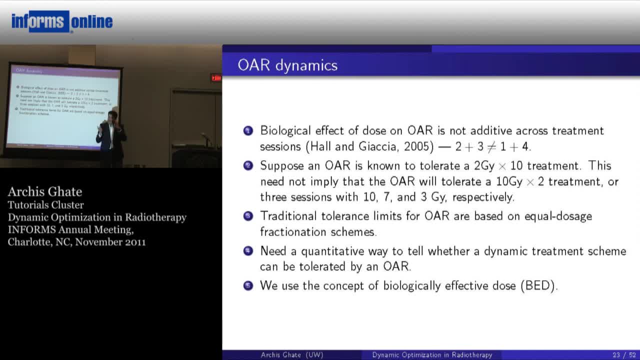 let's take an even number. so let's take 44,. right, They have something in their mind which says that it can tolerate 44 if given In 22 fractions of 2 grade each. right, They don't say it, but I think it is implicit, okay? 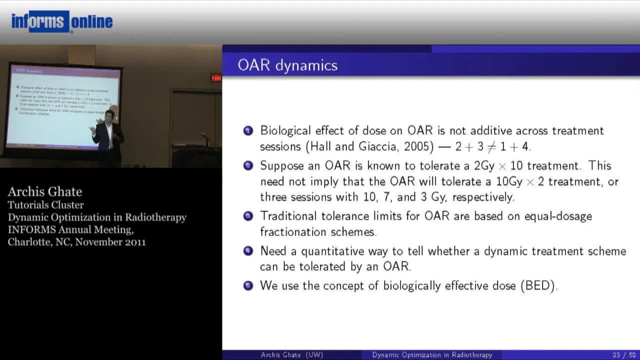 Another example: when they say it can tolerate 20, they mean if given in 2 grade per fraction, 10 times okay. So we cannot really directly use that number. 44, right, Because I'm not going to give the same dose in every fraction. 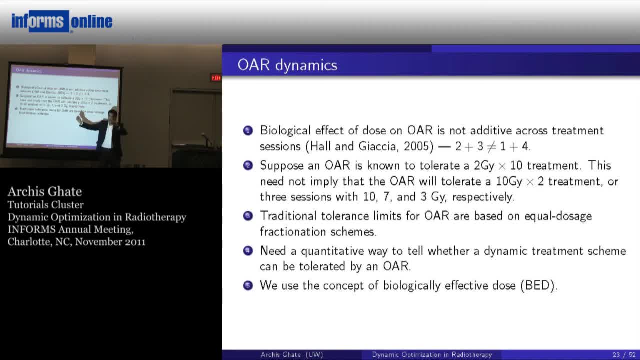 In fact I don't know what I'm going to do. It might be completely all over the place right, Changing non-stationary over time. So that was another difficulty, So we could not use those kinds of numbers directly, okay. 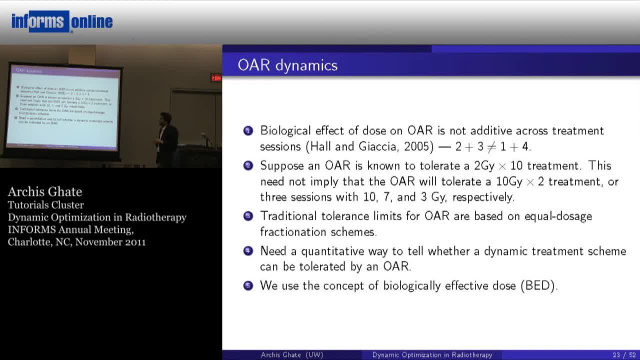 So we wanted to come up with or use a quantitative way to tell whether a dynamic treatment scheme can, in fact, be tolerated by an OER. okay, So that was the challenge, And I believe there might be different ways of doing it. In fact, I think you talked about one related issue in your talk yesterday. 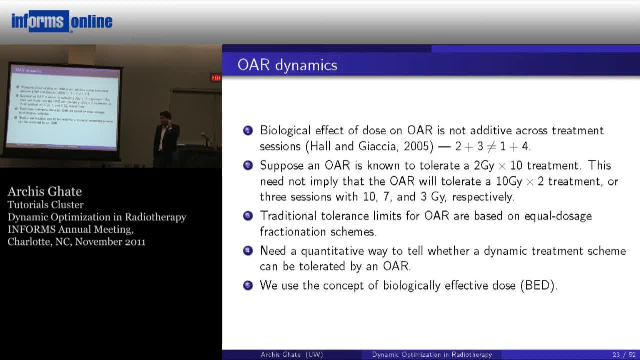 and I asked you a question at that time. okay, So that might be one way of doing it. We are doing it in a slightly different way, So we can talk about that later on again, But I'm going to show you one way of doing this. 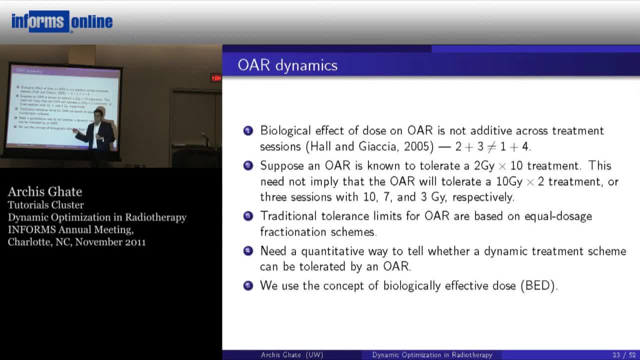 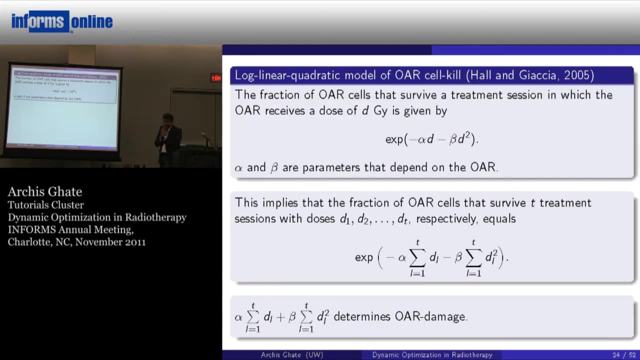 And we actually used something called biologically effective dose for doing this, And this biologically effective dose idea is in that bible on radiobiology, if you want to refer to that later, But the idea is pretty simple. So I'm going to actually, in 2 to 3 minutes, quickly derive things that relate to biologically effective dose. 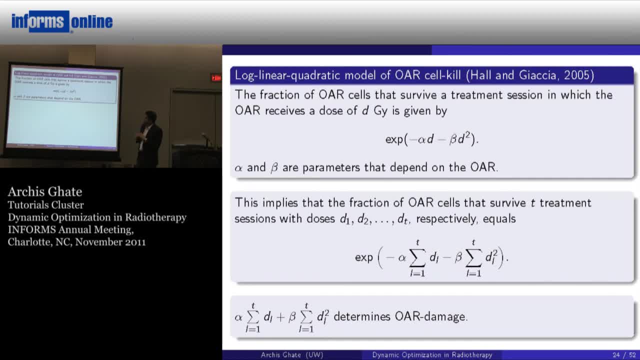 So I'm going to start at the well-known log linear quadratic model of OER cell kill. It's from that book And basically it says that the fraction of OER cells that survive one treatment session with dose T is that okay? So it's log linear quadratic because if I take the log of this I get a linear quadratic function okay. 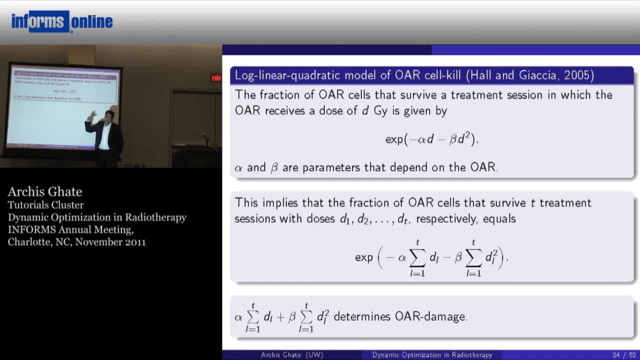 Where alpha and beta are parameters that depend on OER. So spinal cord will have different alpha betas found empirically, let us say, right- As compared to some other normal tissue organ at risk, and so on. okay, So this is actually what I was trying to show you a while ago in that non-linear curve that I showed you. 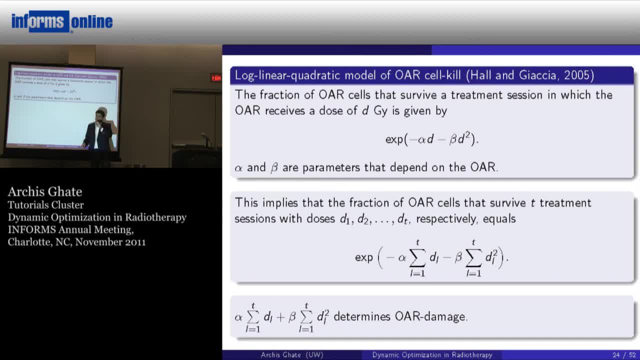 Basically, it was this fractional cell survivor curve that I was trying to show you. okay, So from that, using the property of the exponential function, that if you multiply exponential functions you can add the exponents, right. So this is the property I'm using here. 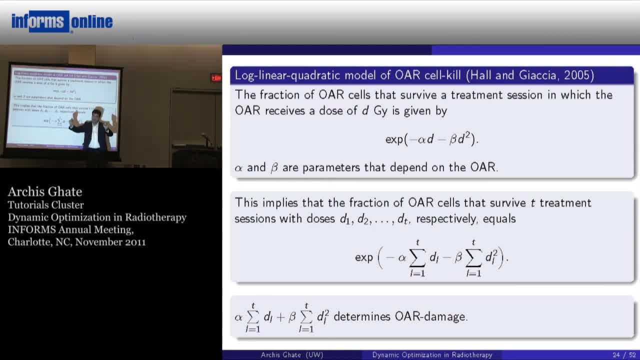 So if I actually give d1,, d2,, d3,, dot, dot, dot up to dt, okay, The fraction that will survive will actually be a product of exponential functions, with d1,, d2, and so on. right, 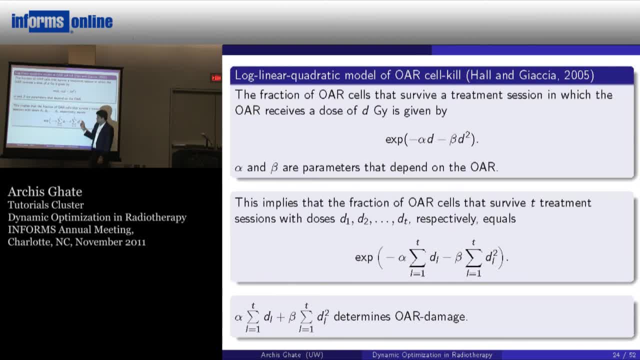 Like that in the exponent And I multiply the whole thing, I will actually get sums Make sense. So exponential A times exponential B is exponential A plus B. That's what I'm using to come here. Yeah, Oh, I guess it's this exclusively. 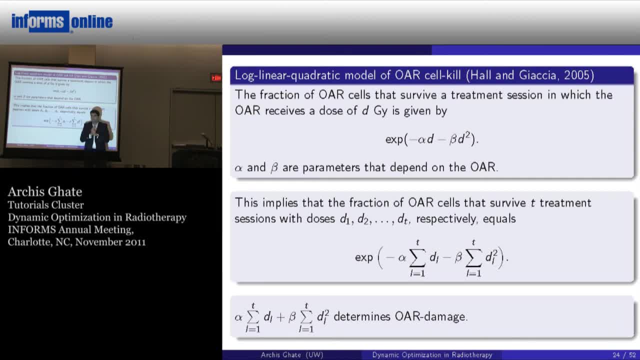 You're assuming that separated is sufficiently time. Yes, Okay, So that is assumed in the sense that 8 to 12 hour separations that I mentioned? Yeah, So that I think that's just algebra. So if you look at this, you know this term lies in that exponent. 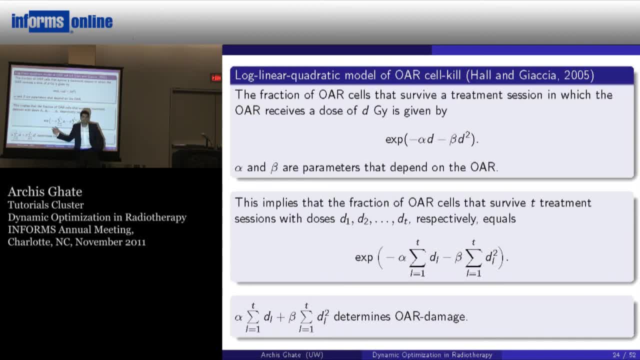 But basically this expression is what decides how much damage will be done to my OAR, essentially according to this model. Okay, So if you just stare at this, the units of this are actually not in dose. Okay, Because this is in the exponent. 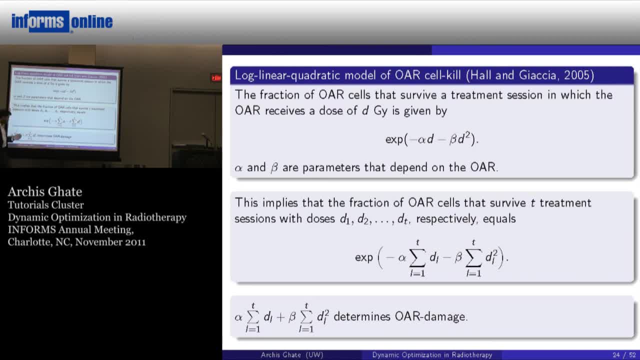 So this is a unitless quantity, Right? So this is actually unitless. The unit of alpha is dose inverse, So gray inverse. So I'm going to just convert this to units of dose by dividing the whole thing by alpha. Okay, 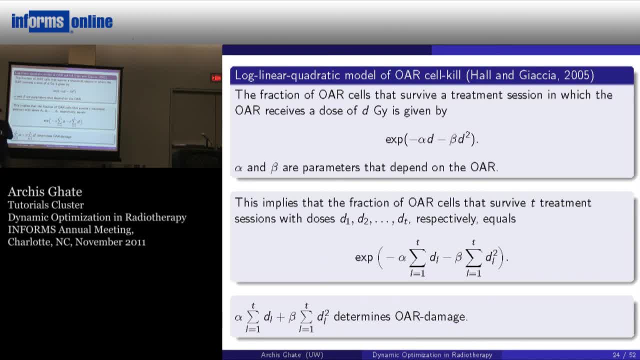 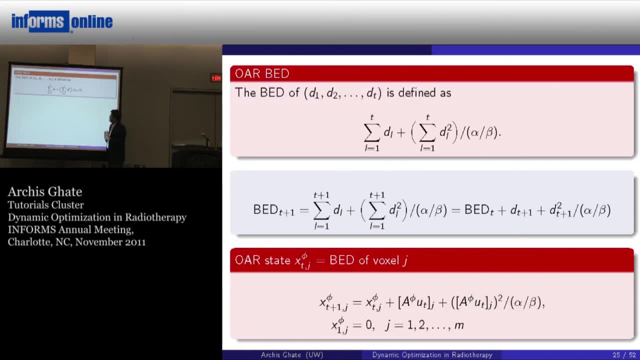 And that gives me biologically effective dose. Okay, And that's the definition basically on my second slide. So the biologically effective dose of d1,, d2,, dot, dot, dot, dt is simply that term that I showed you, divided by alpha. 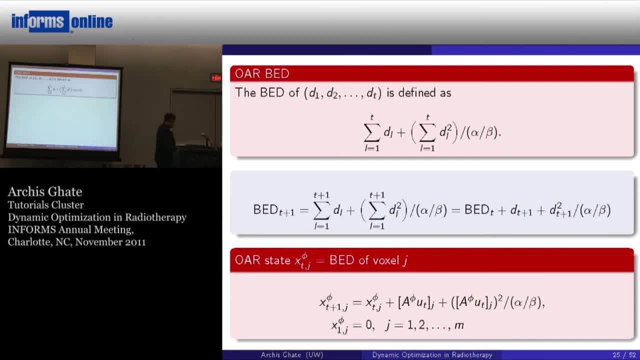 Okay, And I got that alpha or beta in the denominator because that alpha vanished divided by alpha, and I then moved that to the denominator. Okay, So that's how I get this PED expression And that's the definition of PED. Okay, 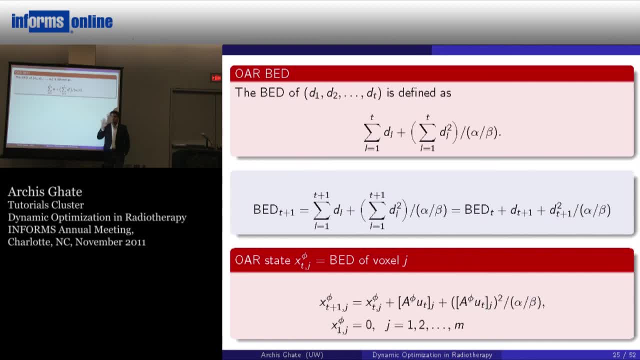 The funny thing is that, if I'm not wrong, this derivation is not in the book. I might be wrong, I don't remember, But there are other ways of thinking about this perhaps, But this derivation is in my tutorial, Okay. 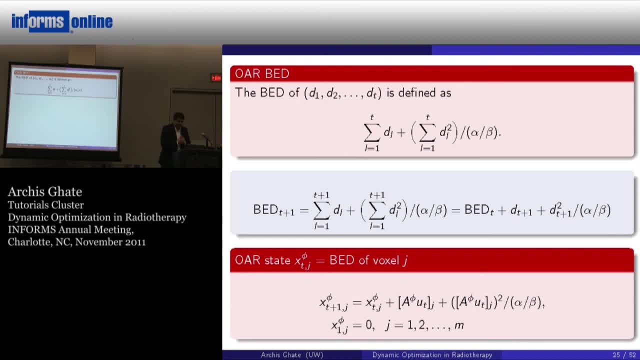 So this is how I think of biologically effective dose. I'm not sure this is the exact derivation, but the formula is the same. Okay, In the book as well. The beautiful thing about this is that now I can actually kind of start thinking about using this as my state for my OER, because that relates to, as I said, the damage that I have done to my OER by giving this sequence of d1, d2, dt, up to dt. 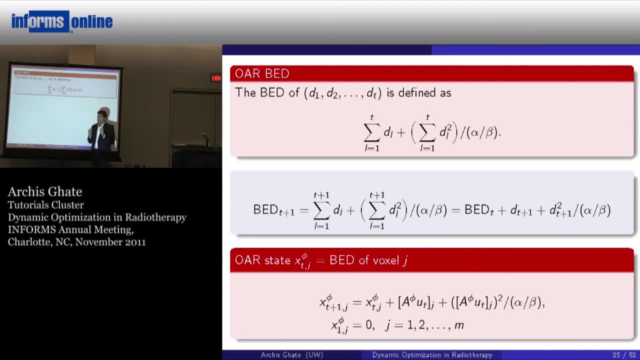 Right, And they don't have to be constant or anything like that. That's one. If you stare at this, you will see that this will actually give you a very simple state update formula for the state Right. And that's my next slide. 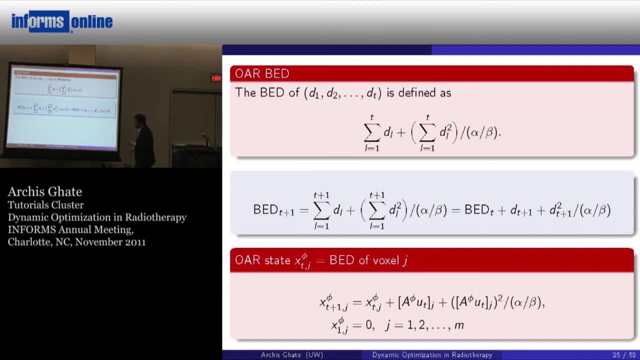 And that's also a beauty of this, I think. So we were very happy when we just kind of discovered this. you know the fact that, okay, this gives me a very simple PED update formula, meaning that if I give a sequence from d1 to dt plus 1, then using that formula, I have this: 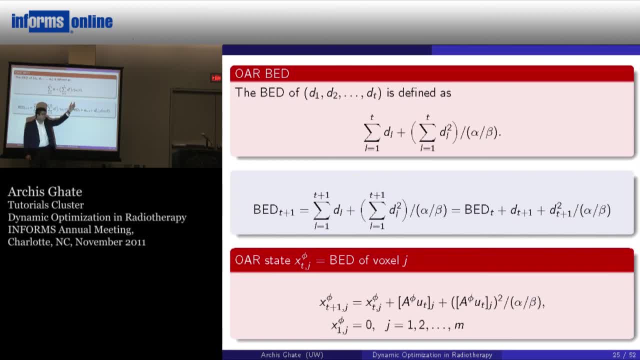 Right, And because this is all just additive stuff, right, I separate the terms and I get PED up to t plus the additional damage that I do in that session Make sense. So that's the beauty of this. So I'm actually going to use this as the state for my OER and, going back to that x notation for the state, 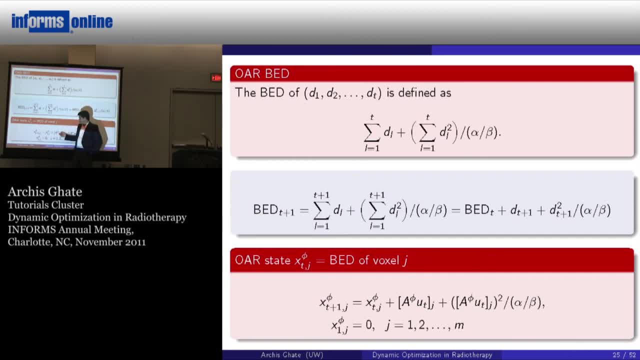 So all I need to do is now I have an equation that tells me how my OER state is going to evolve. This is my PED. This is my PED after t, which is here. This is my next PED, And I simply need to add a dose term plus a scaled squared dose term. 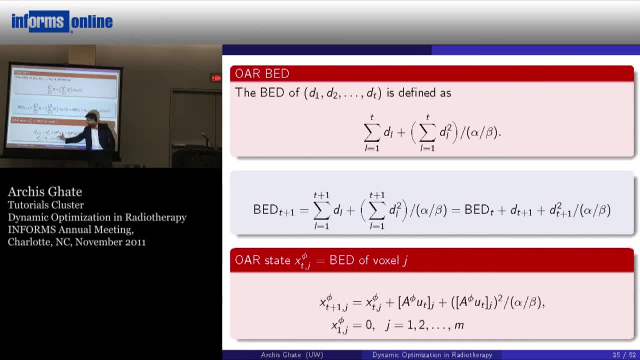 Right And, as you remember, this is the dose that is given to the jth voxel of the OER, Right In our notation, And this is the square of that, divided by alpha over beta Right. So I now have a simple state update formula for my OER in terms of my current state. 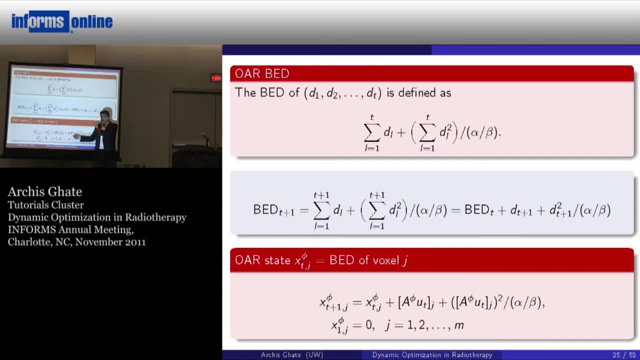 And the intensity vector that I choose in that treatment session. Right, That's what I need and that's what I have now. One more last piece: Initial PED is zero, assuming that I have not given any treatment before that, So that PED is just zero. 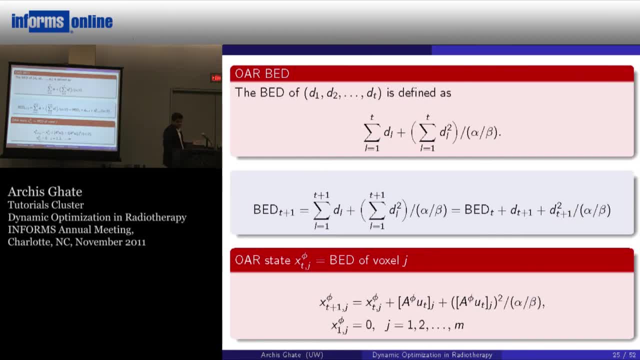 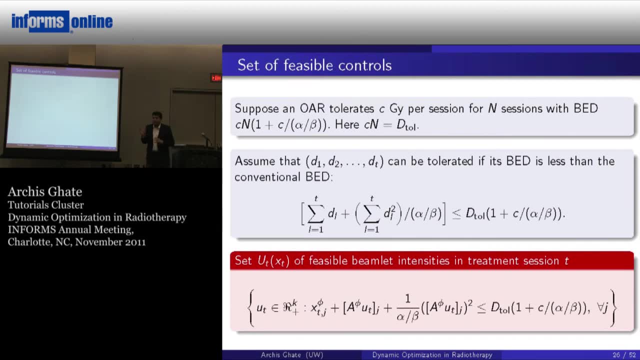 That's fine, Or any other number, It doesn't matter, Just I need some initial condition. So now I have OER dynamics. That also gives me another very elegant thing which I like, And that is it actually is going to give me the set of physical conditions. 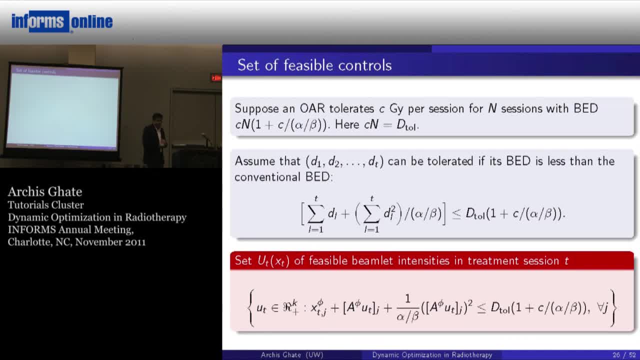 Right, The set of physical controls. Okay, So what we did is that? remember I had mentioned that this difficult to a difficult meaning. it's not obvious how to compare two different schemes, Right? So two gray per fraction ten times, Is that the same as three one four five. two, three, one four five. 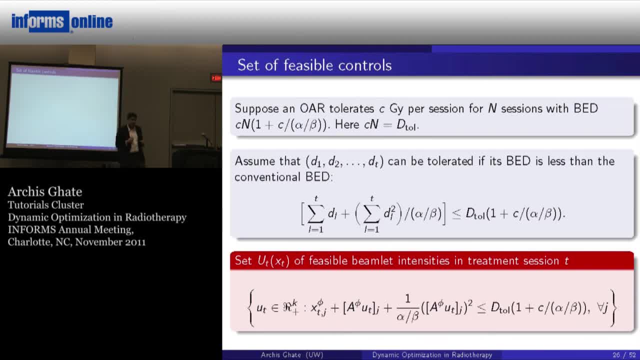 Or something like that. If I want to compare two crazy things like that, how do I compare And how do I say whether this thing is even feasible, whether the OER can tolerate this crazy thing? Right, And the idea is that here, so I'm going to assume that some sequence- D1 to D2 P can actually 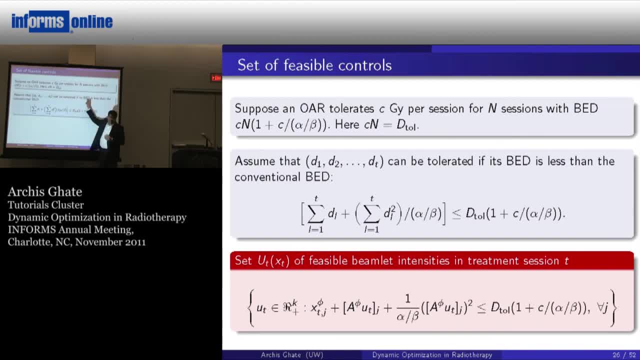 be tolerated if it's PED is less than the conventional PED. Okay, So let's go to conventional PED. So conventional, remember constant. So C grade per fraction for n sessions. Suppose that is the constant per session And that is known. It is known that OER can tolerate that. 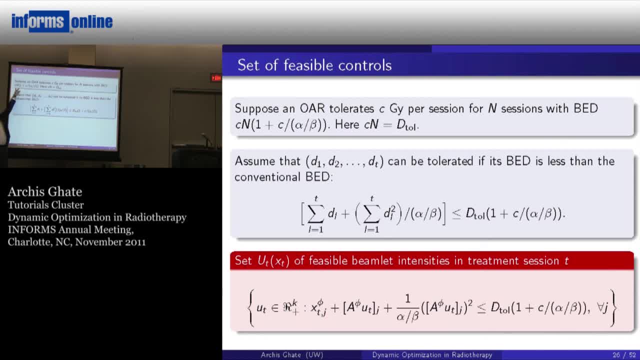 So I simply compute its PED. And the PED is simply, you know, the sum of the doses. So I'm giving C n times, So that's the sum, And then C squared n times divided by alpha over beta. So this is the PED of the conventional treatment fractionation scheme, which the OER is known. 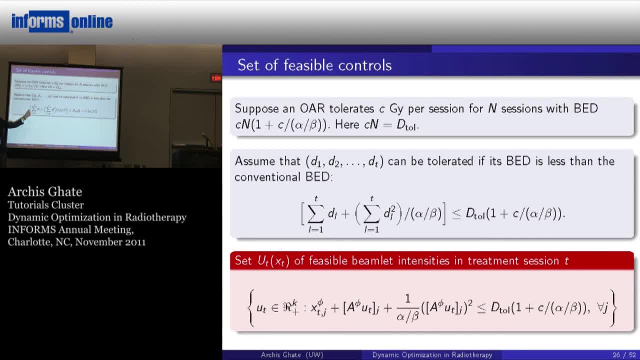 to tolerate. And what I am saying here is that some other sequence- D1 through DT- will be tolerated if its PED is less than what the OER is known to tolerate. And why is that an appropriate assumption? Because the PED essentially characterizes damage to the OER. 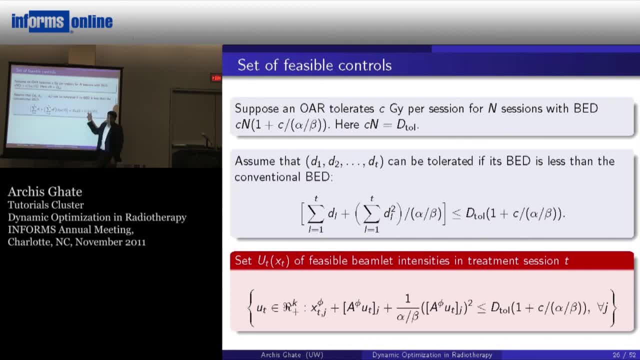 Right. So if this damage was okay, then this must also be okay, because the damage is, in fact, less Okay. That's the idea And, as you can see, this will give me the set of feasible controls. Why? Because I have my PED in terms of my U. 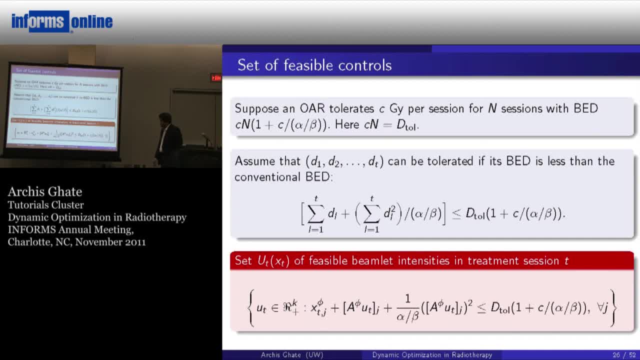 Right. So that's my next slide. So, given that I am in state XT Right, As I said in the previous slide, this is my PED Right, New PED, And then that has to be less than this And that gives me the set of feasible use. 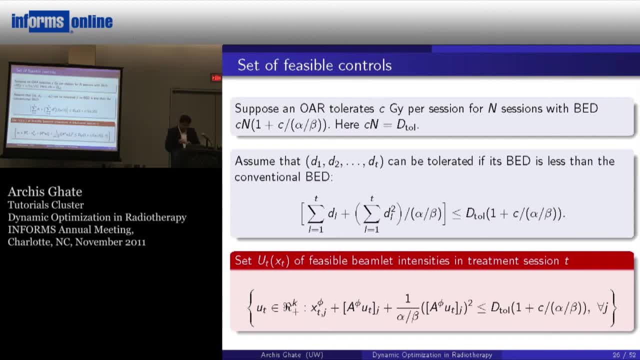 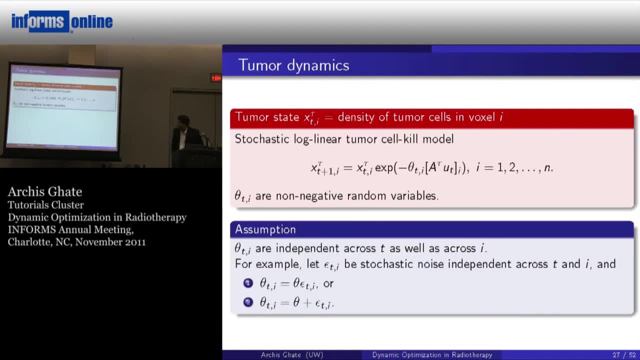 Right. So this way of modeling not only gives me my OER dynamics, but also gives me the set of feasible use. So let me speed up a little bit. So the next part is tumor dynamics. So what we did was tumor dynamics. We also used a similar model. 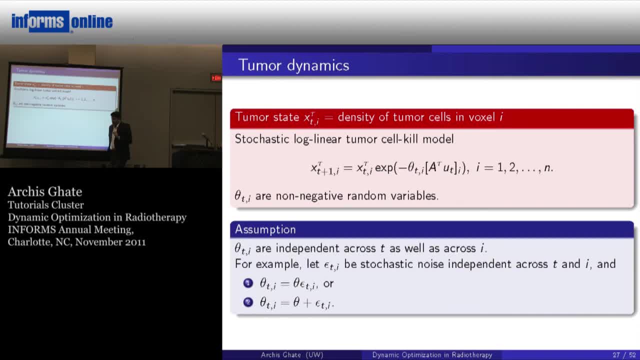 The only difference was that. so there are papers out there which says that the alpha over beta ratio for tumors is different from typically the alpha over beta ratio for the OERs, In fact. so the alpha over beta ratio is high for these tumors. 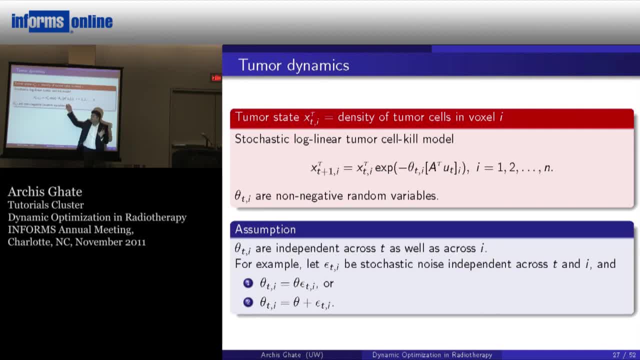 So I am actually ignoring the quadratic term here. You don't have to do that, We don't have to do that. In fact, we have follow on models where we actually did not do that. There are a lot of different models. There are a lot of different ways in which you can model uncertainty in tumor response.